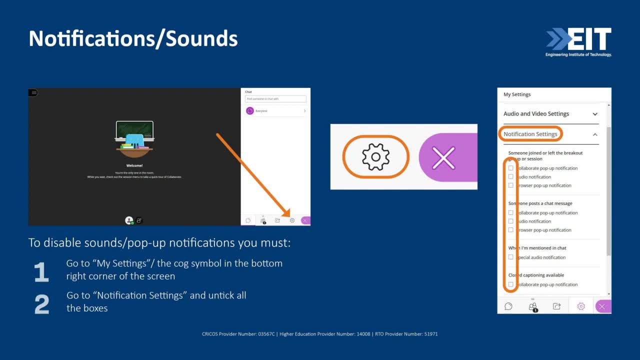 Alright, I can see people giving me the time. I'm gonna go ahead and start the notification settings. Alright, I can see people giving me the time and I'm going to press any of those buttons- the thumbs up- for the notifications part. so if you have questions about how to do it, you can. 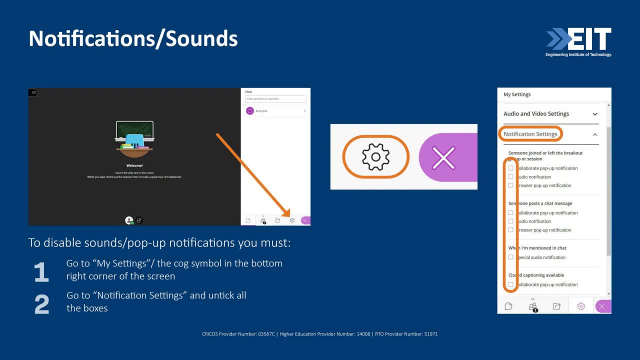 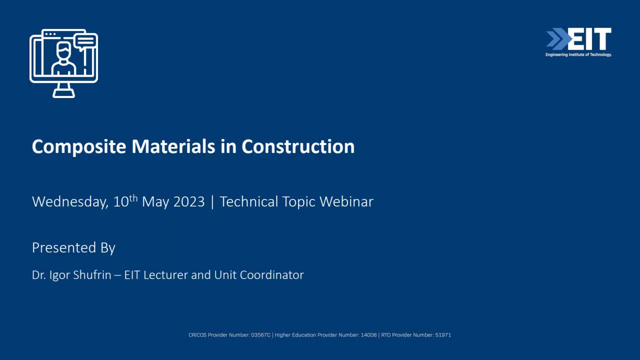 just post it in the chat. i'll go ahead and give you the instructions again later on. all right, so for today's session, our topic would be about composite materials in construction, and this is going to be presented by dr igor shafrin, and he is one of our lecturers and unit. 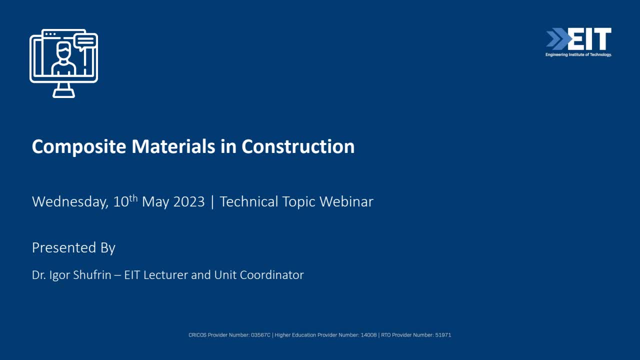 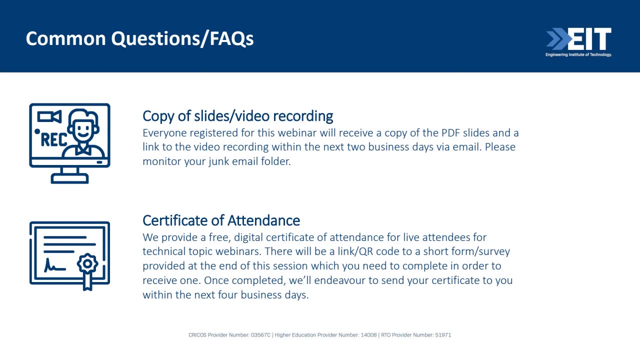 coordinators at eit and later on he will be introducing himself as well. so about the copy of the slides that are going to present today and the video recording of the webinar? we will be giving a copy and of the video recording to to everyone and that is after the webinar session. most likely we will be um. 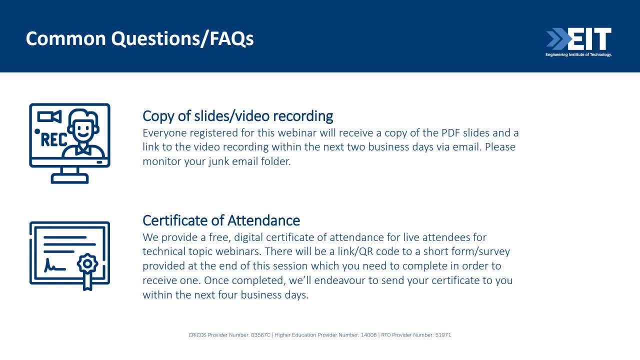 having that available in the next two to four working days and the certificate of attendance as well. please note that you should use the qr code or the link that I will be posting later on to register and request for your um certificate of attendance and again, it will be available or will be sent to your email in two to four business days as well. so just a little bit of background about electric projects in the ects business days this evening. it's hard to make sure that all of you can find my slides very quickly. i mention them that way soon as needed. y'all definitely can find my slides. there's a lot of stuff down there. a little bit more about 1- порядiner, which i will show crochet seminary ops and how to use it in this session if you'd like to check out. thank you again for your insight and i will see you at the end of the session. so until then, thanks again to you all for having me and i will see you all next week. bye, so just a little bit of background about integral a ölian. so all of us talked about re-enabling. 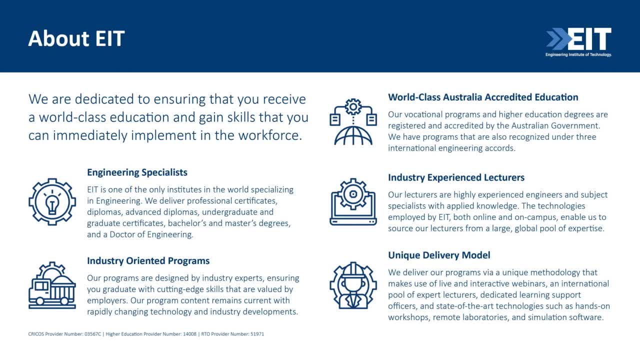 EIT. So we are an engineering school and we are based in Perth, Western Australia, And we are also one of the very few engineering specialists institute in the whole world And we deliver a lot of courses, ranging from professional certificates to diplomas advanced. 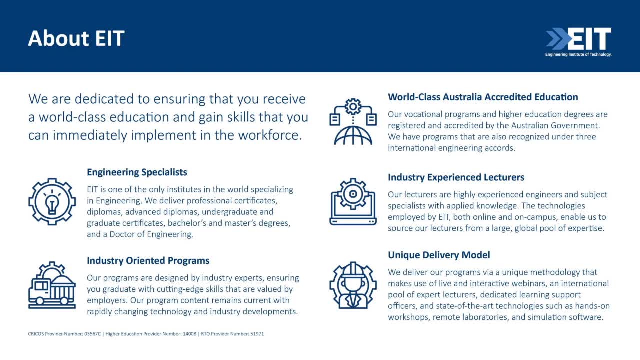 diplomas, undergraduate and graduate certificates, higher education courses like bachelor's and master's degree courses, and even a doctor of engineering course. And the good thing about EIT, or what makes EIT unique, is that we are industry oriented. Our programs are. 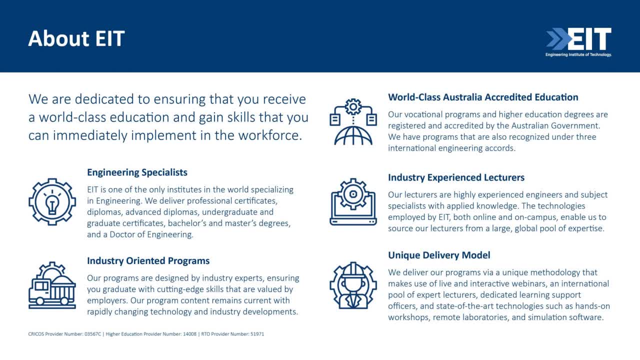 designed by industry experts, just like our presenter today, Dr Eager, And we are ensuring that our graduates would have cutting edge skills and these skills will be valued in the workforce. And, of course, we also make sure that our school and our 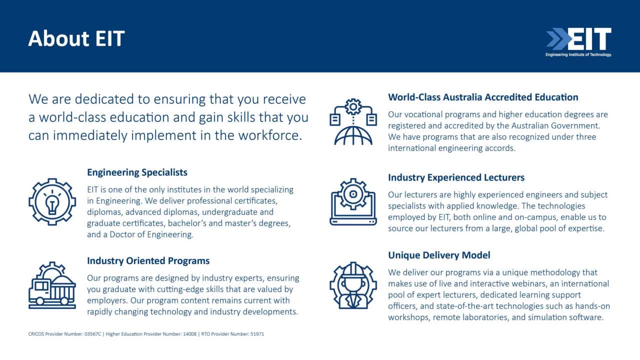 facilities would be up to date with the rapid technologies in the industry And we also have world class Australia accreditation. So we have international accreditation and we also have accreditation from Engineers Australia in some of our courses And that would be in the Sydney Accord, the Dublin Accord and the Washington Accord as well, And for our other 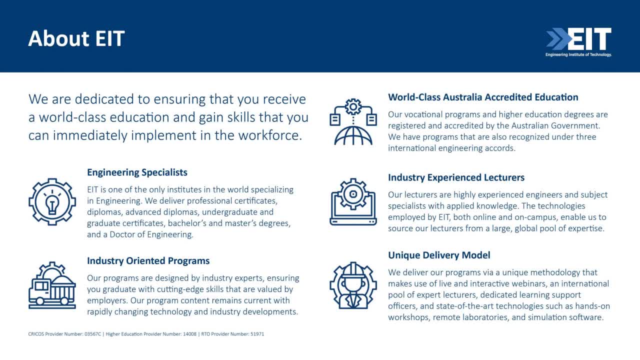 courses they are. they are all accredited by the Australian government And, of course, we are proud to have industry experienced lecturers, just like what we are having today, because we would like to have our students would be exposed to the up to date or the latest trends in engineering or in the 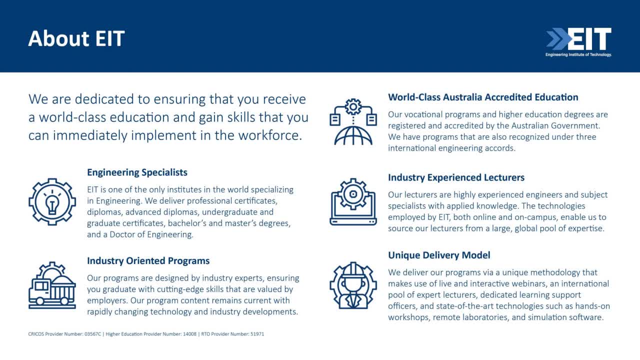 industry And, of course, these lecturers would be able to give practical, updated insights about our engineering courses. And we also have a unique delivery model. we have a unique methodology And that is through our interactive webinars. we also have live lectures for our on campus programs And we also assign a 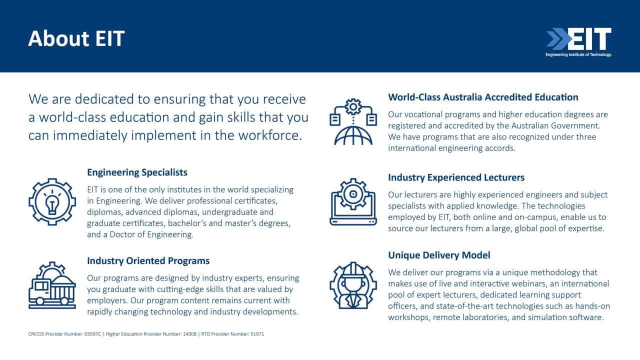 dedicated learning support officer for each course so that our students would be supported all throughout the course. And we also have state of the art technologies, such as our hands, hands on workshops and also our virtual laboratories and our remote labs. So those are our simulation softwares, So our practical activities for students. 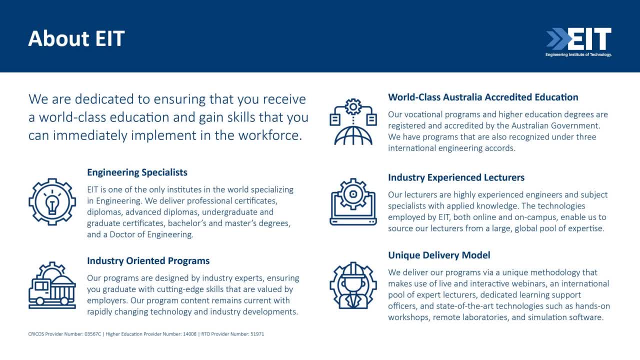 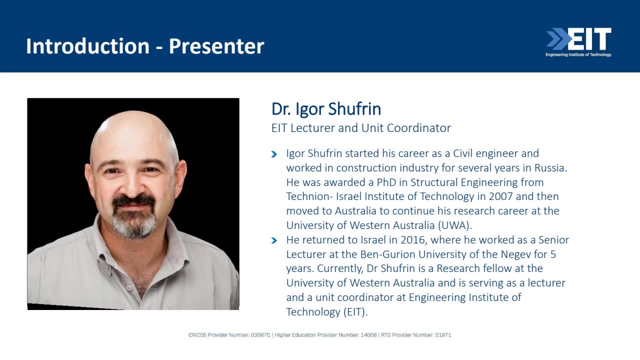 are really close to reality. And that's it about EIT. Now I'd like to introduce Dr Igor Szafrin Again. he is one of our lecturers and unit coordinator at EIT, and I give him the liberty to be碼. 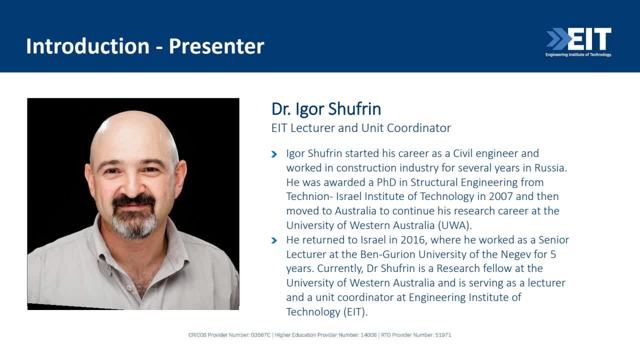 to tell more about himself now. Thank you so much, Dr Eger. Hi, Lisa, Thanks, Lisa, Can you hear me? Yes, we can hear you. well, Right? Thanks, Lisa, for introduction. So I think the stage is mine now. 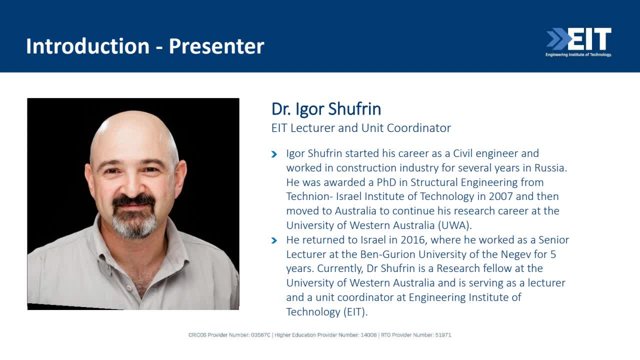 Yes, that is correct. So you can tell our participants something about yourself, or yeah, and you can go on with your presentation. All right, well, thank you very much, Lisa. Yeah, about myself: I am a big fan of hybrid structures and materials. 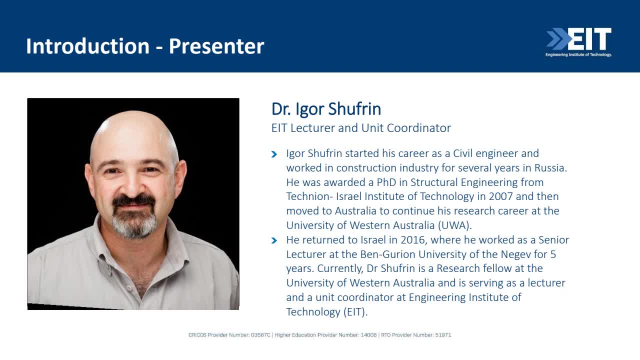 Been- and there's a researcher in the lecture for the last 20 years, So I've got quite an experience. My research topics involves the composite materials, computational modeling, composite structures- mainly for civil engineering, but not only. There are some projects involving the drilling projects. 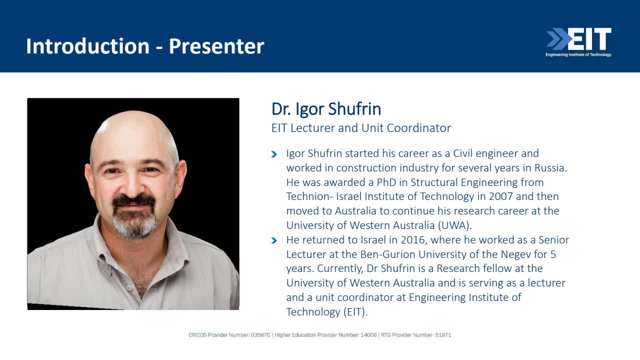 so we can model technically anything which is moving, vibrating and can be made of composite materials. All right, so, and today I will be talking about application of composite materials in construction, So I will probably share the screen first, And it should be this: 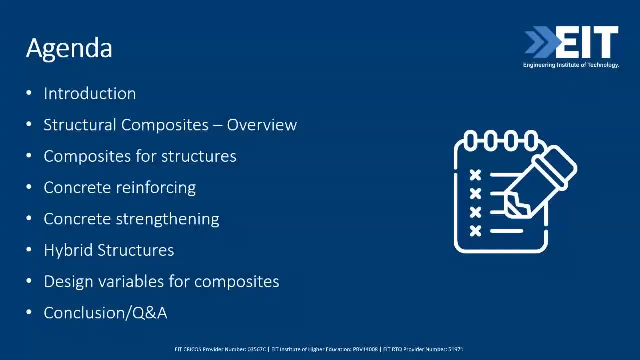 All right, All right. so the topic of this webinar, of this presentation, is composite materials in construction. Like I said, this is a very exciting and innovative area, but the title sounds too broad to capture this in one hour talk, So we'll need to. 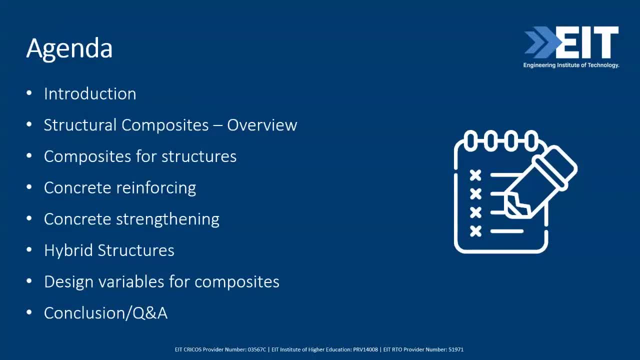 we'll need to narrow this down, So what I will do is I will focus on structural applications One. in the last two decades, the field of composites has grown enormously. A huge range of non-structural components is produced nowadays using composite materials. 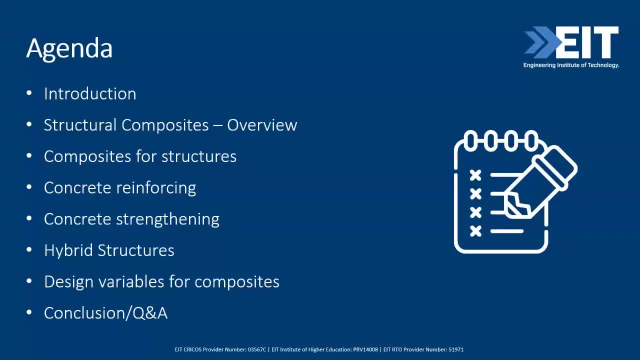 which includes some architectural elements: building envelopes, thermal insulation, windows, smart walls, so many- And they all belong to the area of non-structural elements, So I will not. they will not be our goal today. The main objective of this one, of this talk. 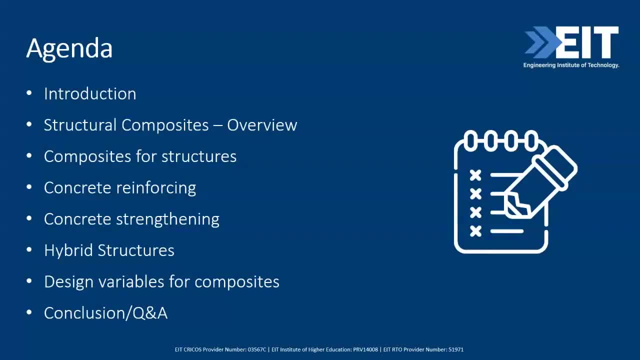 of this webinar is the structural composites And they use in structural engineering the general structure components and they use these components in structural engineering. So the main objective of this webinar is to talk about structural composites And we will talk about this today. 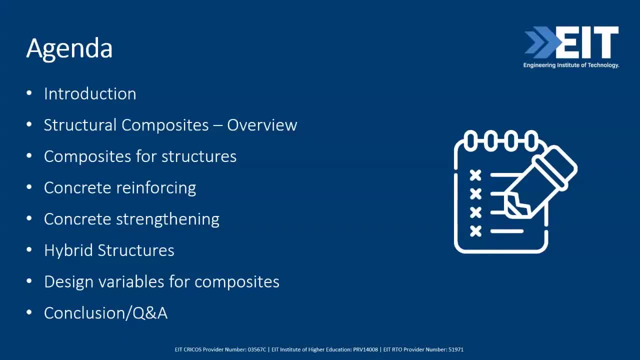 So let's start. So I will first introduce the structural composites, then we will discuss some properties and how it works. then we will see how they can be used in structures, in structural engineering. We will discuss reinforcing- concrete reinforcing. we will discuss strengthening of existing. 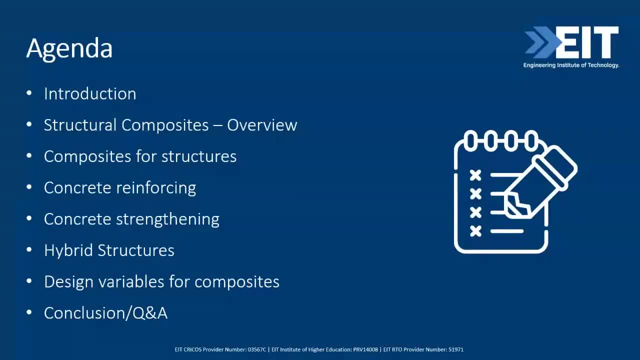 structures using composites. we will, in the end, touch base with some hybrid structures which incorporate composites as well, and I will summarize this by defining a set of variables for design of composite structures, and we'll have some time for questions and 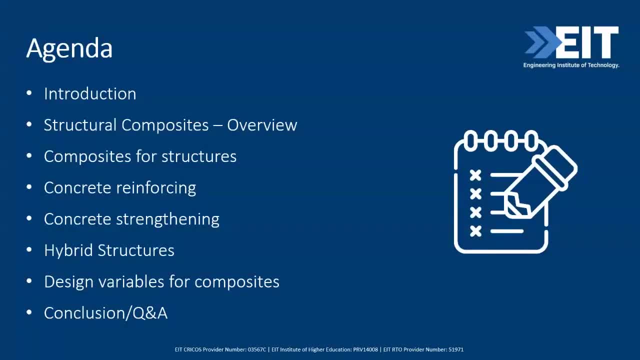 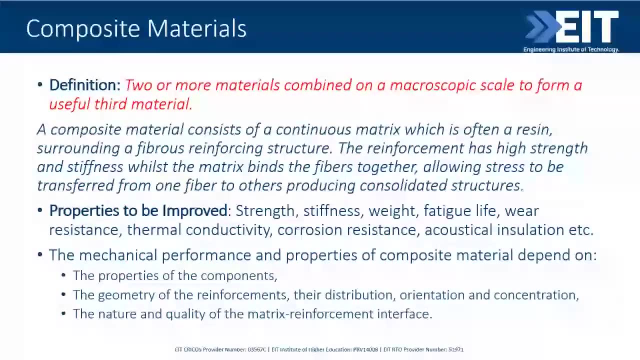 answers Q&A session. Okay, So let's start from some definitions. A composite material is a material made from two or more materials that are combined to produce a material with a third material, which is a new material with enhanced or unique properties which cannot be achieved by the original components only. 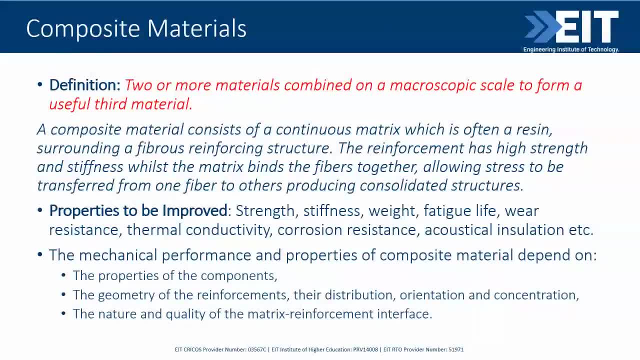 This is the classical definition. There are many types of materials that fit this definition. I believe the most famous one is the reinforced concrete. You would feel that I definitely have very strong structural background in civil engineering because we're dealing with concrete today, but I also believe that the first ever composite 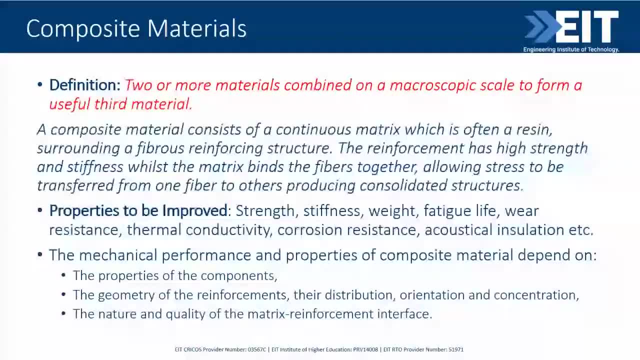 material is the RC reinforced concrete. Okay, Well, that combines. it fits the definition. it combines steel and concrete in a way that they complement each other. Well, the resulting material: no concrete, neither steel. That was the limit. 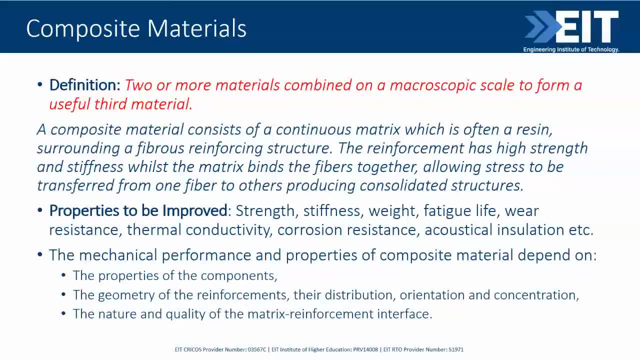 In the structural engineering we have some ratios, so-called reinforcement ratio, which we use to define the amount of steel in the concrete. So in the world of steel we have a lot of steel. So in the world of composite materials we use a volume content of fibers and we 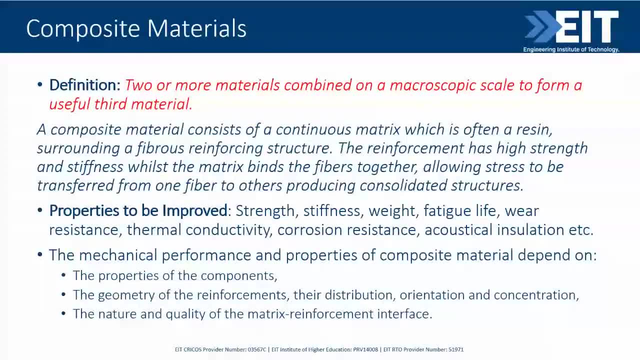 will get to this shortly. So when we combine two materials we call, one of them is a matrix and another one is a filler, So the matrix should be continuous. Often it's a- usually we will get to this as well. so it is some kind of a resin epoxy. 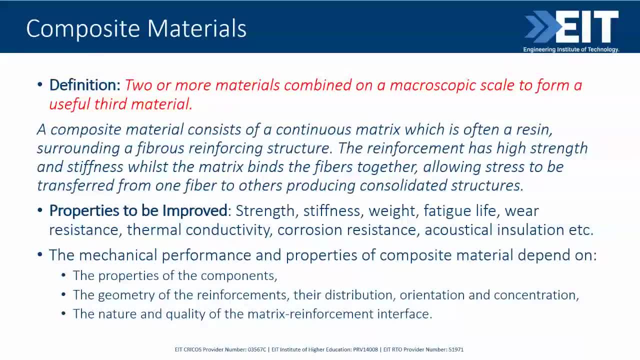 resin. Okay, So the matrix binds together the filler phase, which is which should have higher strength and stiffness, So the other, the filler, must be stronger. So the all together they will form a new consolidated structure. 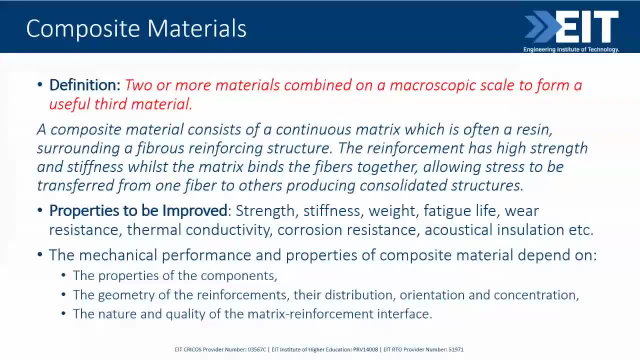 So to create a composite material we need to satisfy two conditions: The connection at the macro level- we're not talking here about molecular or molecular, Okay. The connection at the molecular or atomic levels. we're not designing any chemical, new chemical compositions. 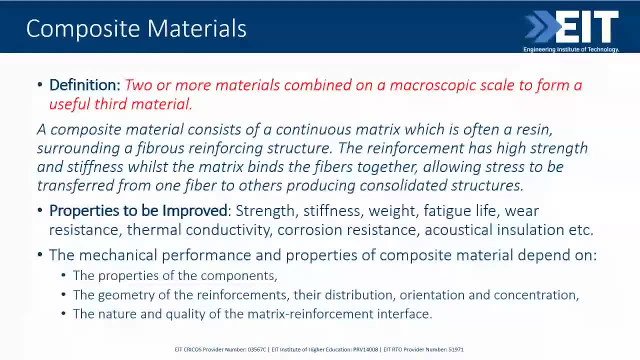 We're talking about combining materials in the macro level which, simply speaking, we can touch, And the second condition is uniformity of resulting material. Okay, So as a result, if we satisfy these both conditions, the mechanical properties will be the same. 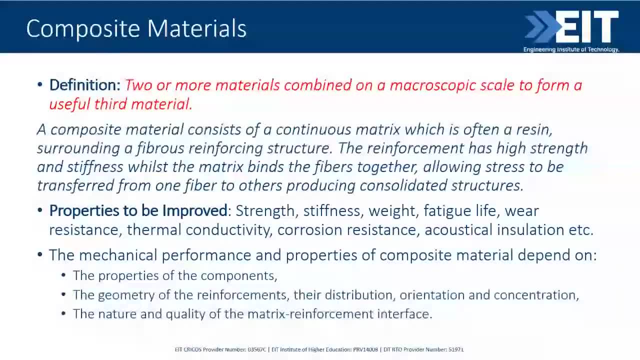 Okay, Okay, Okay. And we, the, the non-mechanical properties or the resulting composite can be defined as effective properties, as some homogeneous effective property, And no matter if I take a flexible matrix and hard filler or I will take a brittle. 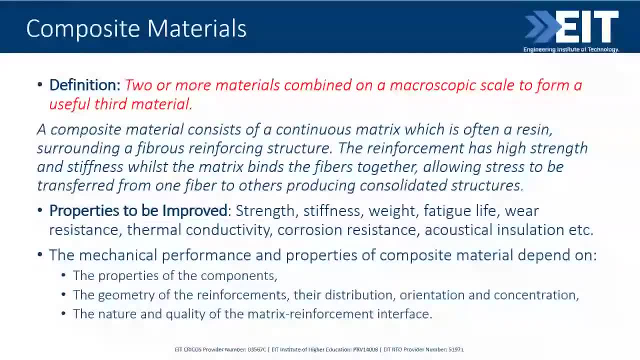 matrix, or it's concrete in tactile filler, or I will take a hard skeleton and embed it into the matrix and create a newiram. Okay, Okay, that protects it in terms of temperature or corrosion. so if this action is uniform, the material, the resulting material, is the compass. so with this, 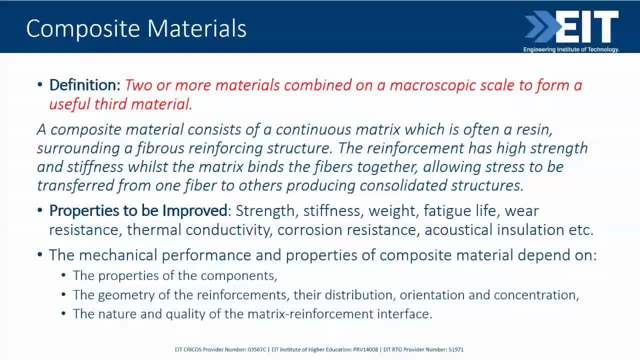 composite materials. well, when opening the range of possibilities- infinite range of possibilities- we can achieve different goals and increase strength. the stiffness can reduce weight, which usually comes as the specific strength. stiffness because we want to achieve some strength as per unit weight. right, so we can improve wear resistance, durability. we can play with thermal. 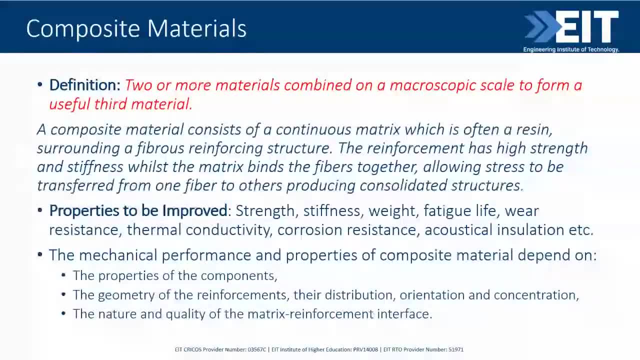 properties. we can change it from positive to negative, thermal expansion, for example. so the least is long. the performance, or composite, depends on the properties of the base material. geometry of the fibers. this part is completely clear. structural engineers running we know, we change, we know where to place. 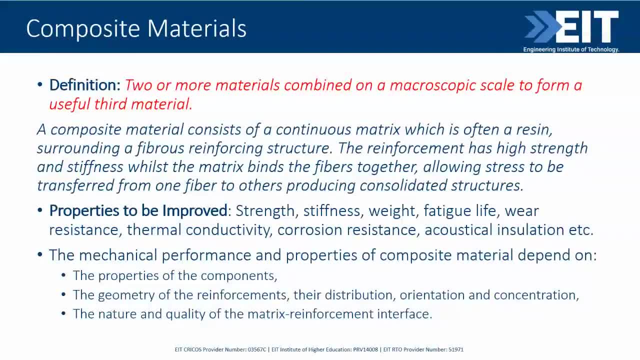 reinforcements, rebars into the concrete plate. the quality of the material is quite high. the quality of the material is quite high of the interface between the materials, so we need this completing a complete bond between them in order to ensure the uniformity, all right. so, as a result- and often we not, we should not mix the uniformity in a isotropic. 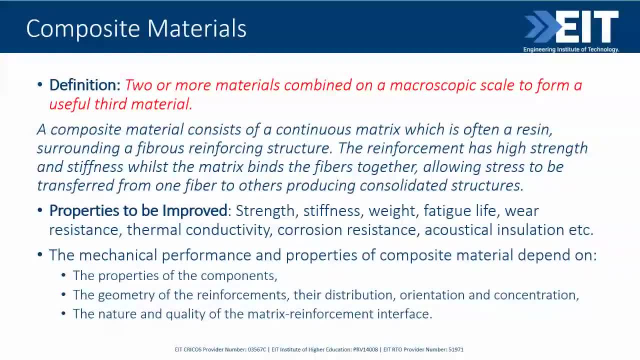 because the compost materials are anisotropic in nature, so they have different properties in different directions, even though they still uniform. so in this anisotropic nature of a composite lies the main advantage. so there we know. the reinforcement can be designed to follow the stress pattern in structural knowledge. 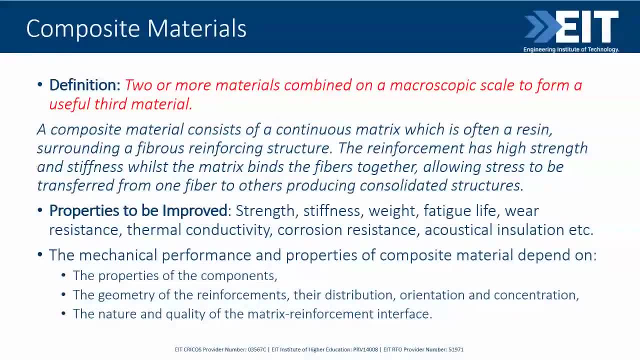 concrete design. we know this. that's what we do. we use the reinforcement and the places where we need it. so similar idea can be used for composite materials so we can improve the performance and we can achieve the much better performance than the traditional isotropic materials. so there's some classification. so this classification- 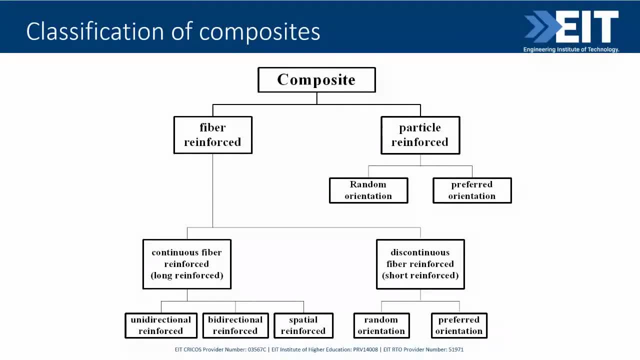 of of composites follows the basic, basic concept we defined earlier: a matrix. matrix made of one material being reinforced by another material. so the reinforcement. second, so reinforcement phase, can be either fiber or particle, so both can be random or randomly oriented or arranged in a certain way. the fibers which are 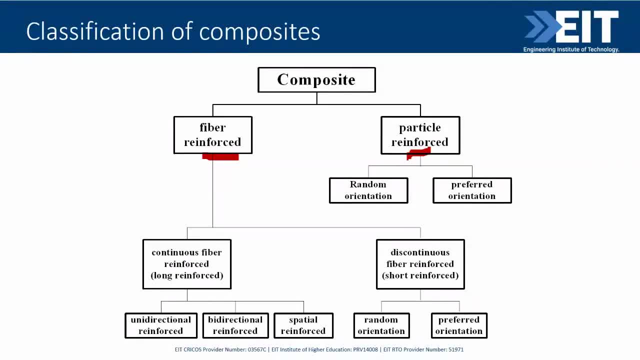 more important for this tool can be short or long, can be show oriented randomly or arranged in a certain way, and they can be long. facts can be short or long. facts can be super restricted for some. what does that mean? so the log fibers are usually continuous and can be set in one direction to. 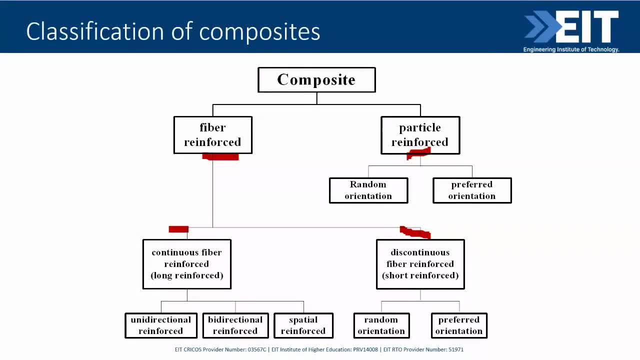 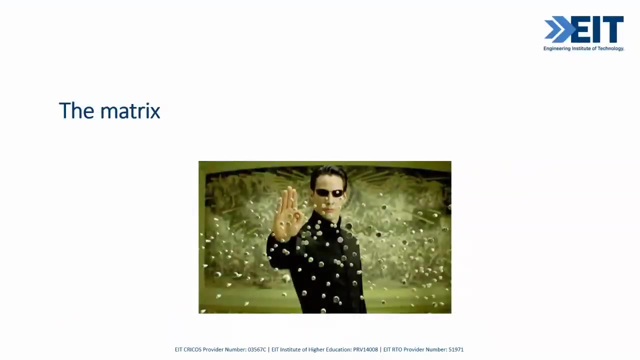 orthogonal direction or in any predefined angles. all these options here, so well. next we'll have some brief insight in the properties of matrix and fiber materials used for structural composites, and then we will look at the effective properties we can achieve using that. so first is matrix, so the 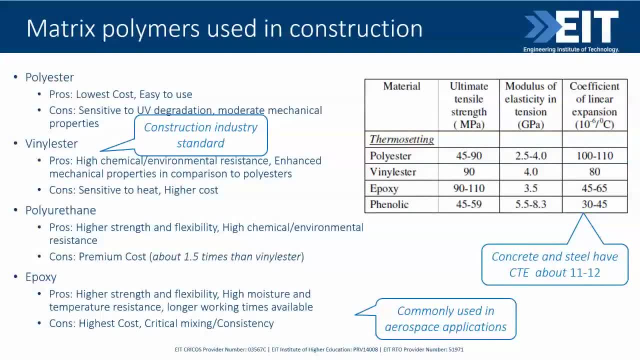 role of the matrix space, as I mentioned already, to bind the fibers together and to protect base surfaces from external influences and bridging environmental degradation. and so they, the matrix also, should maintain the position of fireго's guess. we arranged dem hebt NP-139. the matrix also transfers the stresses to the farmers. 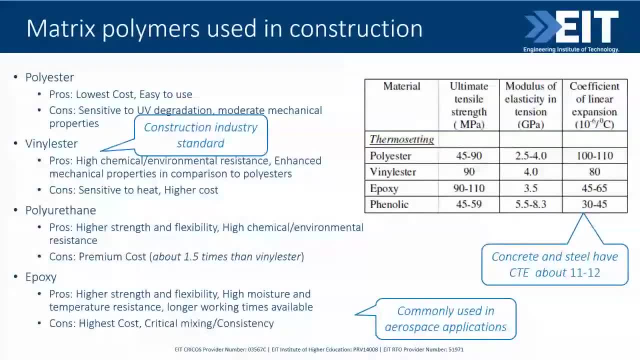 by adhesion or by friction, the. so this requirement should be coupled with adequate matrix. shear strangulation now, in addition. in addition, the matrix has to maintain the position of fibers and the mesh good was covered by two non preventative methods. dvd-100: amazing methods to paint with this word找 31 00. 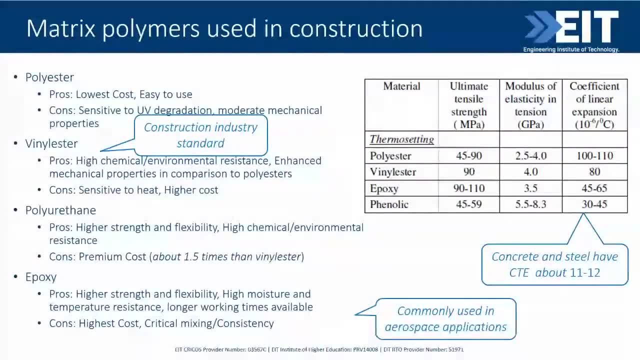 maintain the chemical and thermal composition, so compatibility with fiber, or they will not affect each other chemically. and the matrix provide the color and surface finish for the aesthetic view, so for any architectural elements. so the matrix materials used in structural composites are usually polyester, uh, featured by the polyester actually. 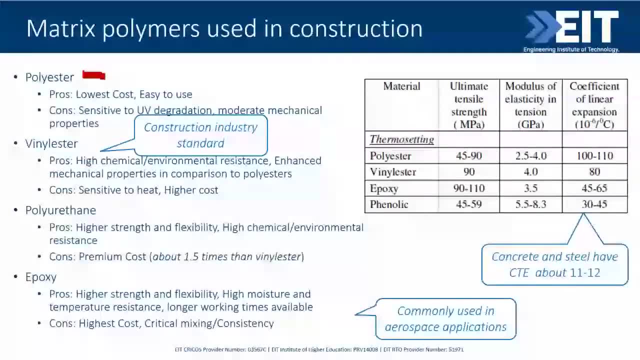 featured by low cost and easy application. however, it's quite sensitive to uv lights and has a quite moderate mechanical properties. what you see here and not so, it's only 40, about 40 to 50 megapascal strength and modulus. modulus of elasticity is up to four gigapascal, so not great. 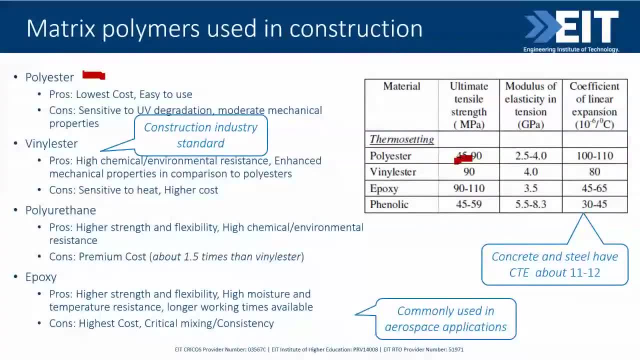 the next one is coming: vinyl ester, which is a higher chemical, environmental resistance and mechanical properties, better- and that's better- than the polyester. we can see here was increased ultimate strength already to 90.. uh, which is actually the vinyl ester. dude is relatively low. 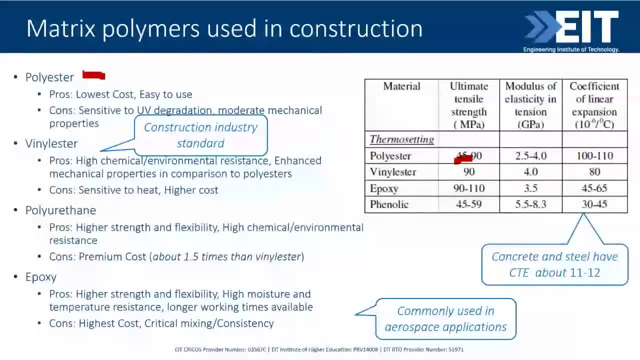 cost is is the preferred material in construction industry, which is slowly changing nowadays. so the disadvantages of this are is sensitive to it and they still still higher cost but relatively cheap up in order in comparison to the other ones. so the polyurethane is the next one is probably the best. 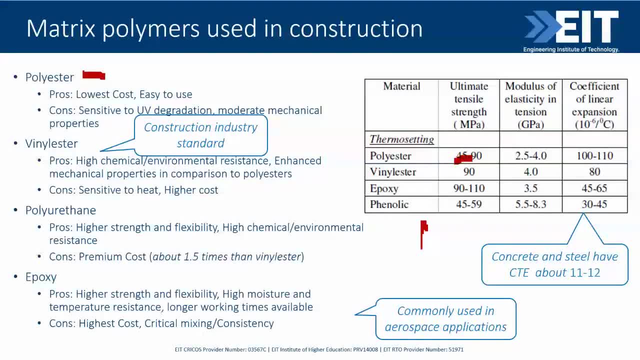 doesn't really appear in my table here, however, because it's too costly, still too costly for construction. that's the only reason. so the higher strength in the flexibility, very high chemical environmental resistance, so it is very, very good material for this. uh, the main disadvantage of this is the 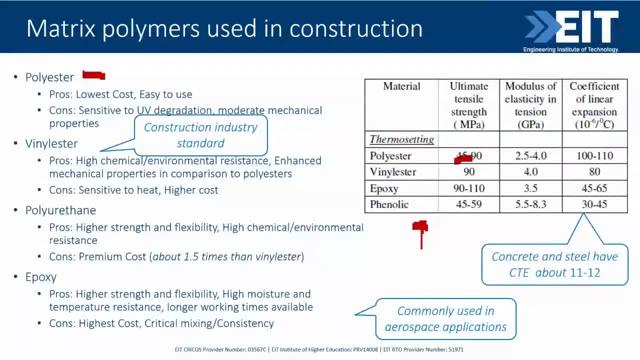 premium cost. it's about one 1.5 times costlier, costs more than in vinyl ester. well, the some most useful, most popular one, also the which you hear everywhere, it's epoxy resin, which provides high strength and flexibility, high moisture and temperature resistance. so that's the moisture temperature. 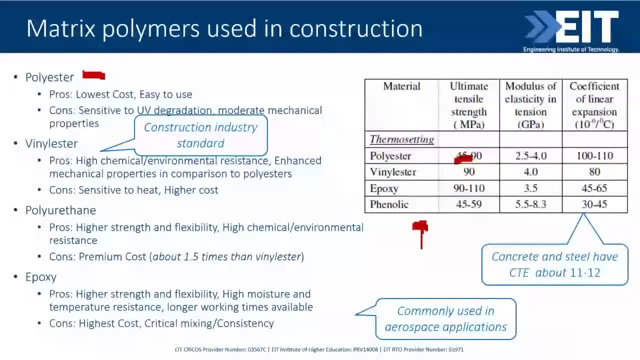 resistance. all the curing time is a bit longer, so we can provide longer working tasks, which sometimes becomes important. the cost is still a bit high, but it's getting better nowadays and the critical mixing consistency is a bit hard to get, but the end- that's the problem in construction industry- we need 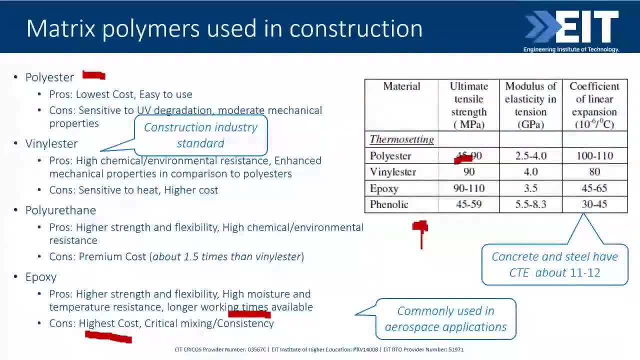 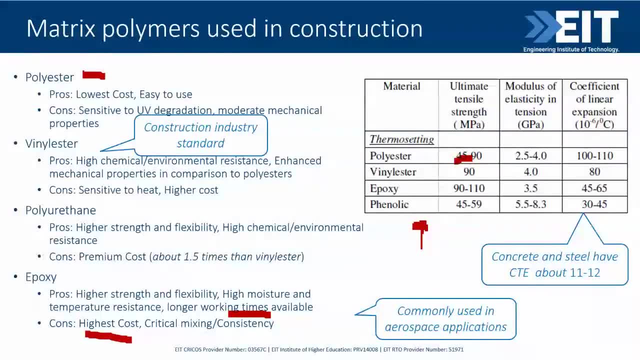 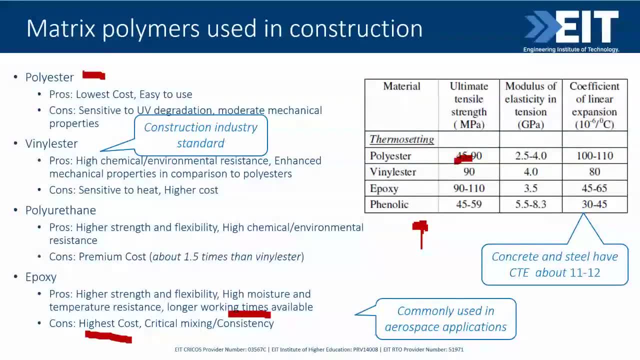 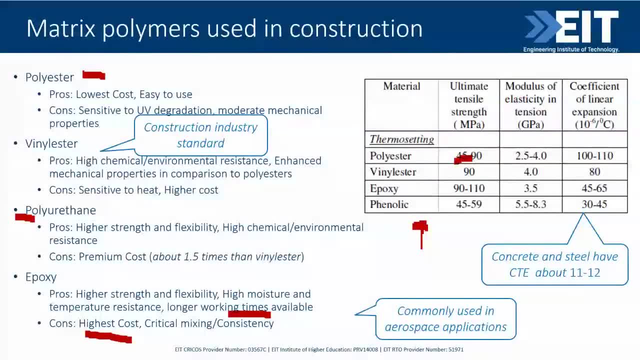 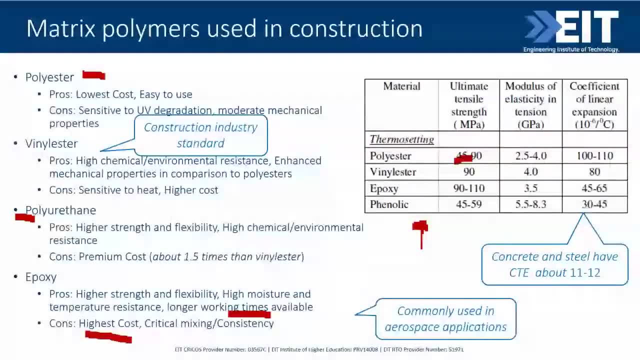 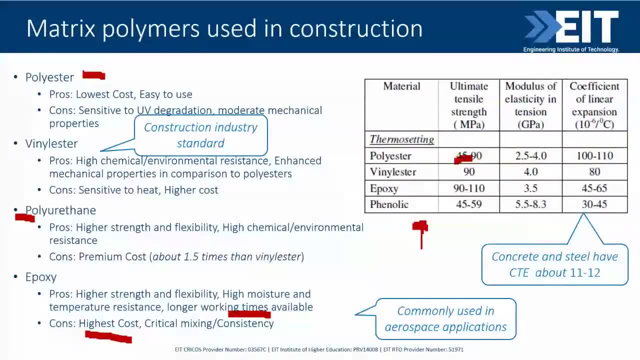 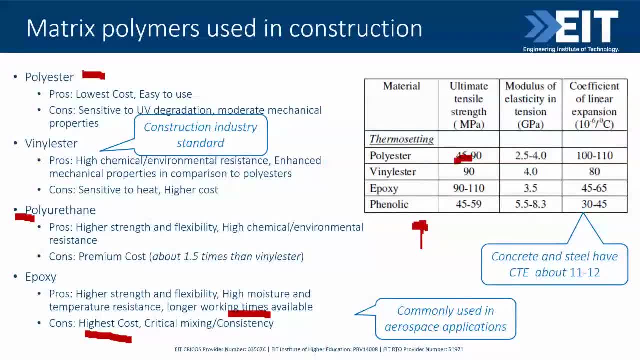 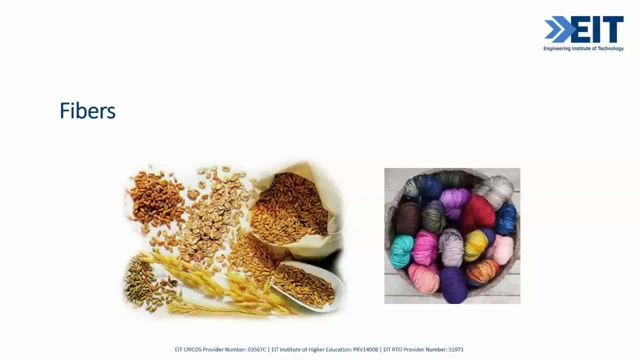 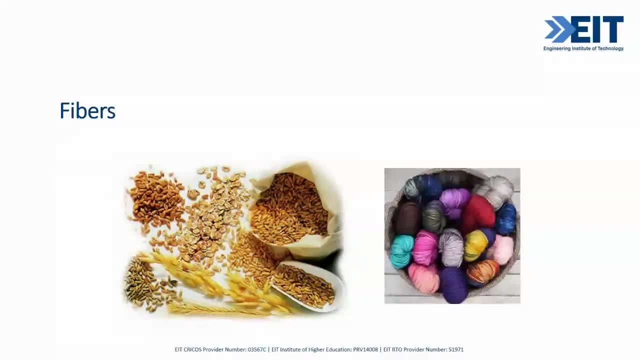 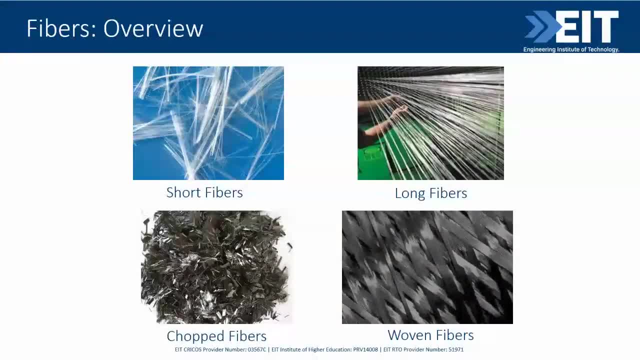 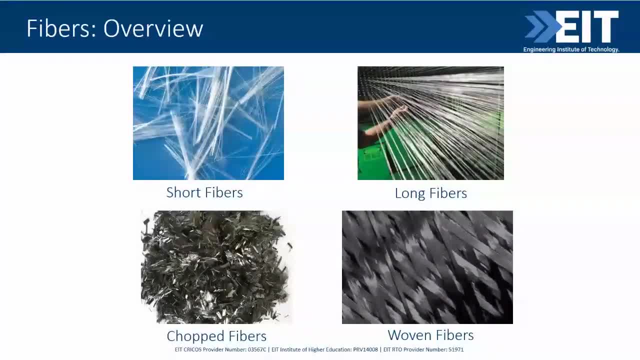 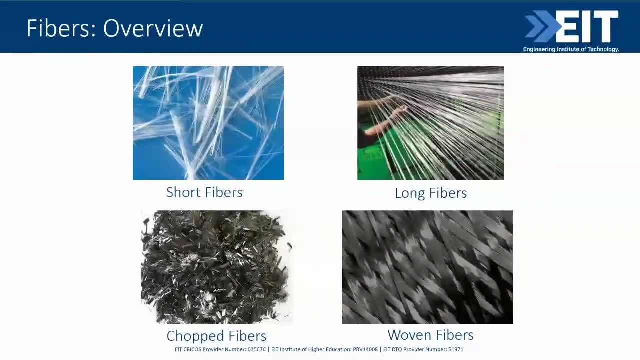 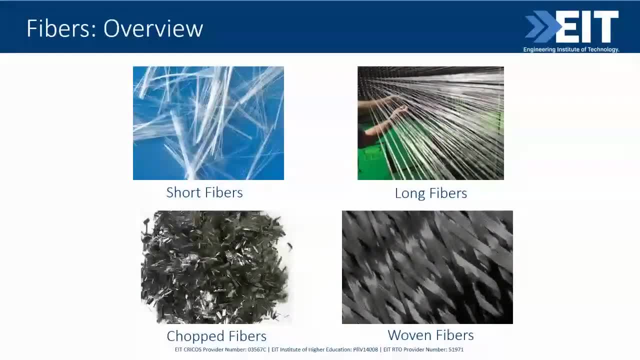 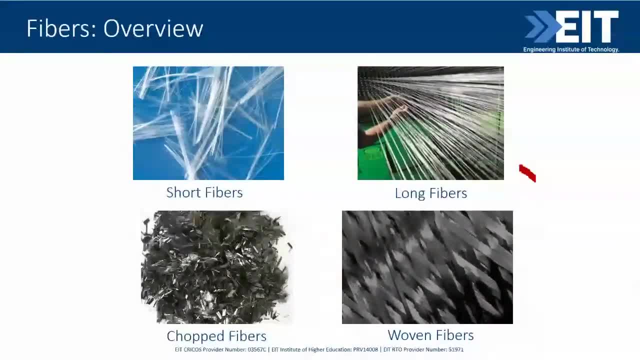 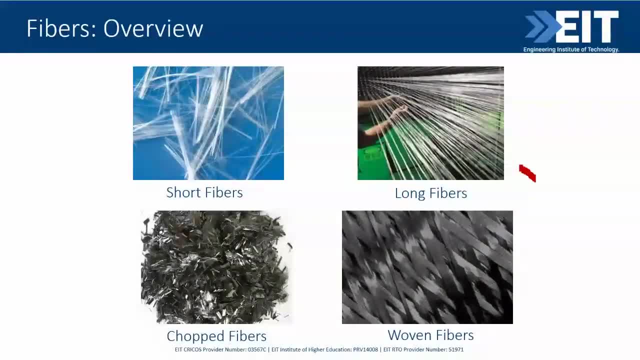 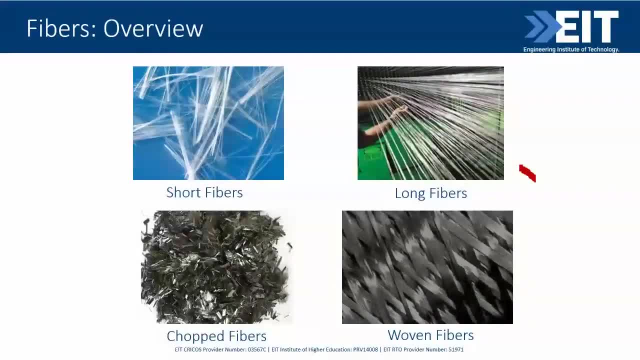 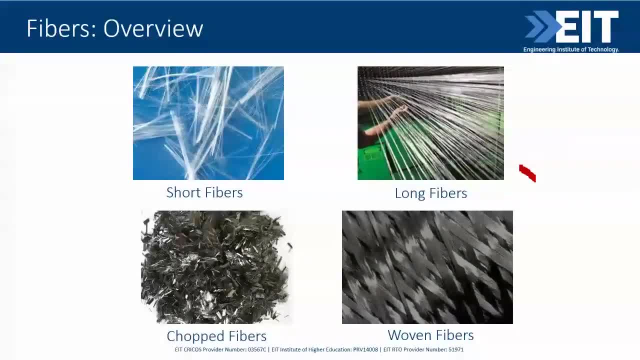 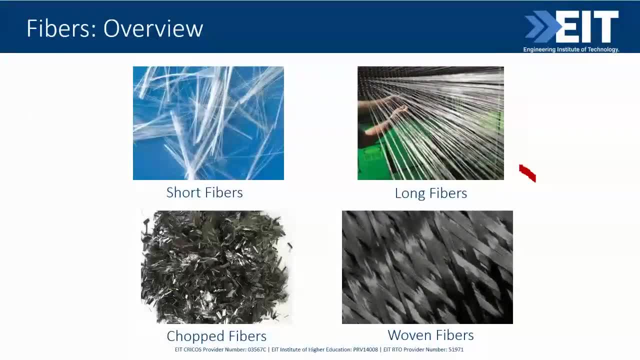 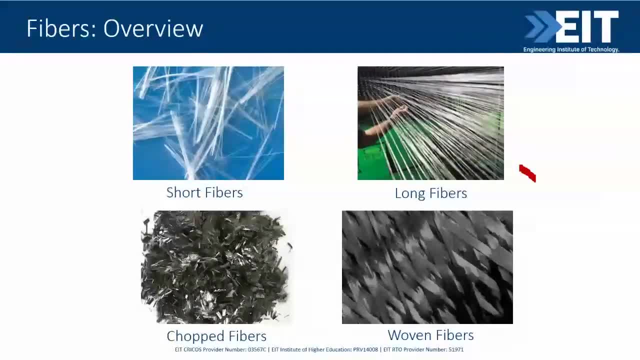 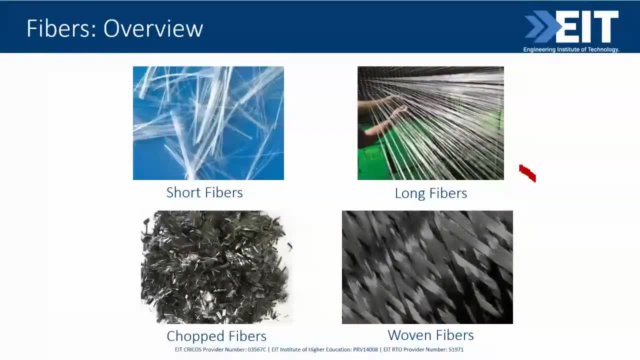 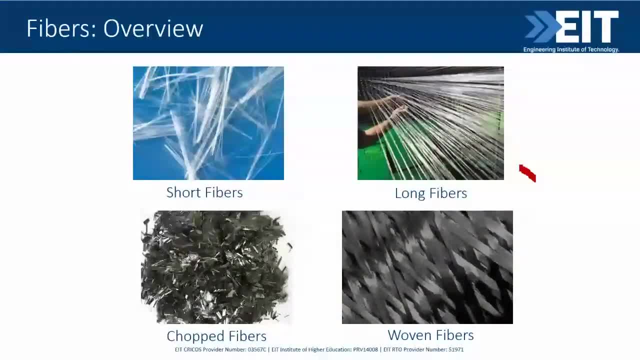 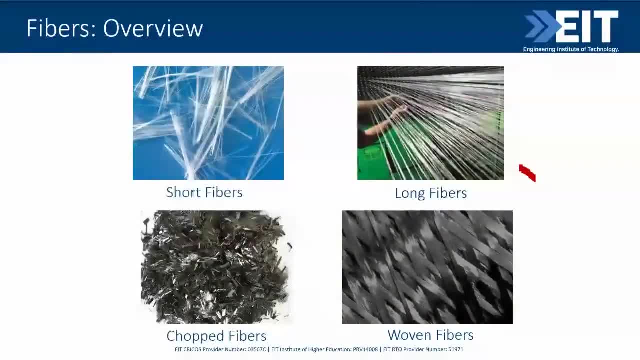 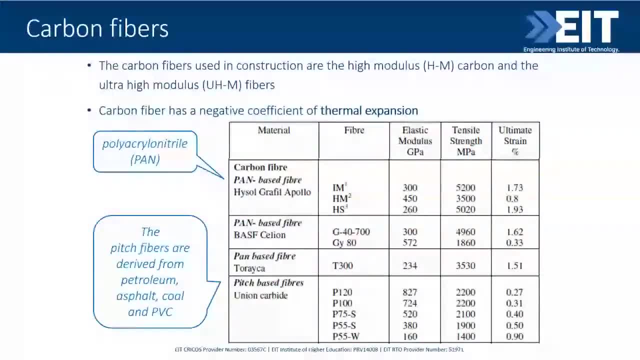 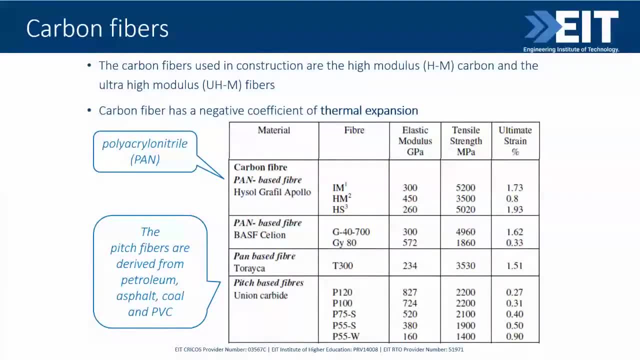 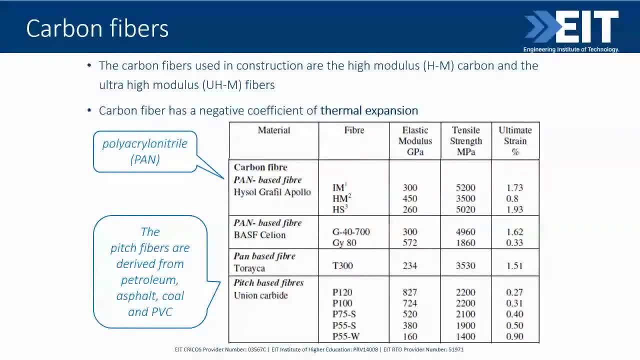 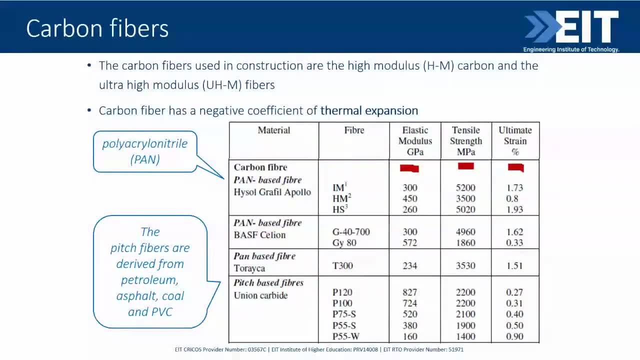 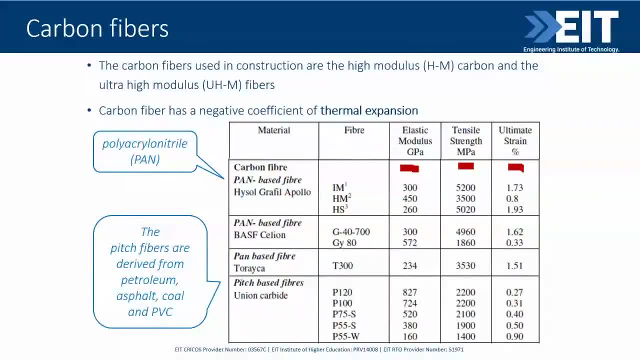 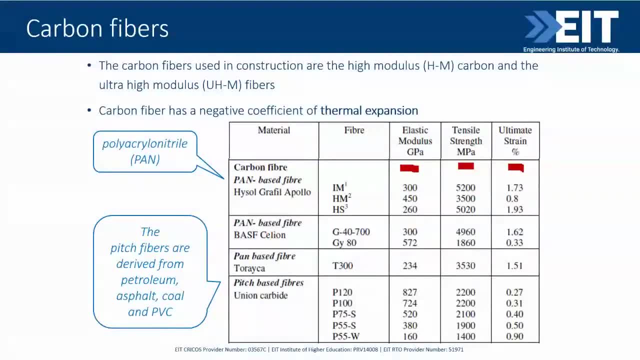 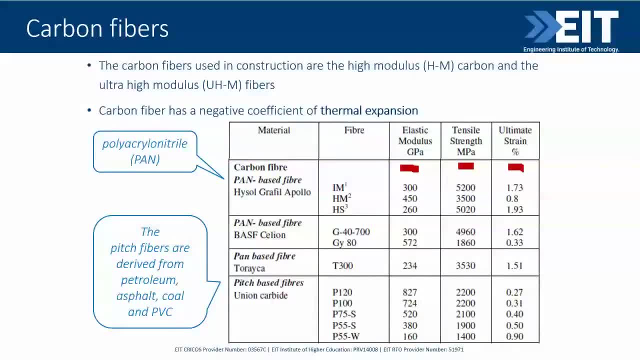 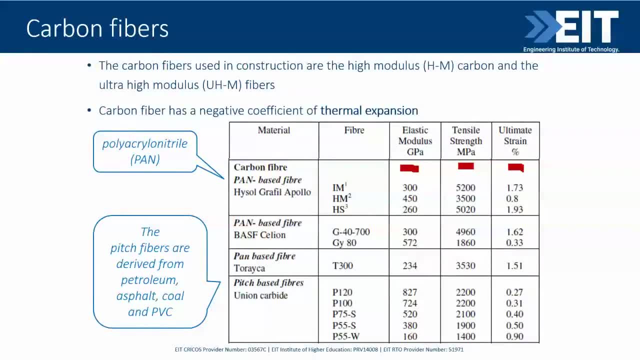 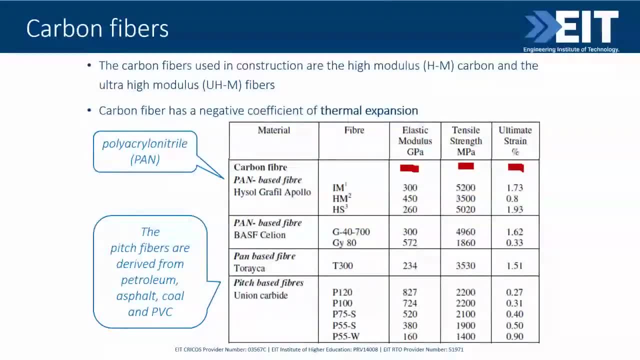 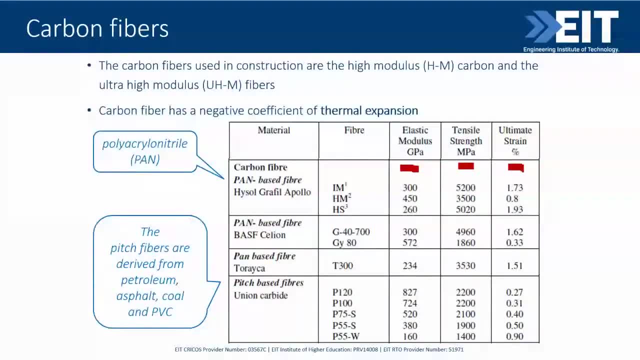 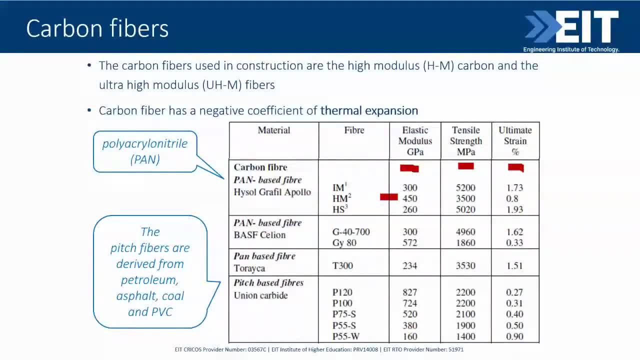 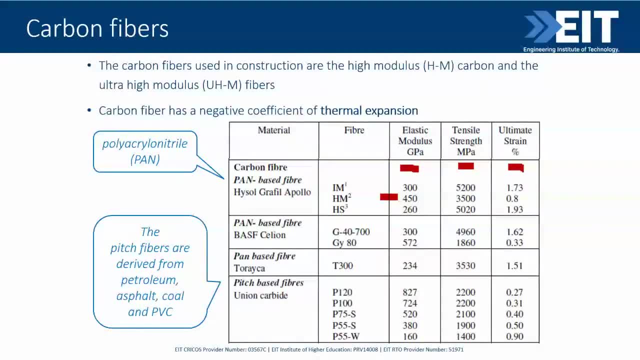 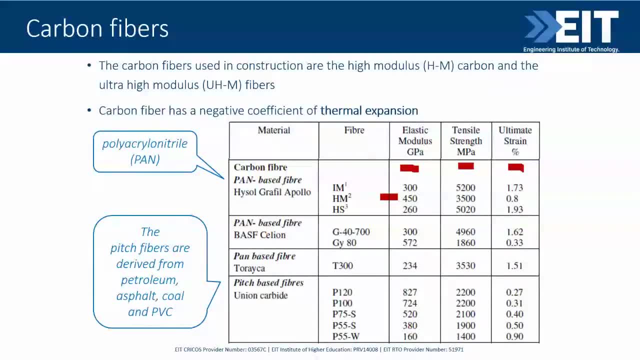 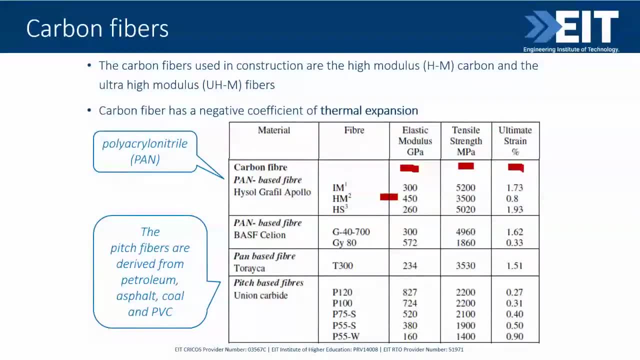 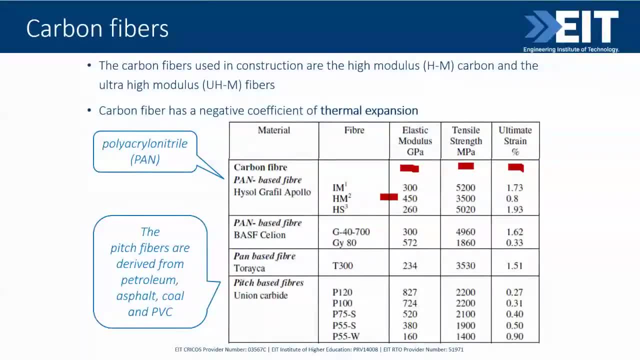 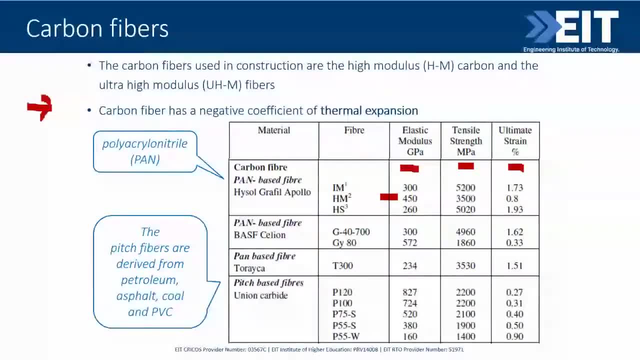 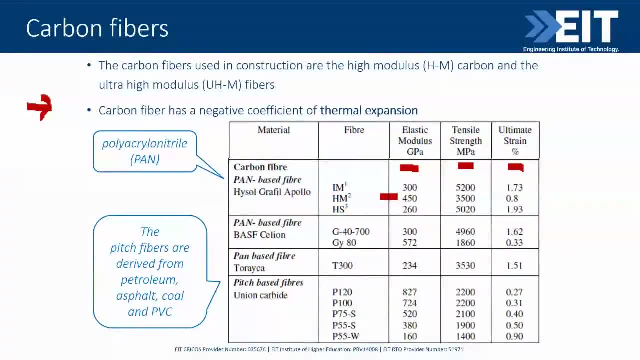 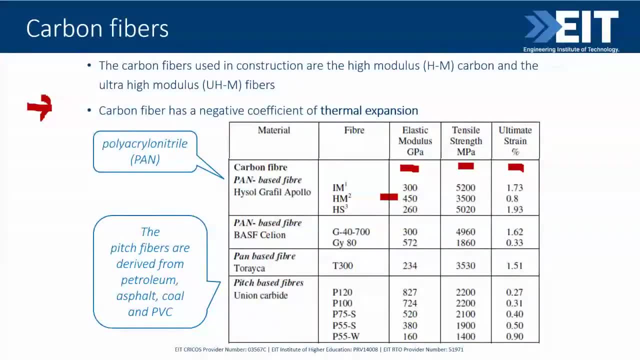 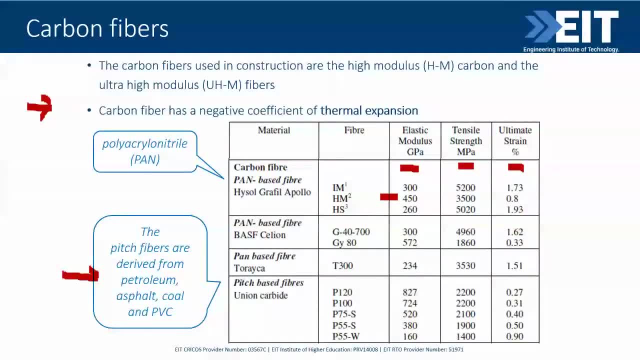 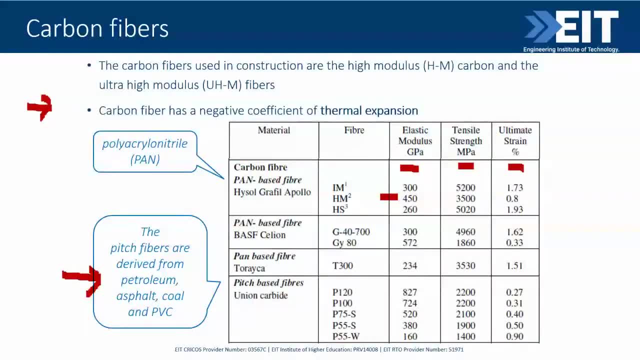 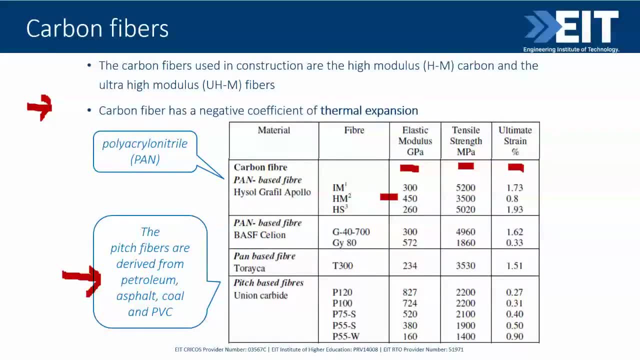 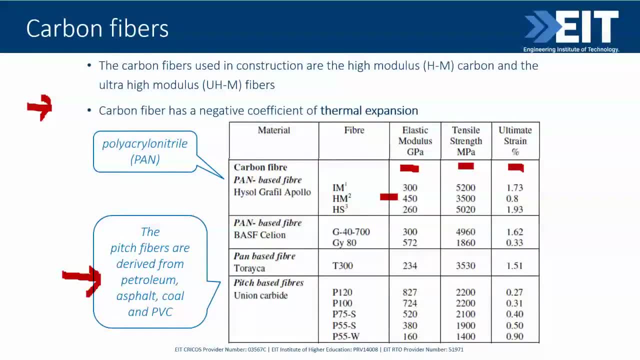 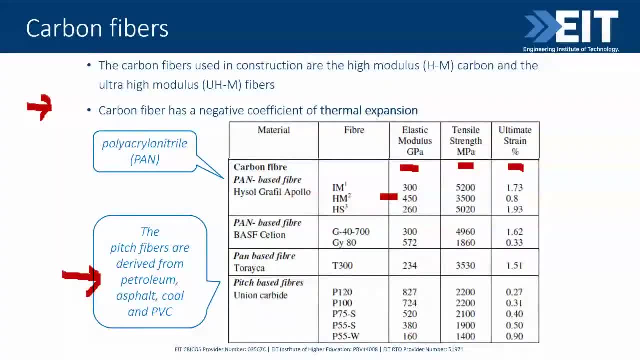 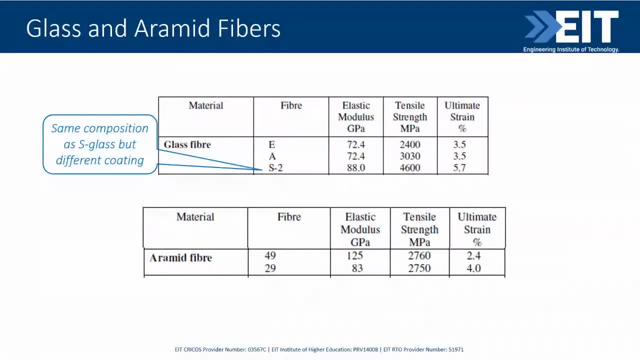 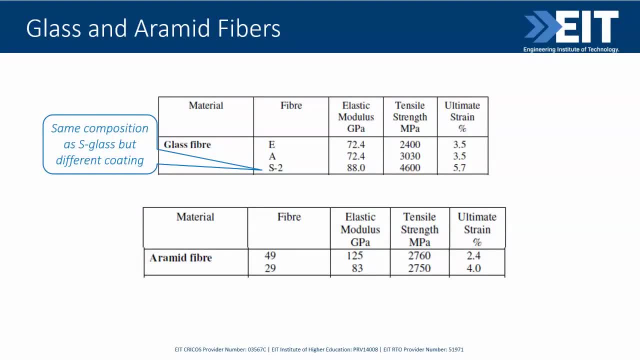 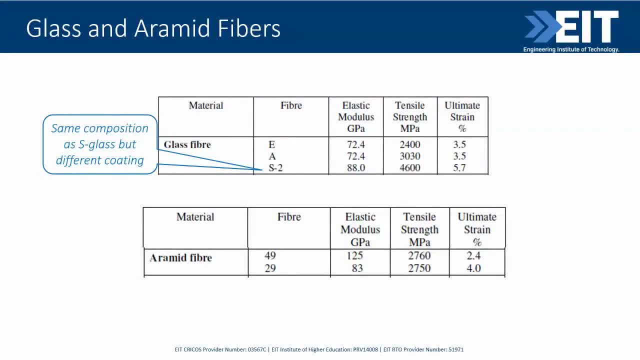 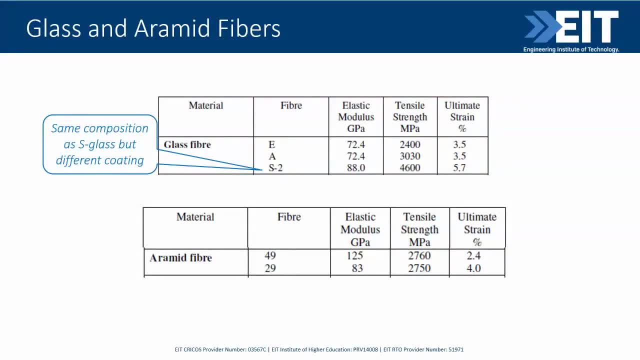 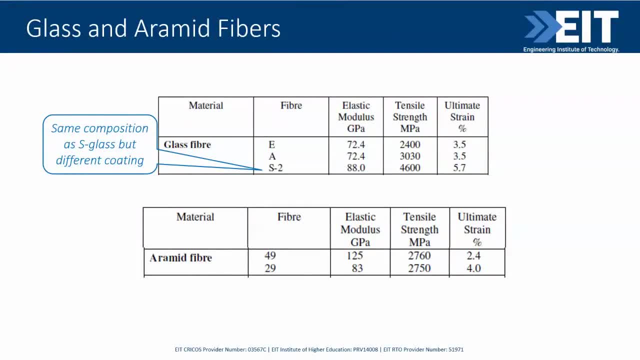 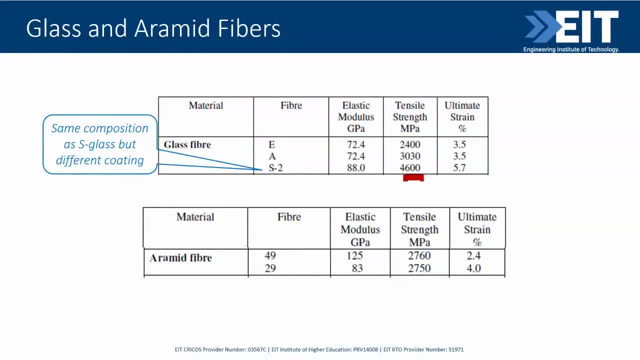 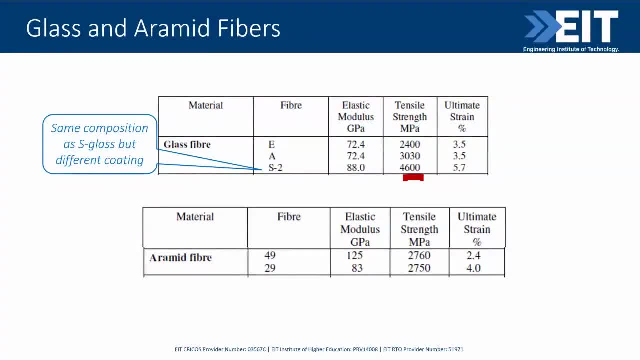 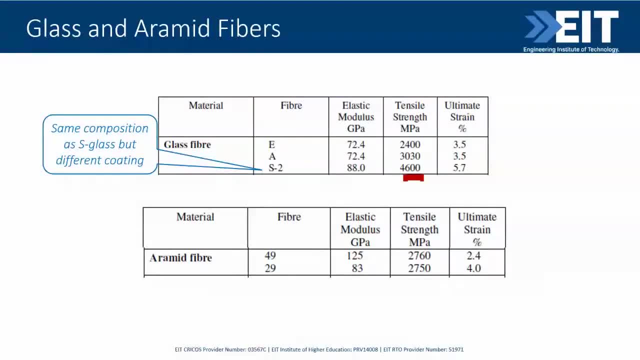 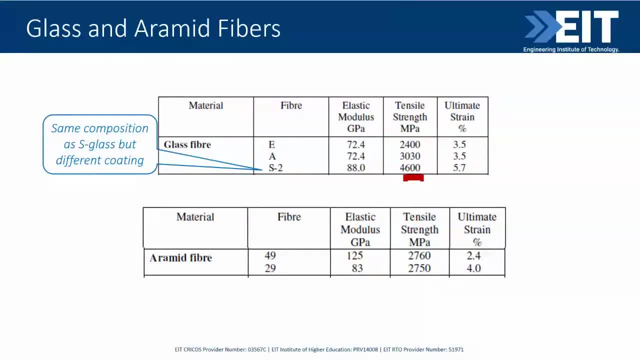 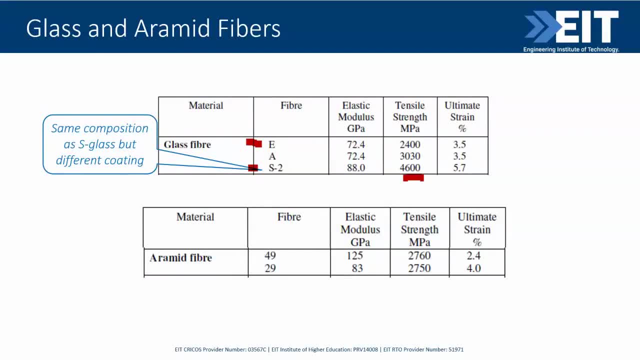 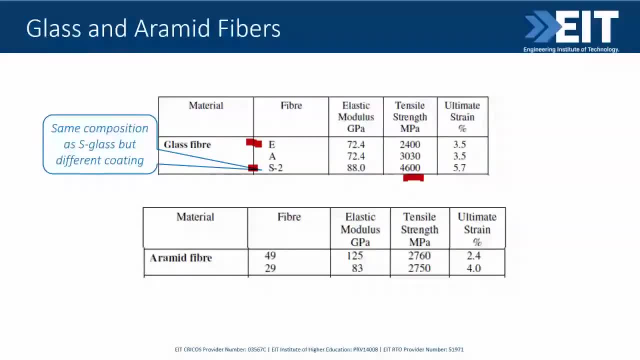 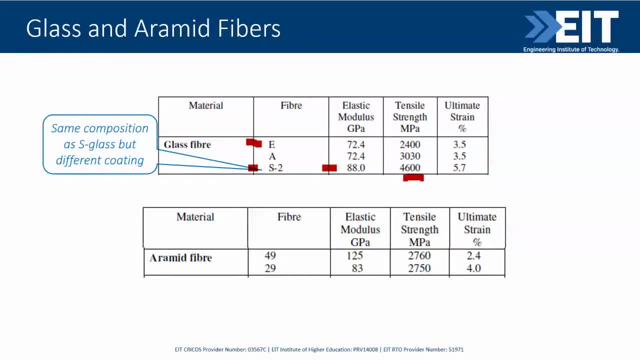 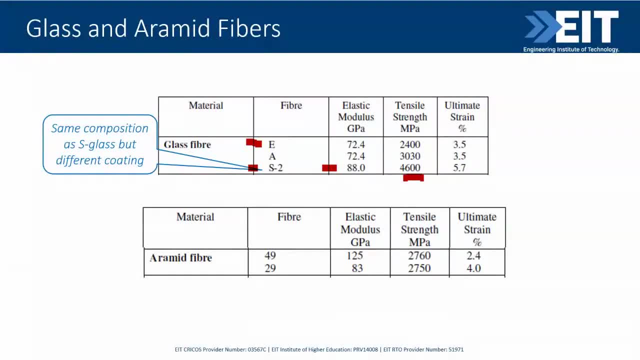 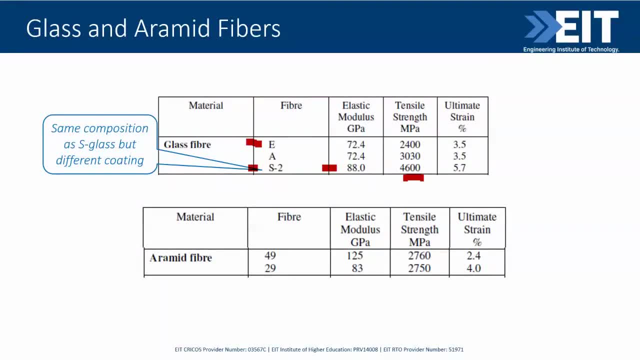 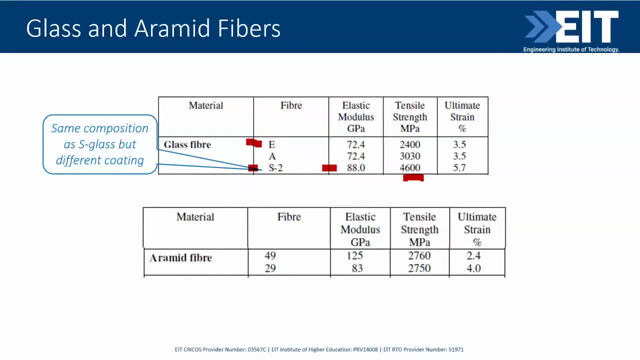 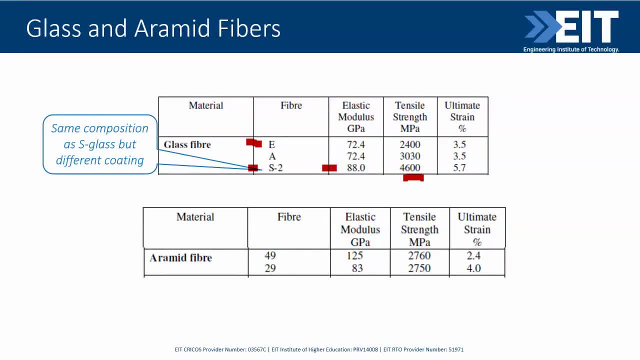 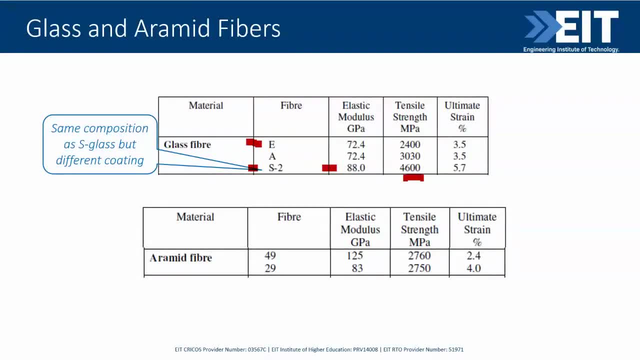 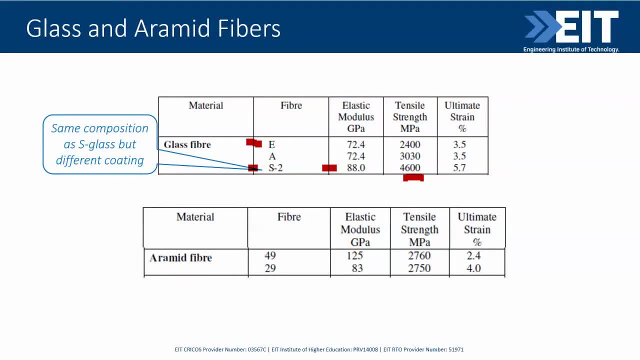 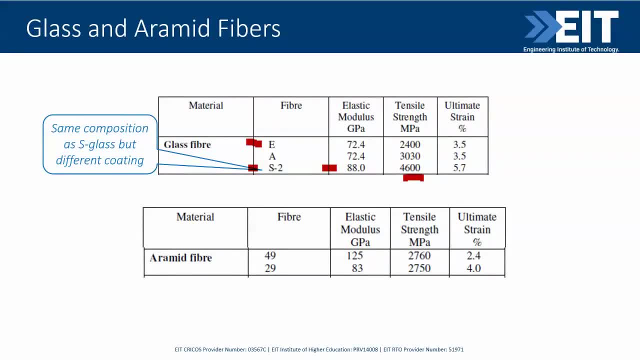 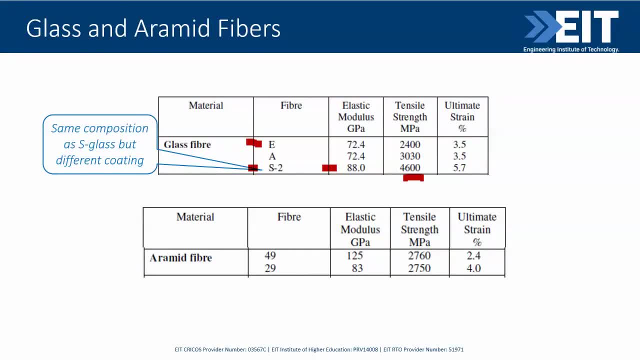 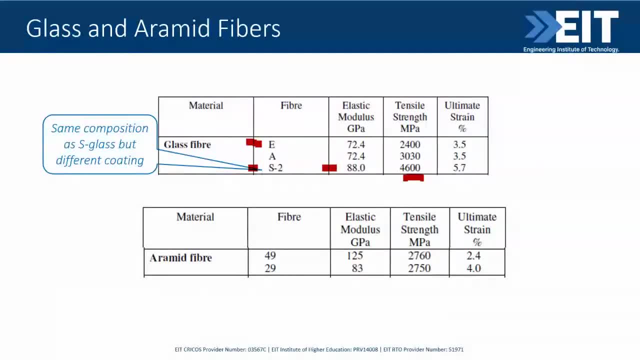 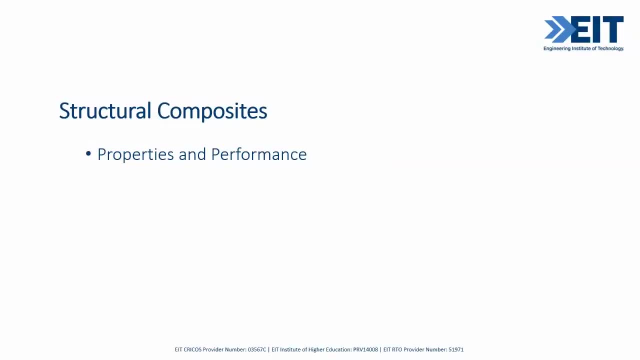 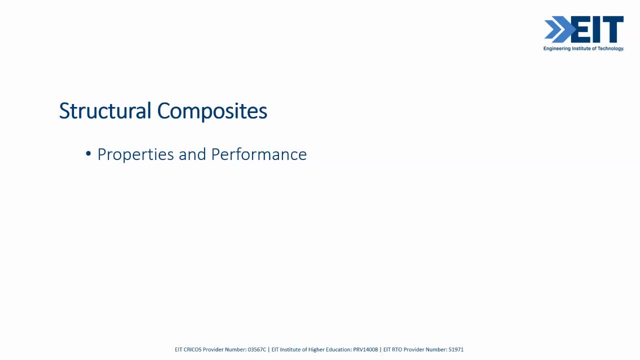 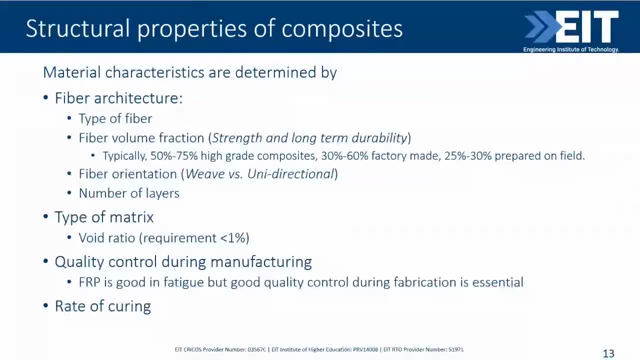 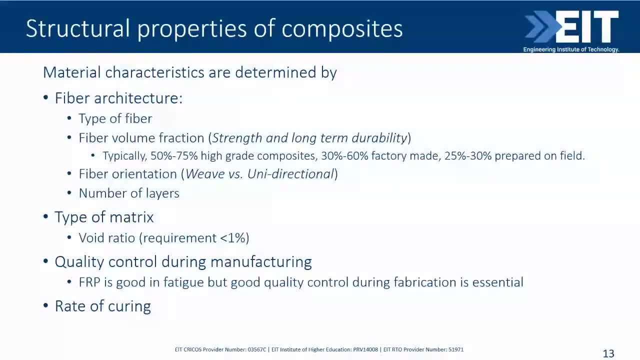 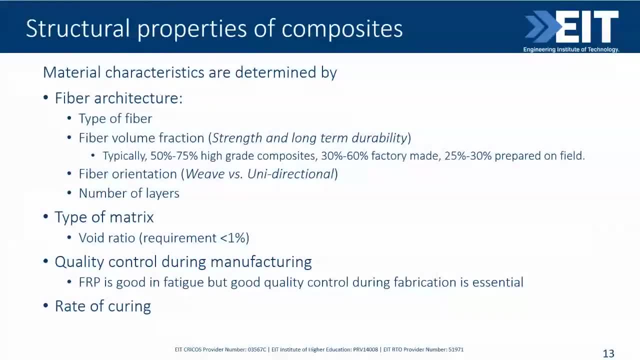 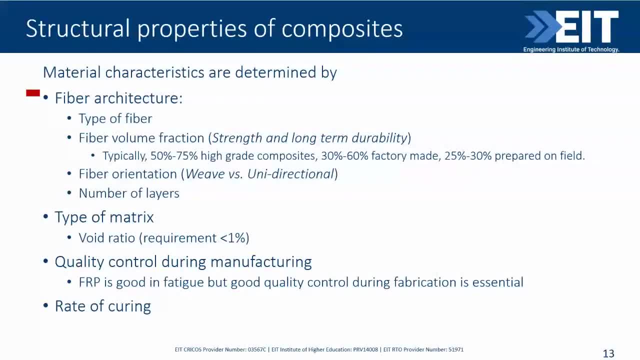 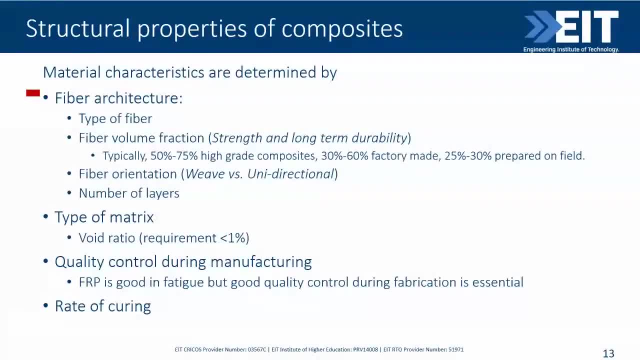 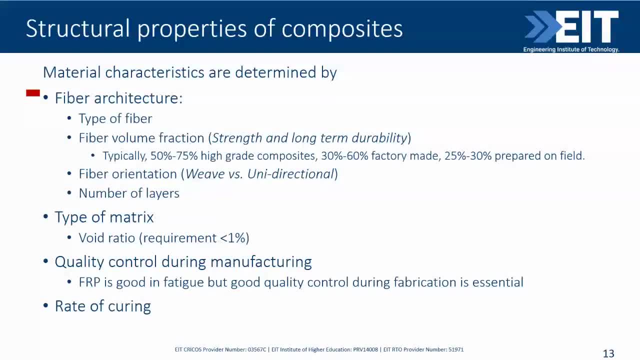 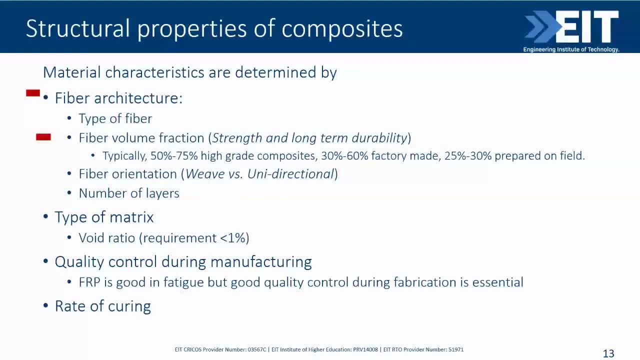 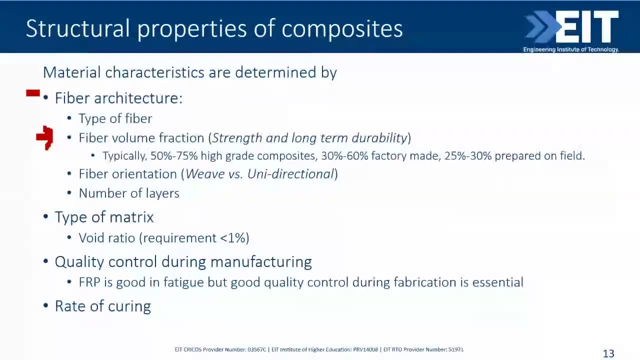 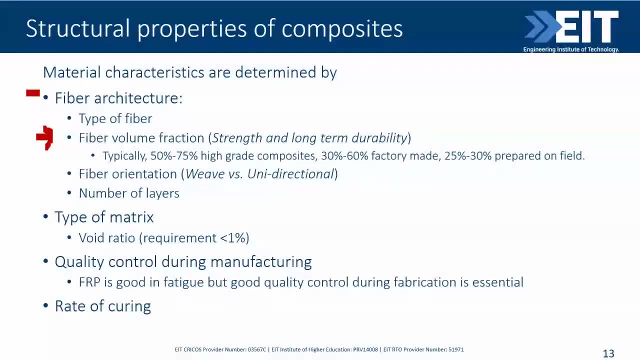 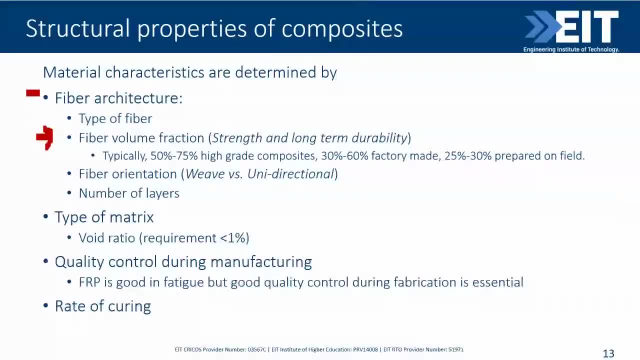 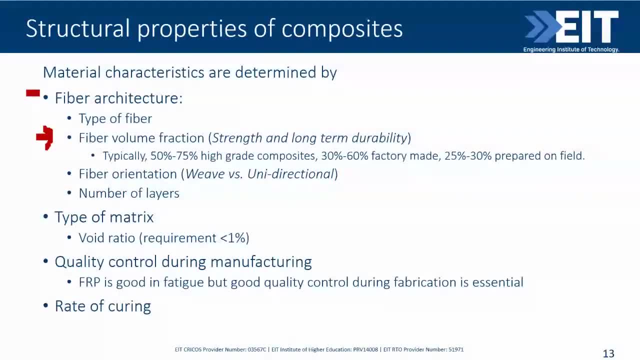 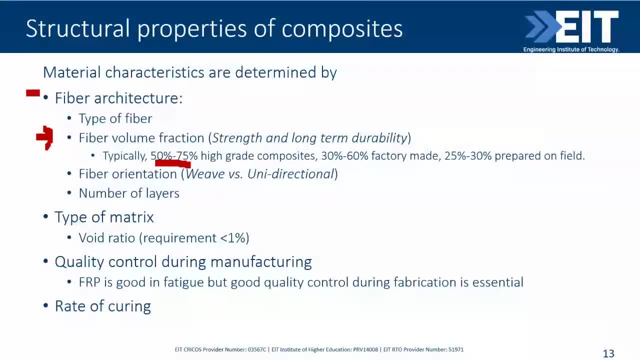 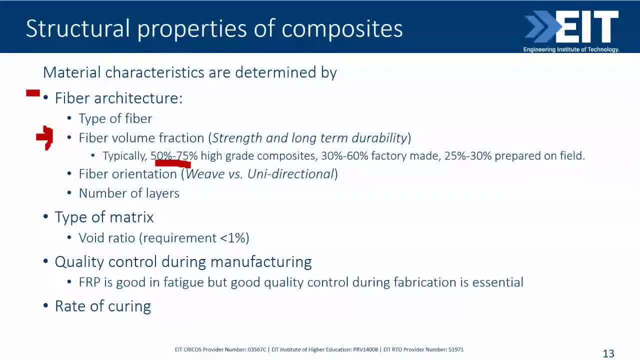 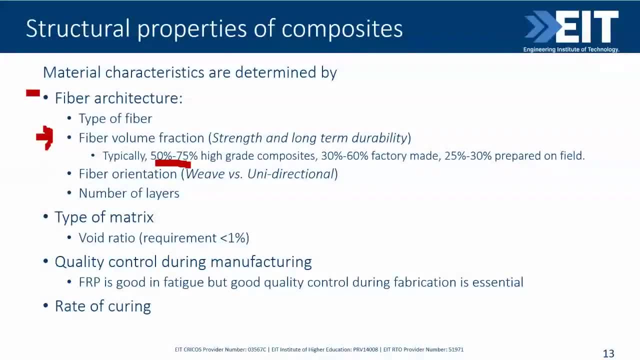 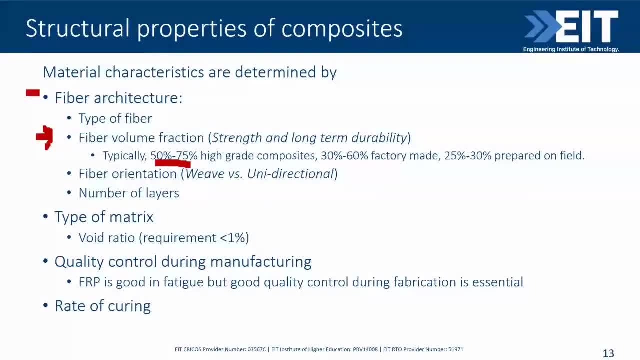 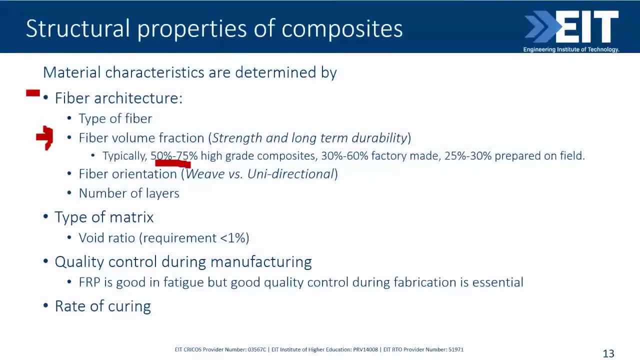 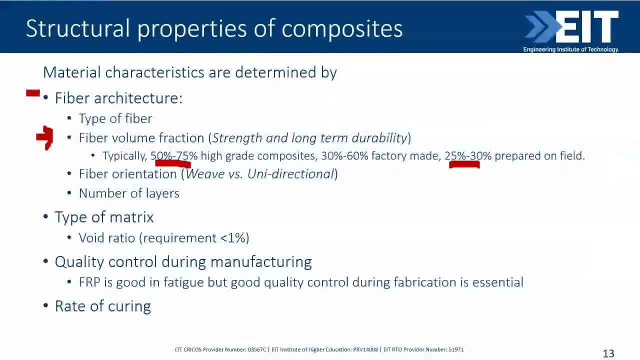 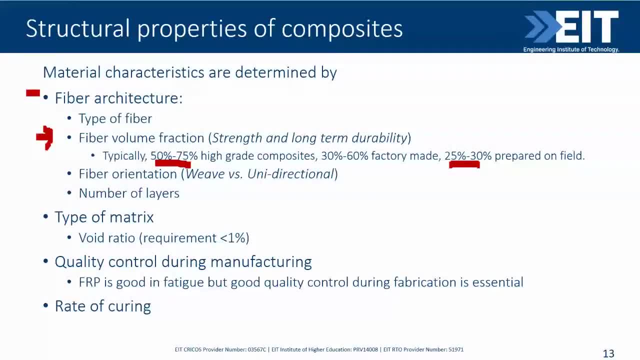 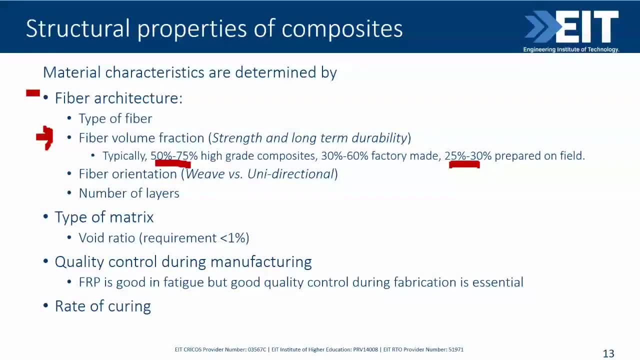 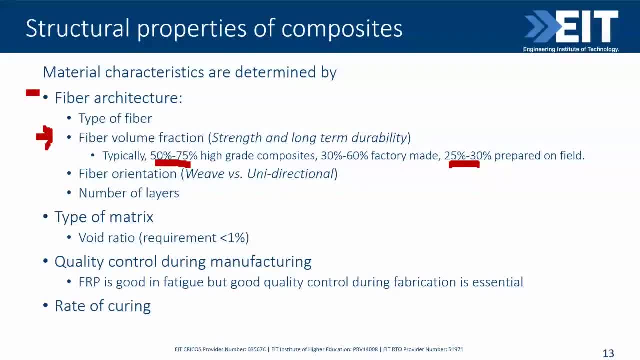 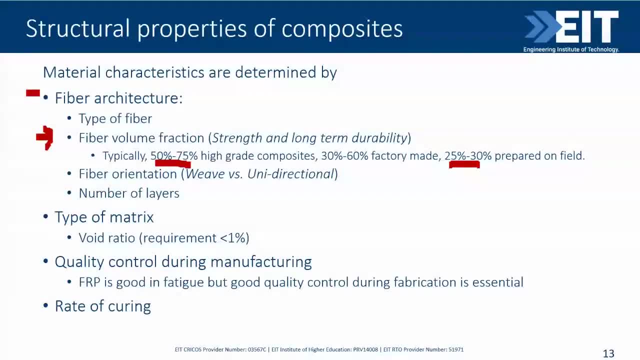 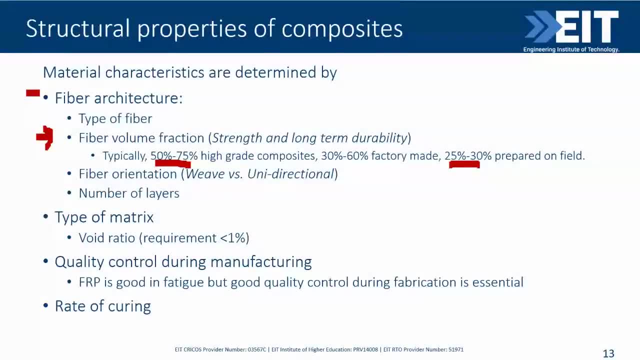 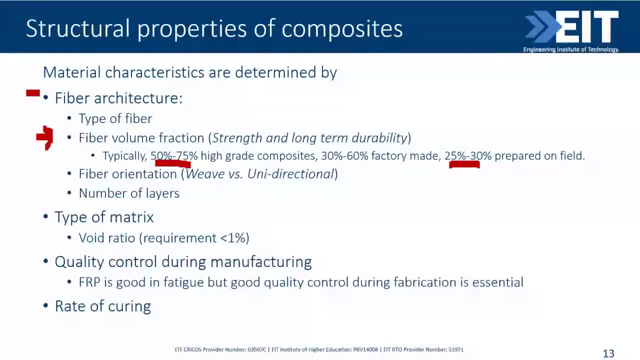 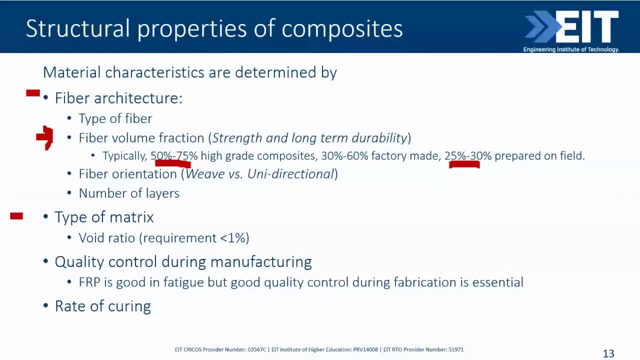 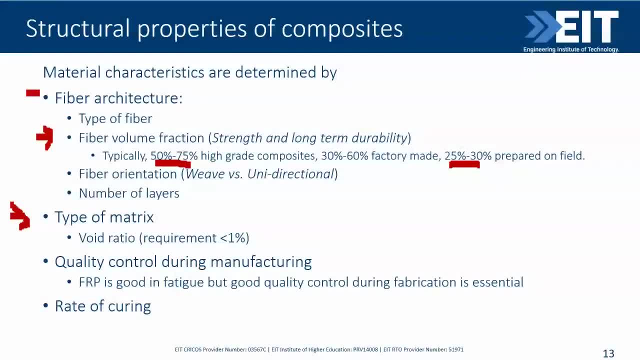 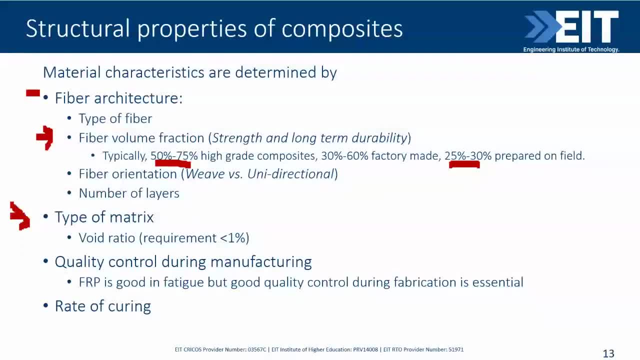 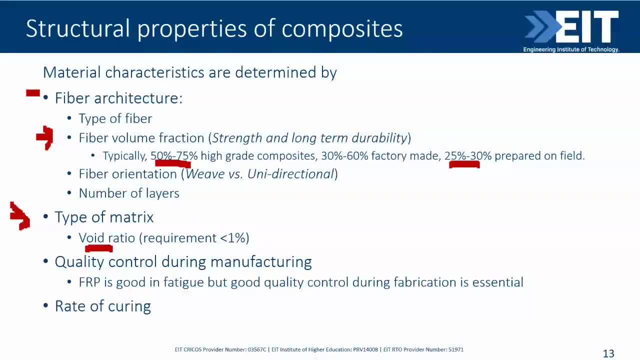 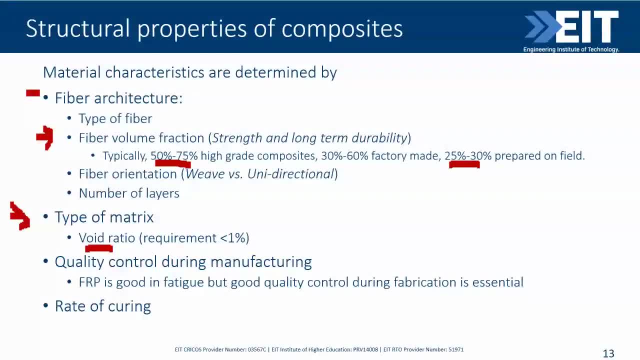 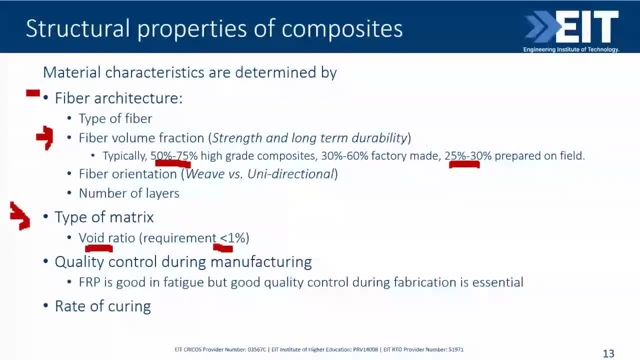 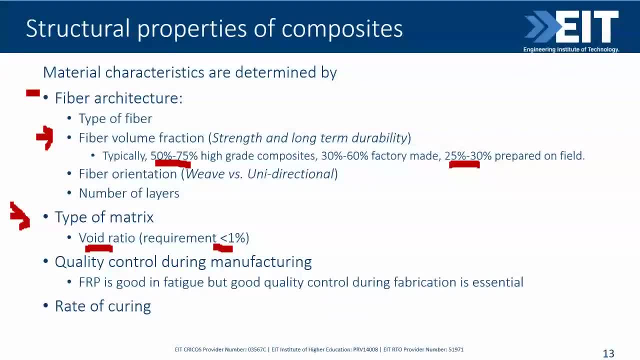 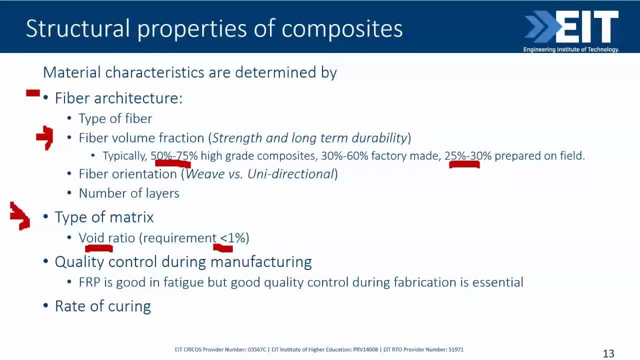 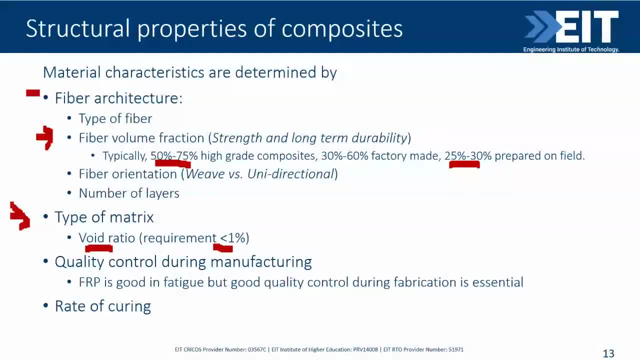 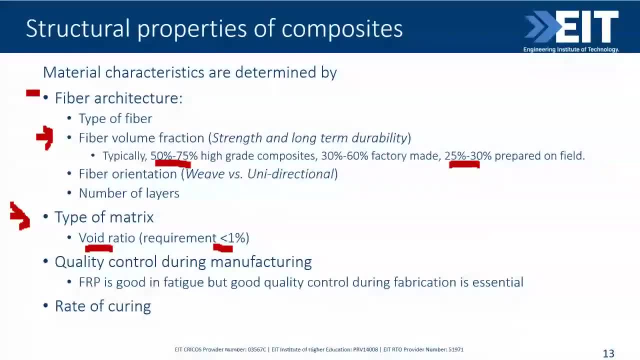 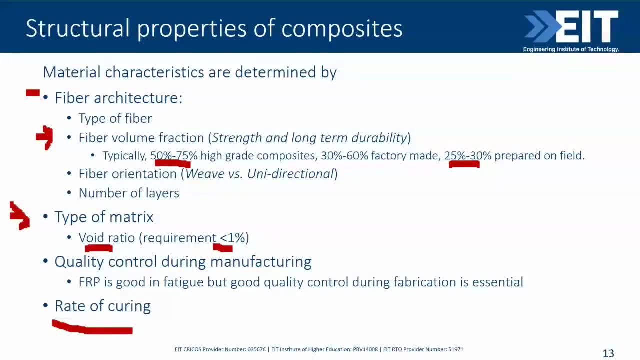 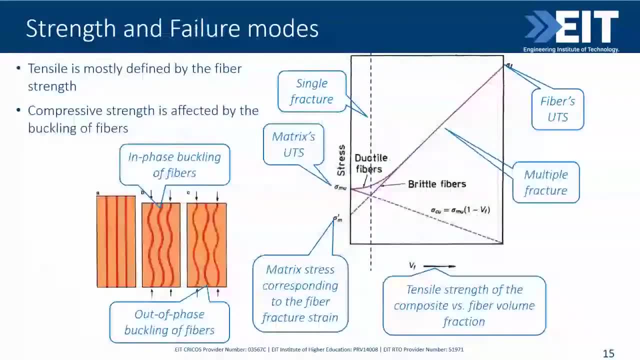 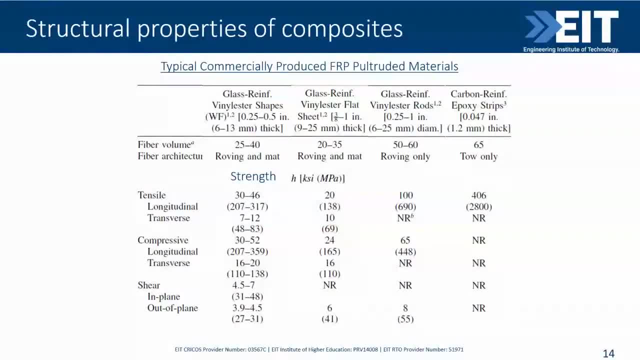 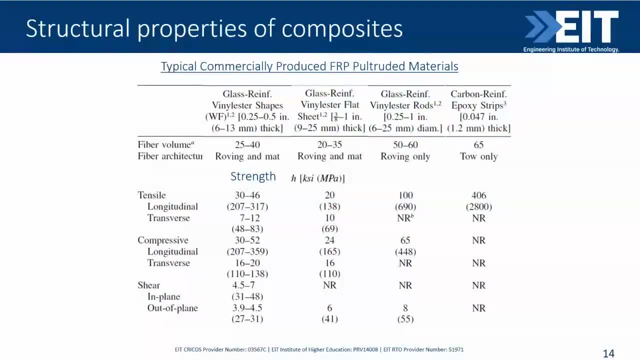 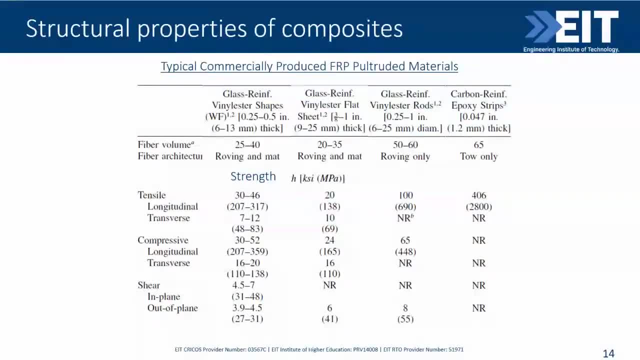 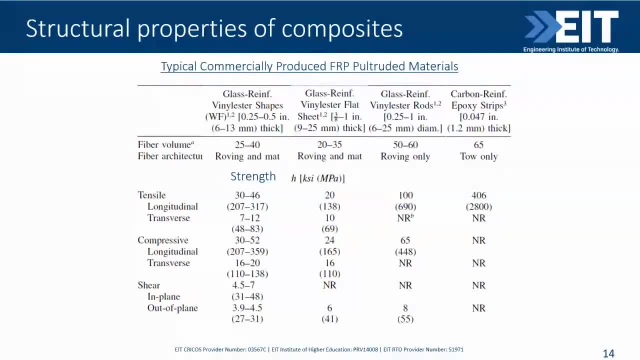 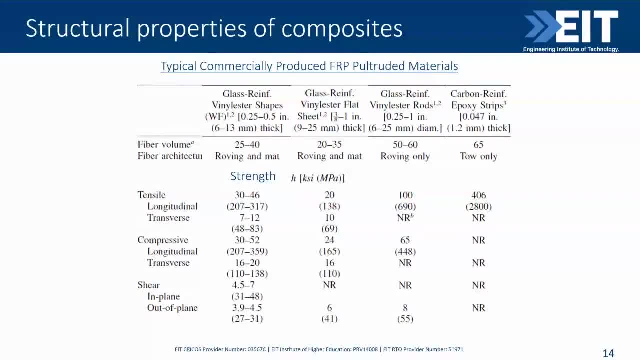 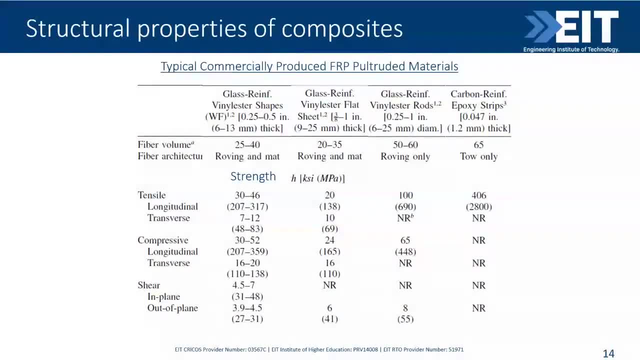 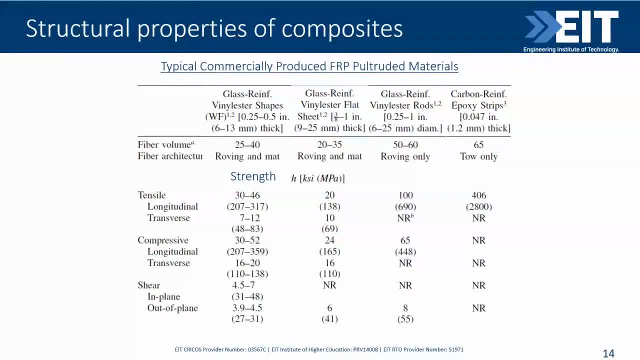 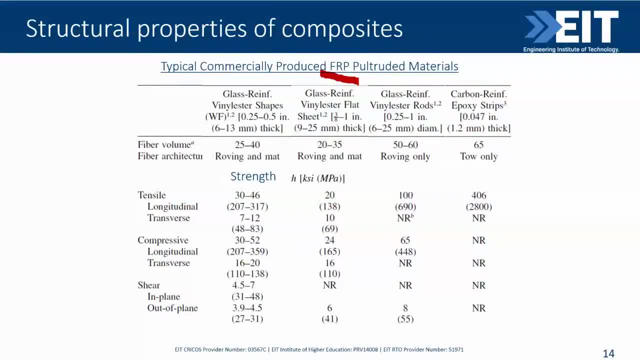 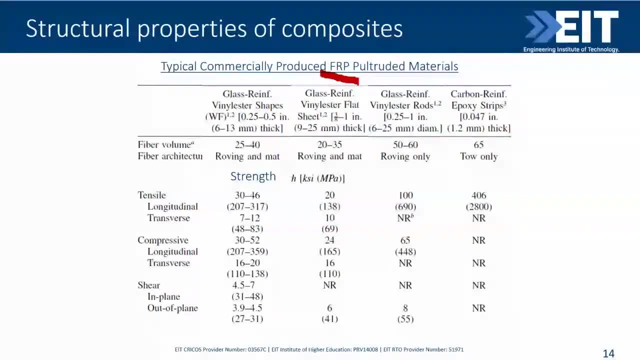 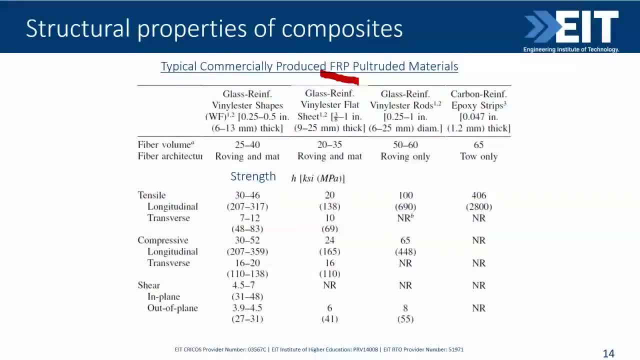 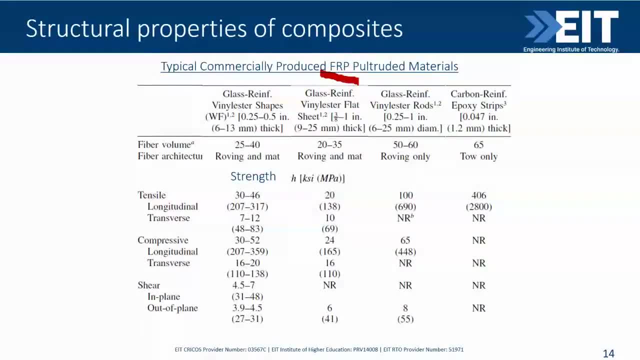 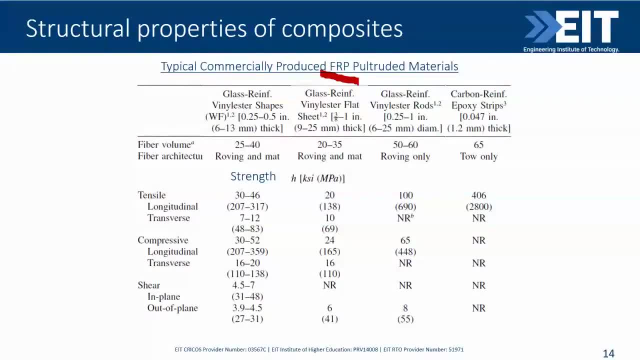 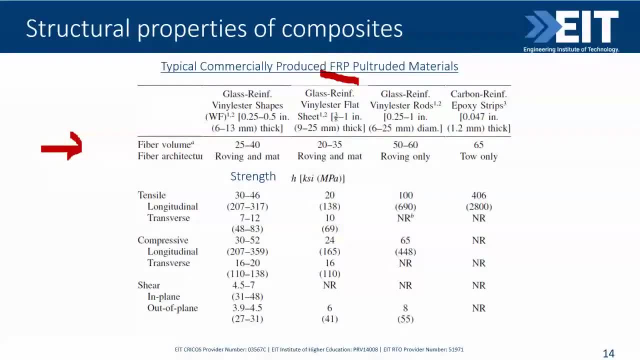 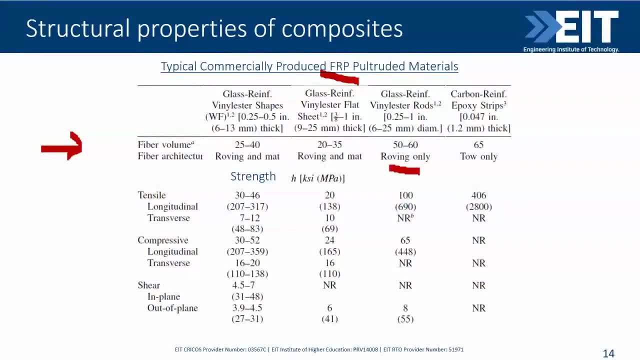 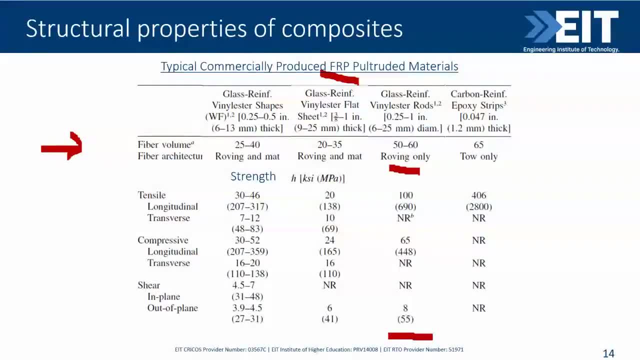 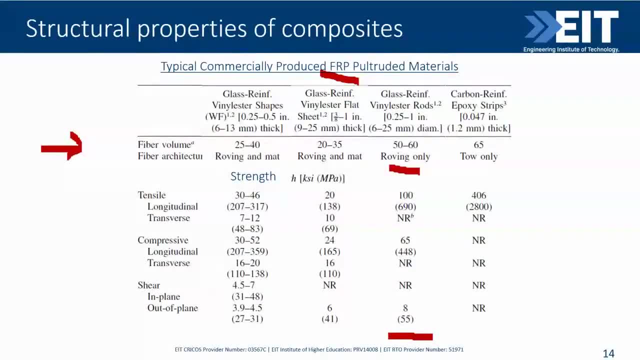 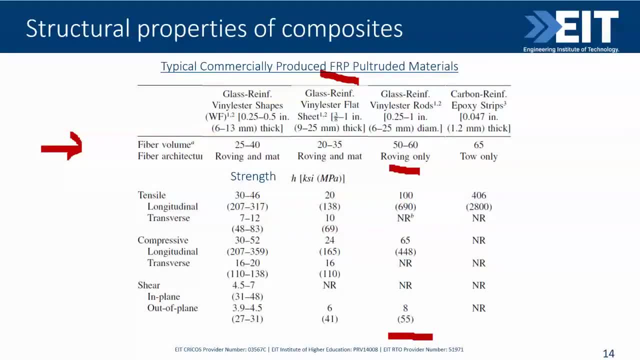 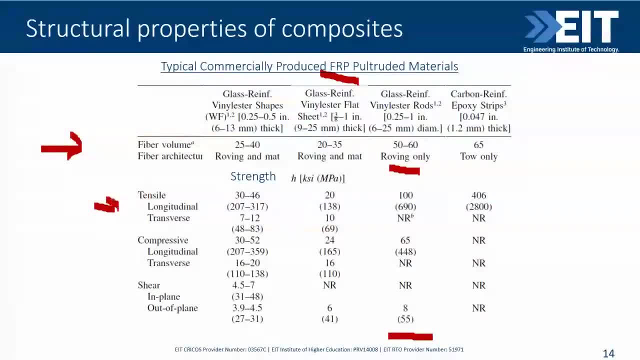 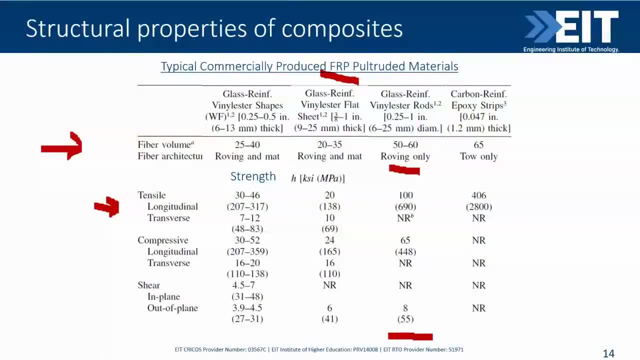 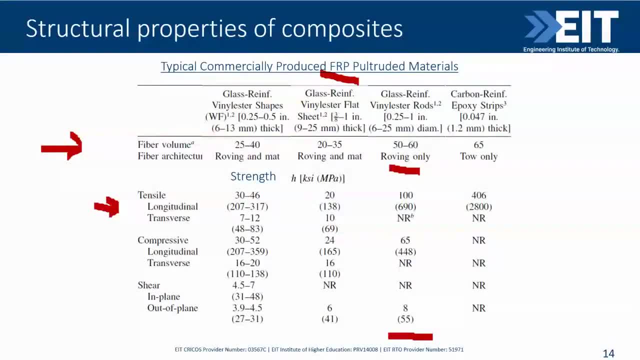 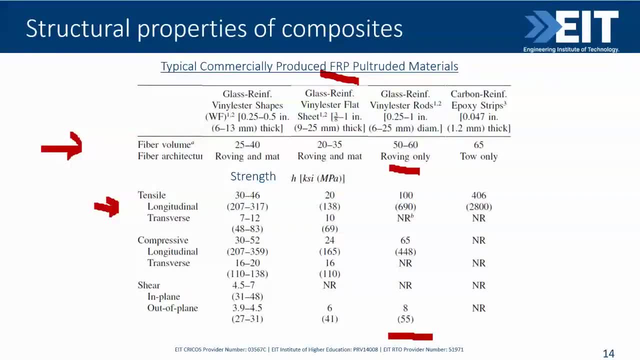 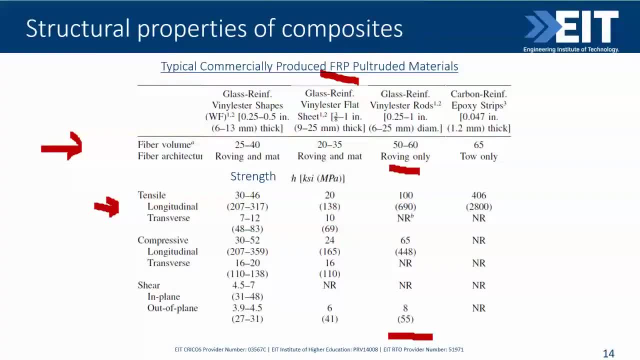 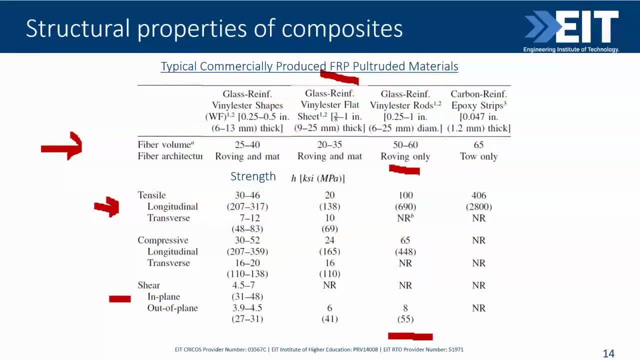 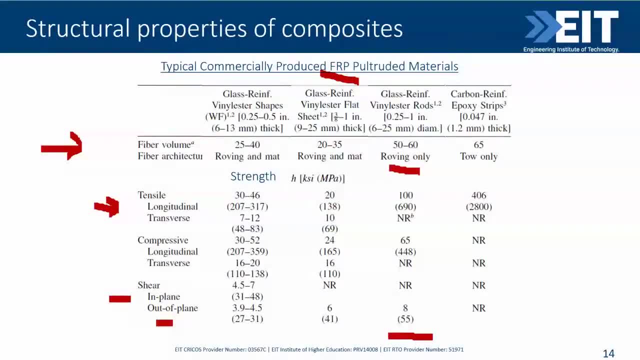 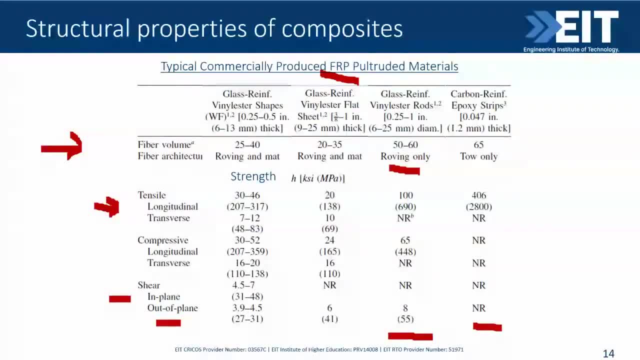 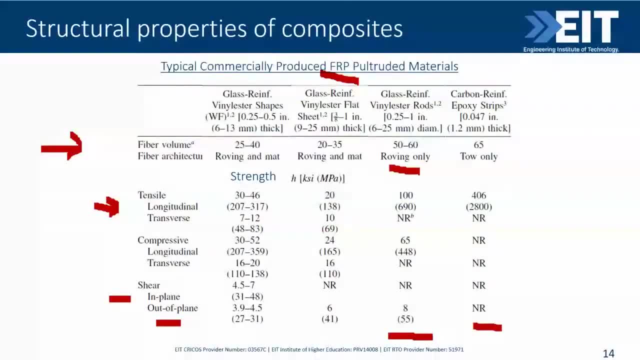 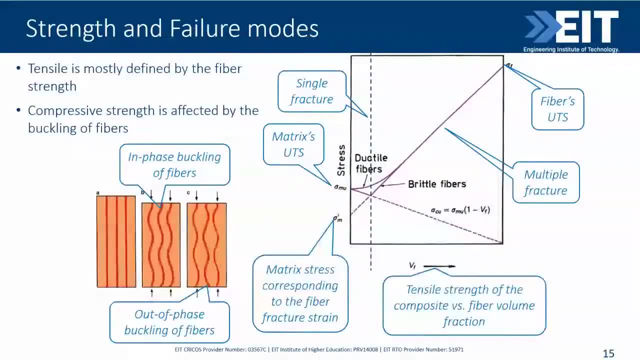 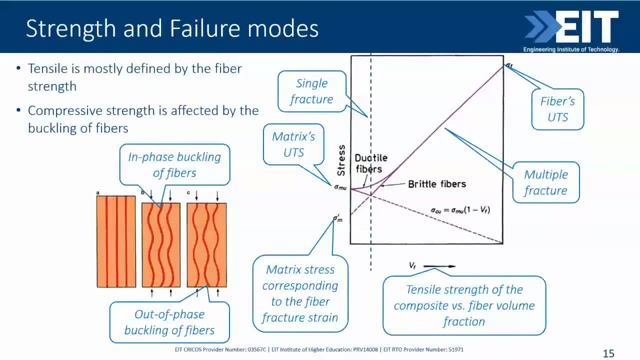 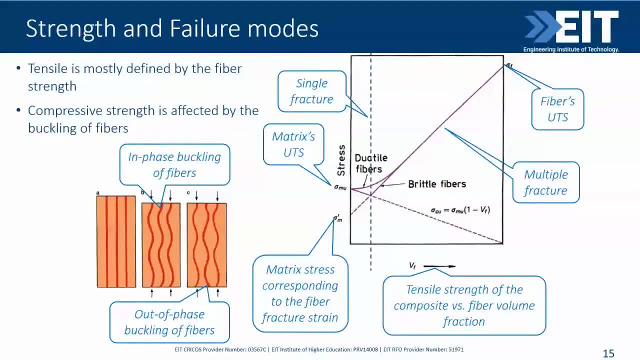 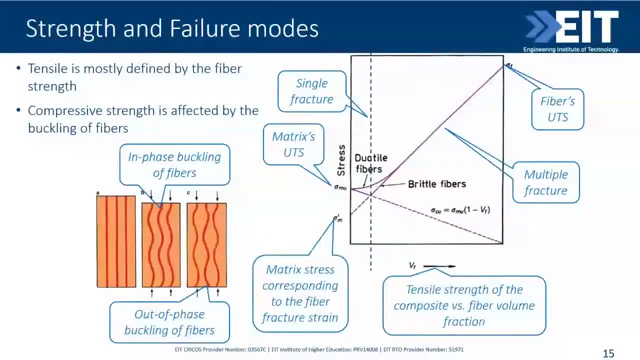 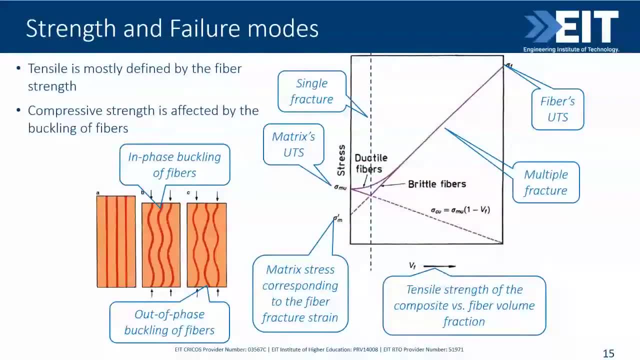 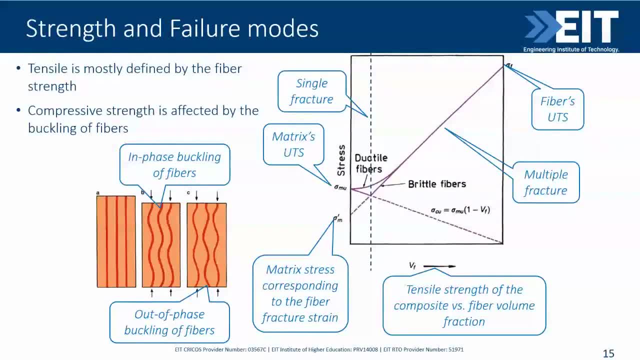 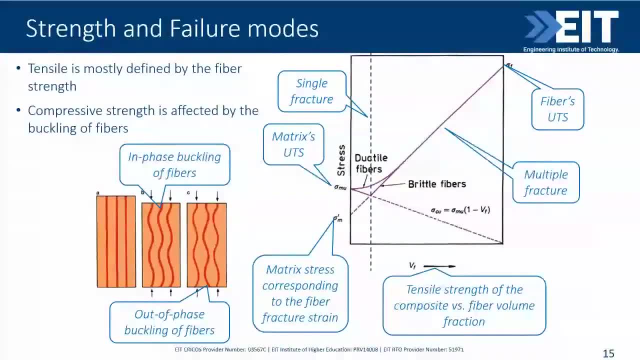 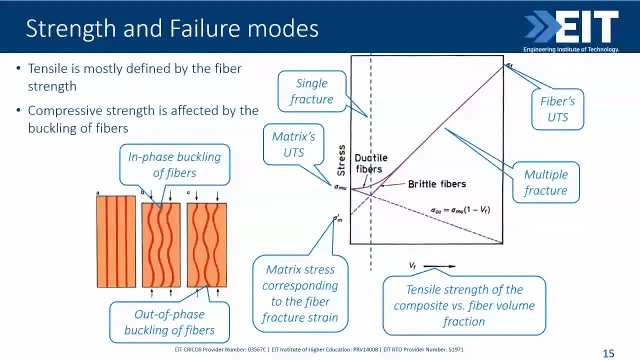 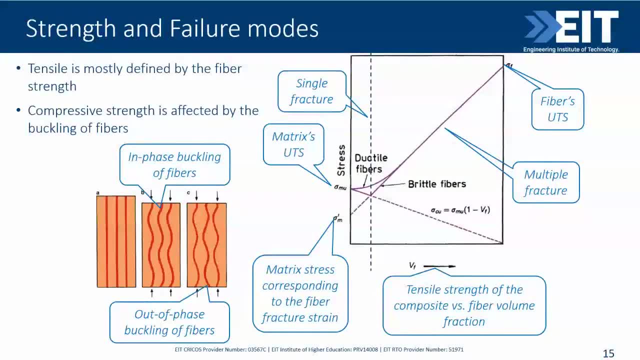 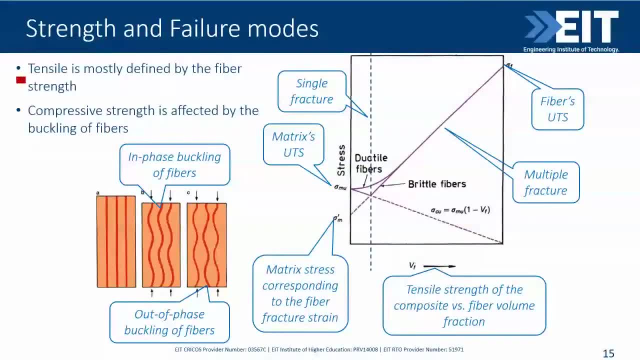 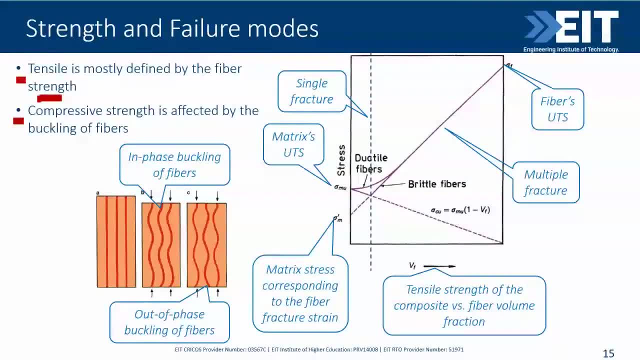 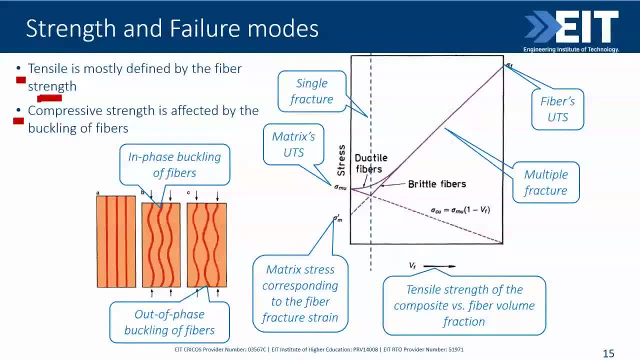 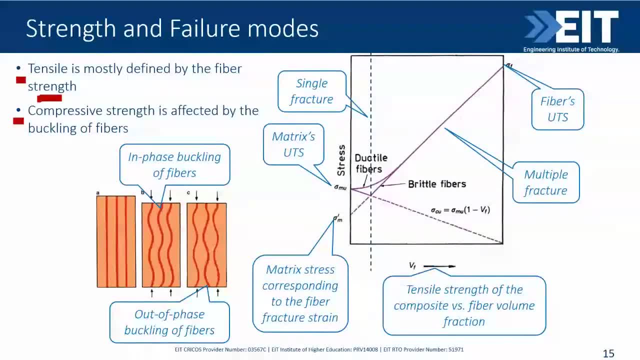 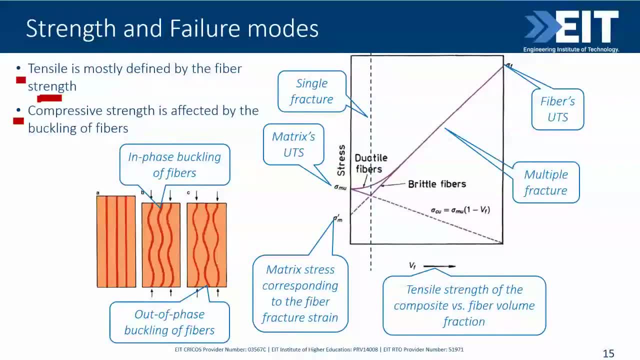 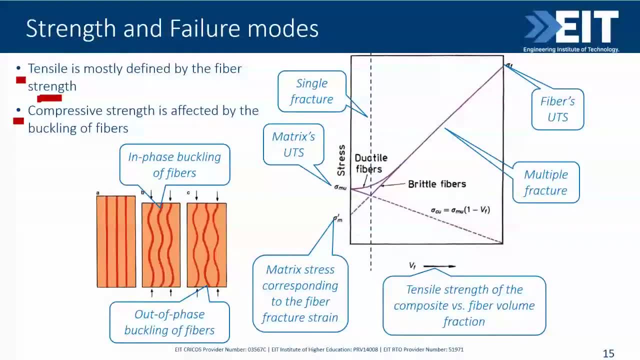 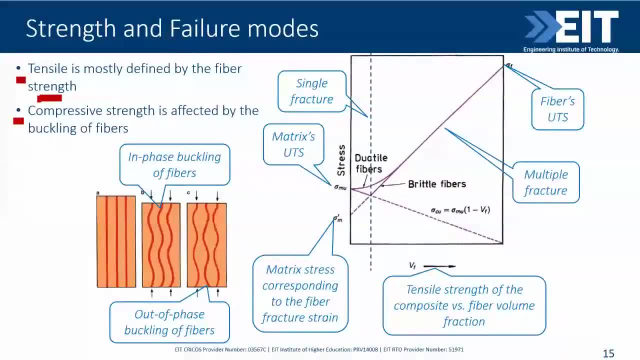 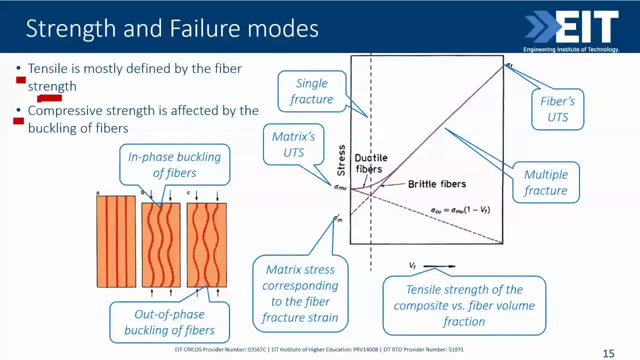 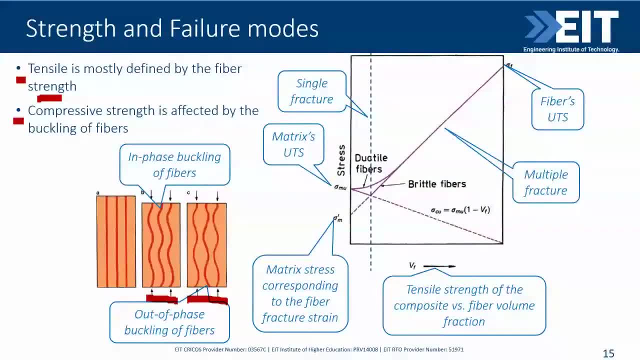 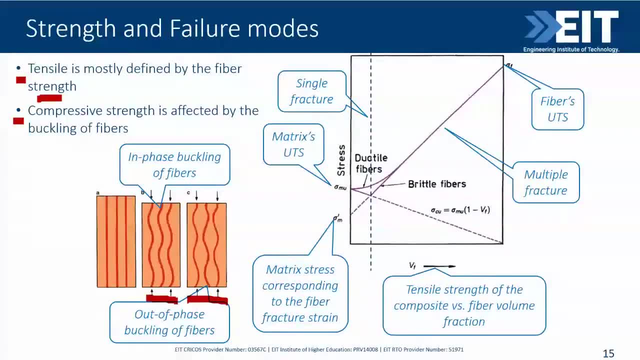 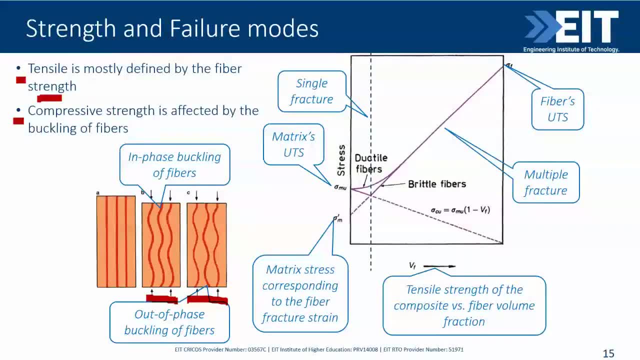 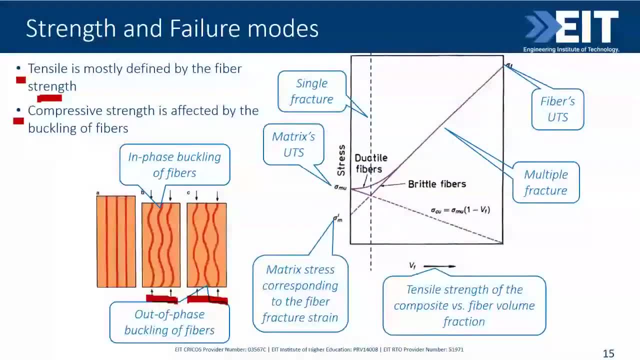 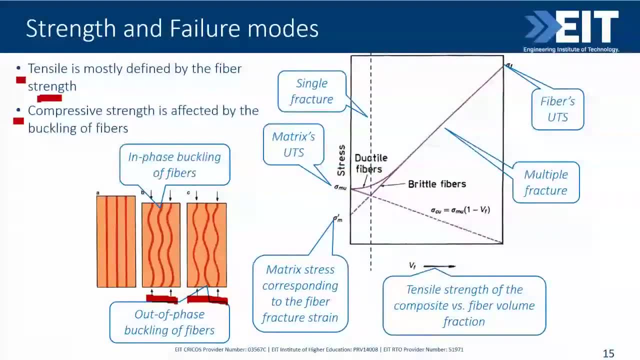 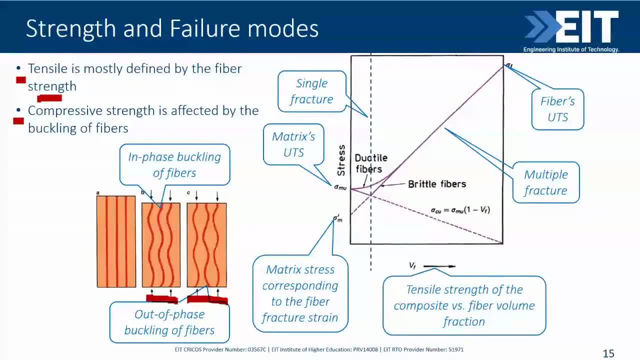 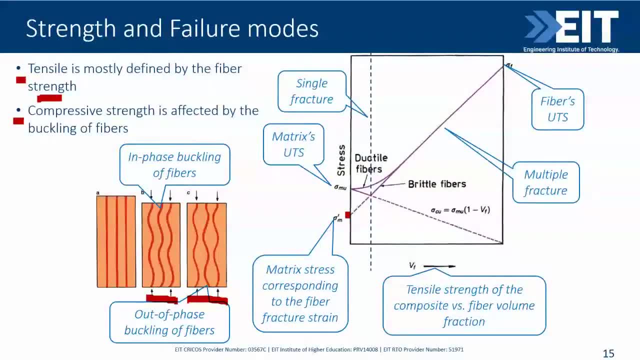 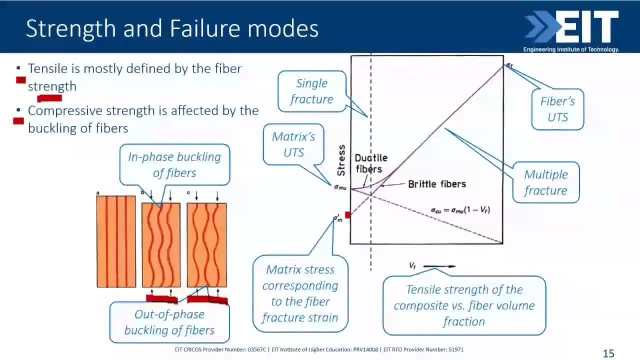 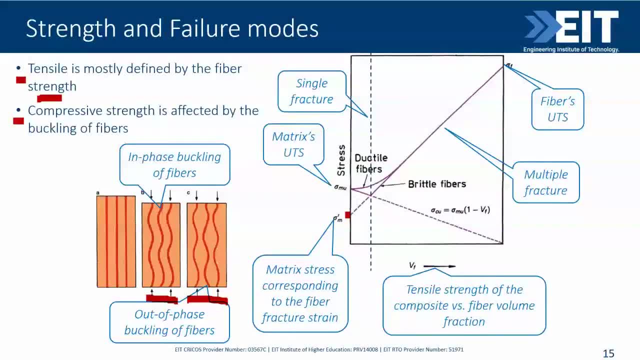 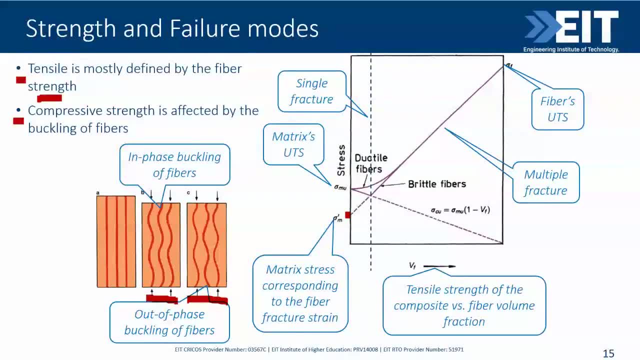 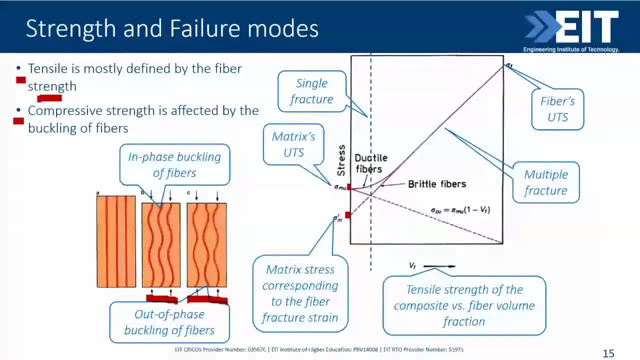 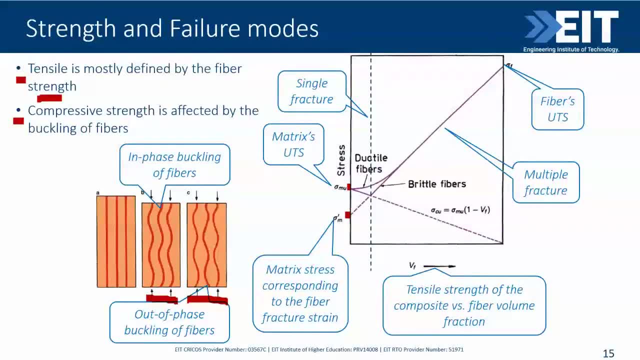 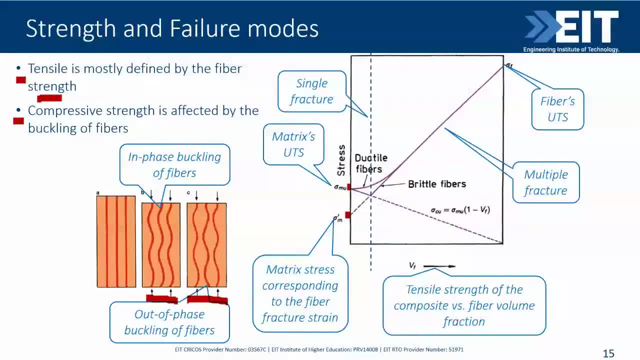 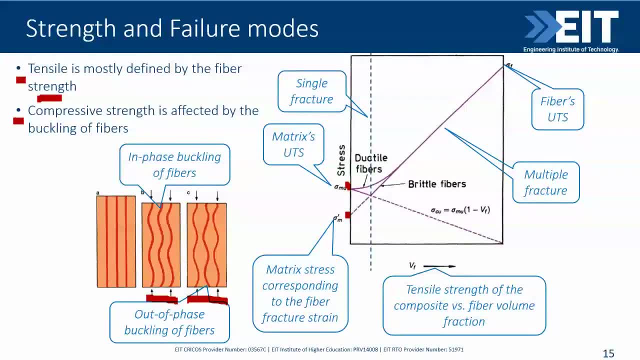 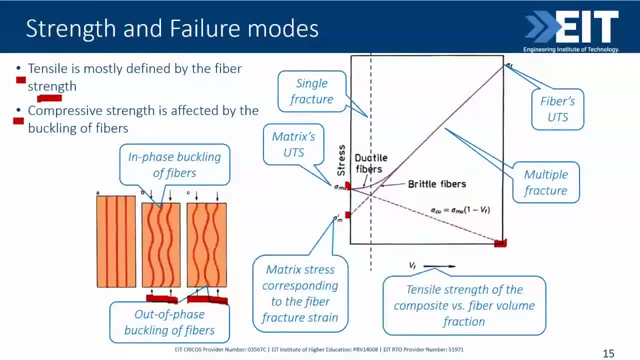 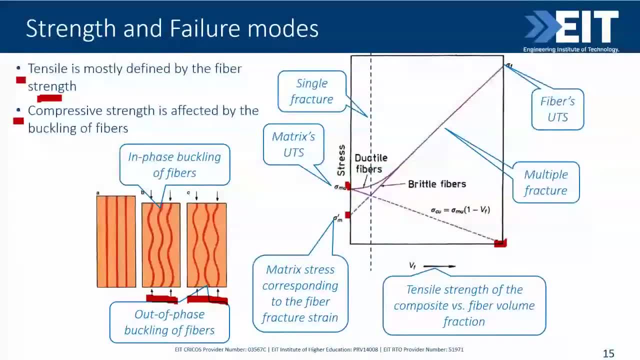 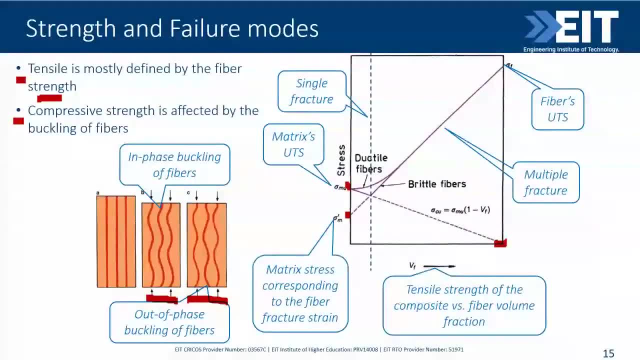 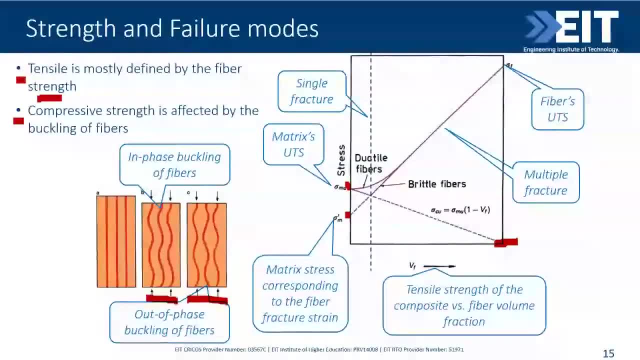 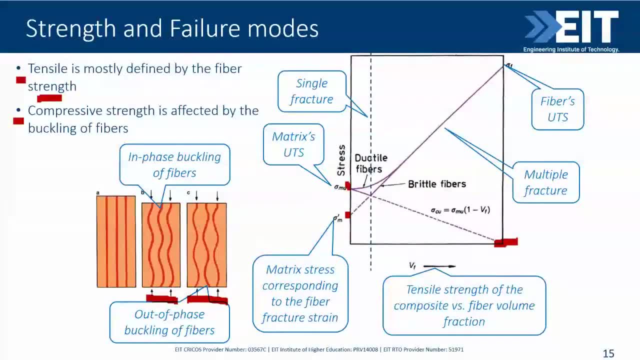 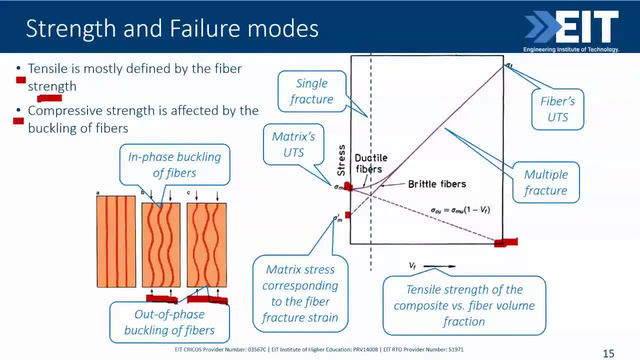 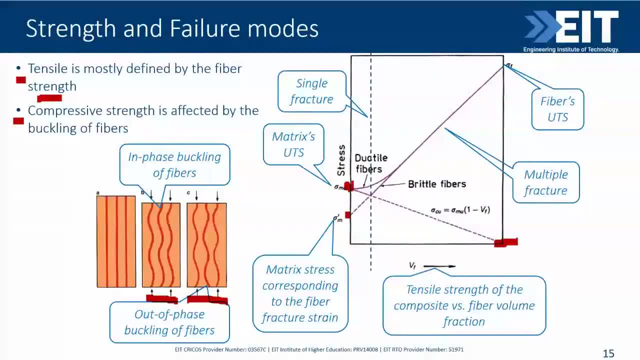 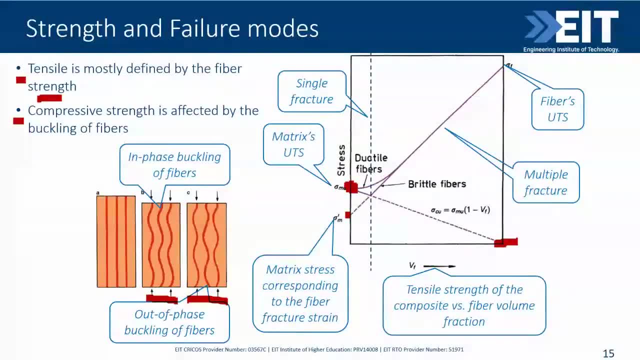 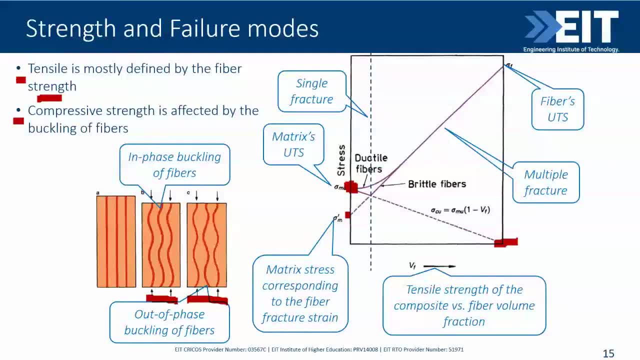 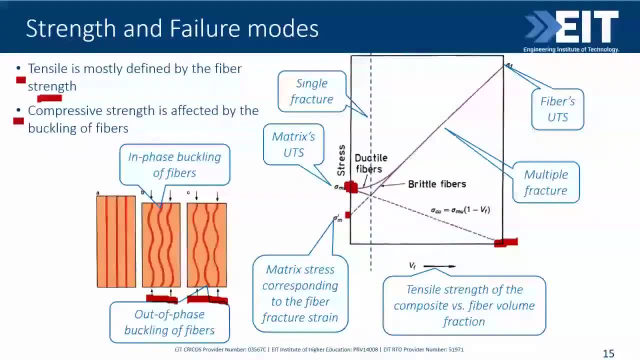 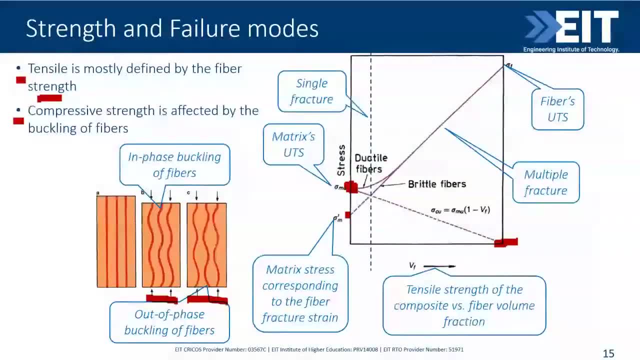 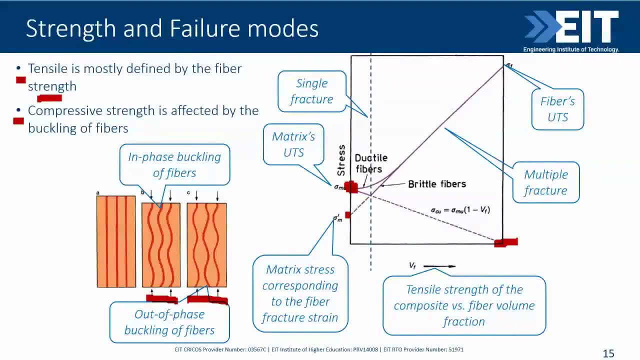 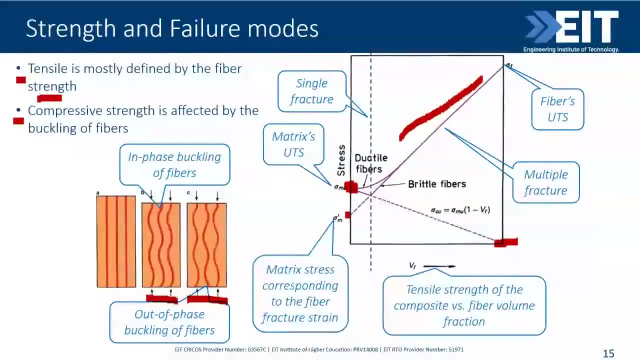 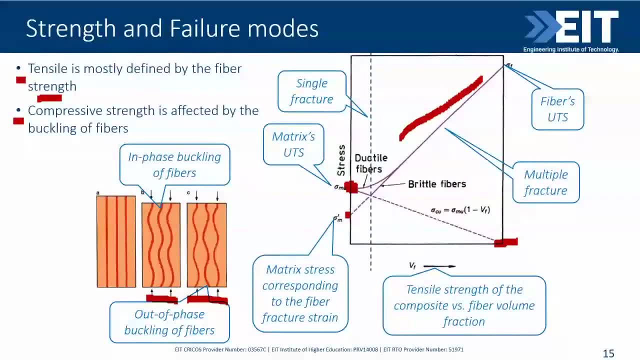 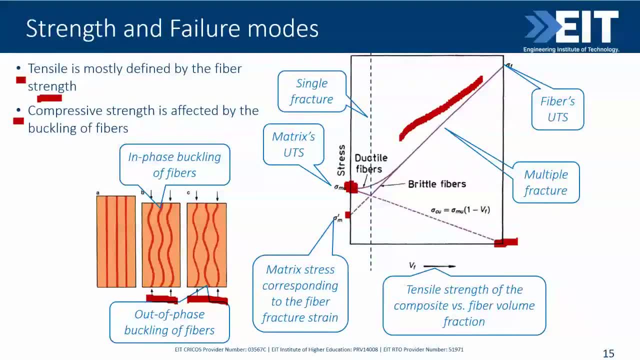 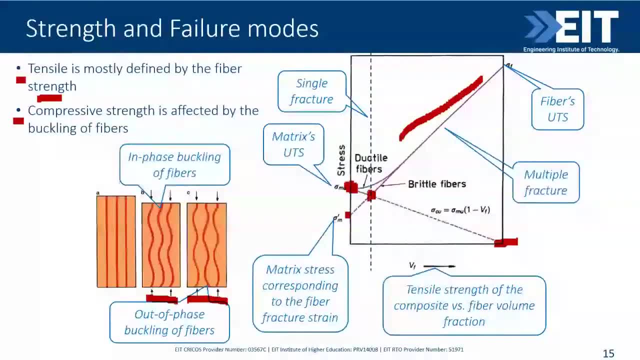 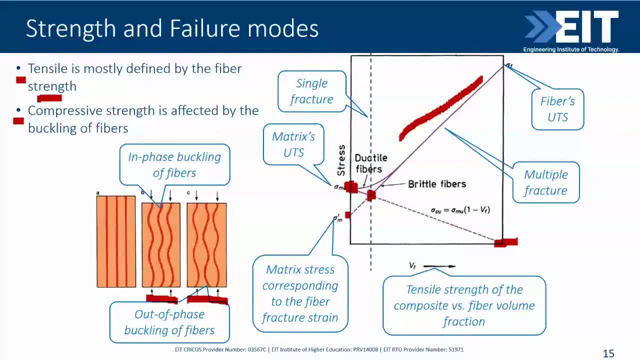 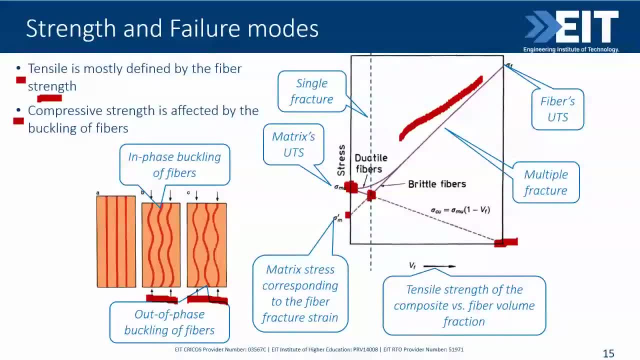 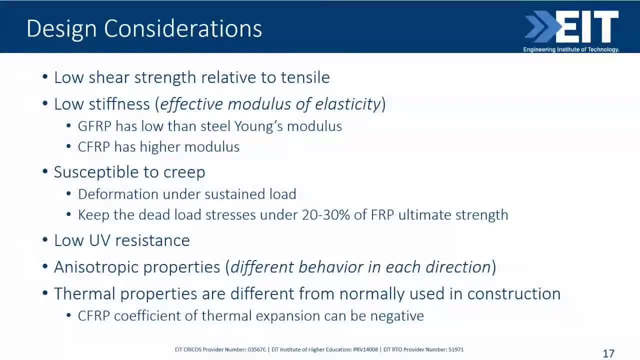 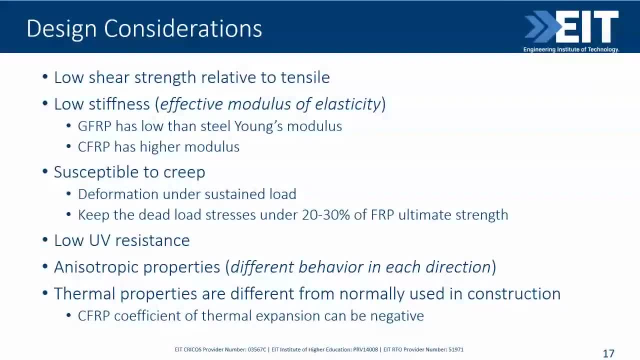 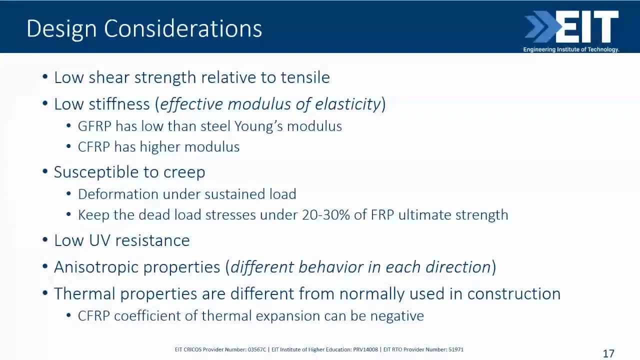 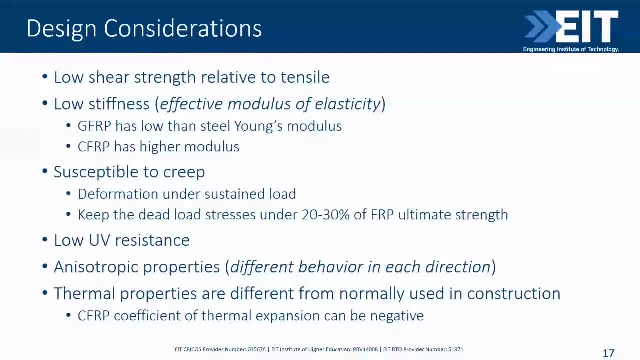 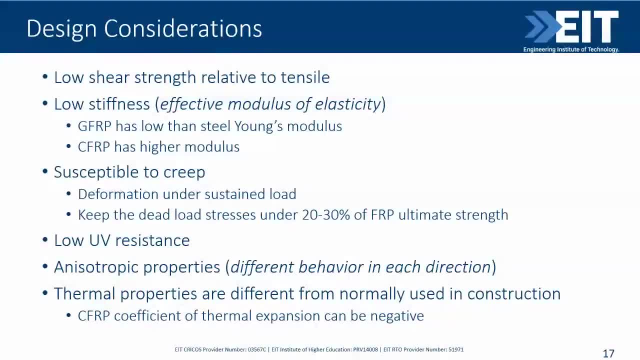 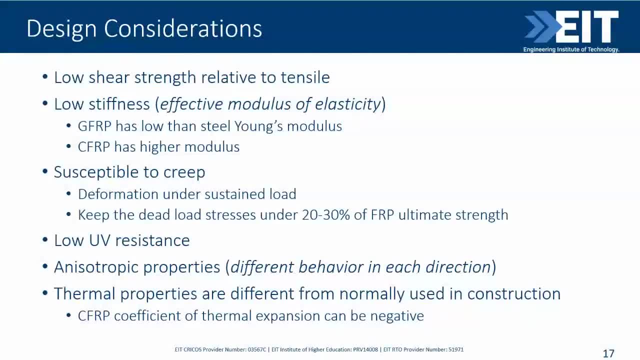 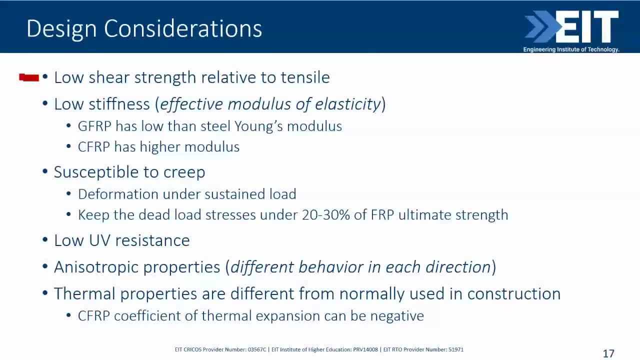 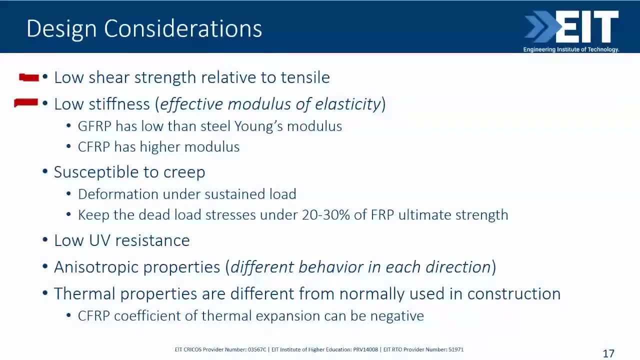 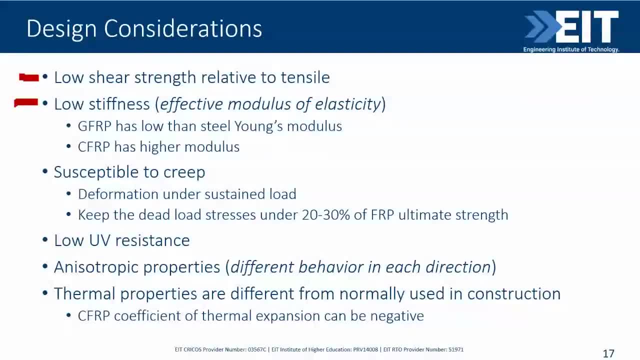 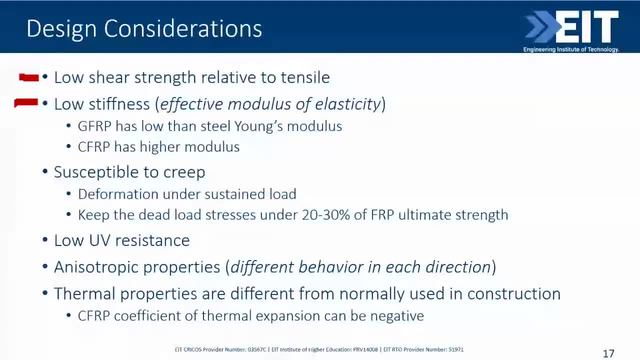 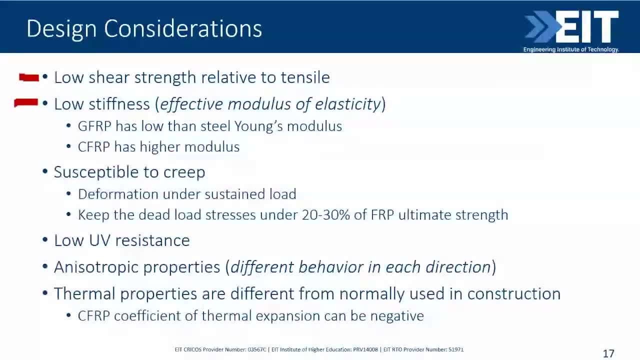 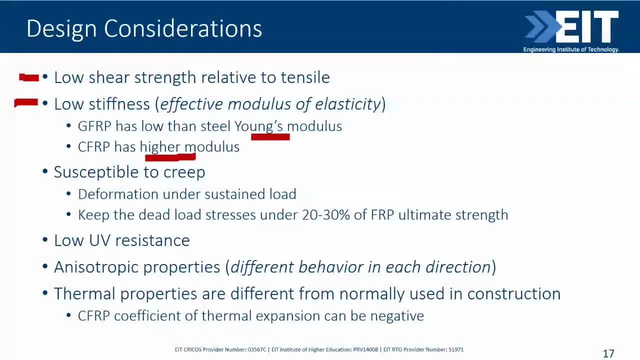 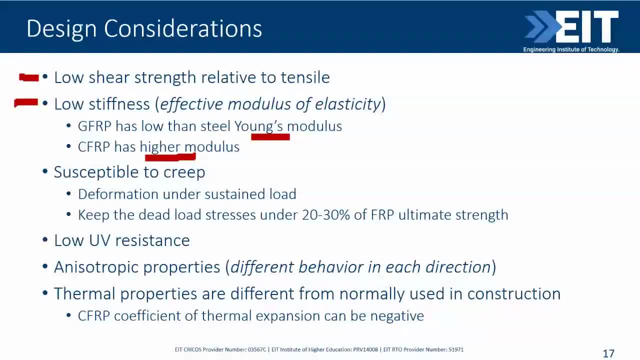 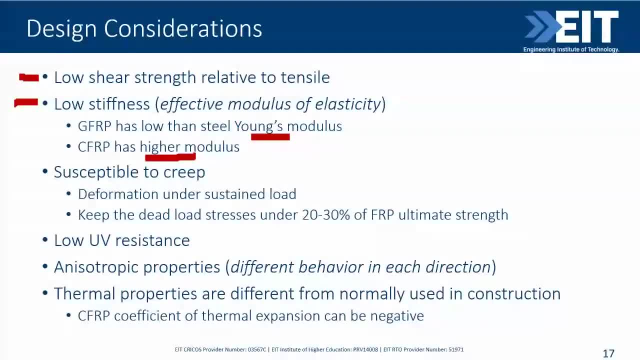 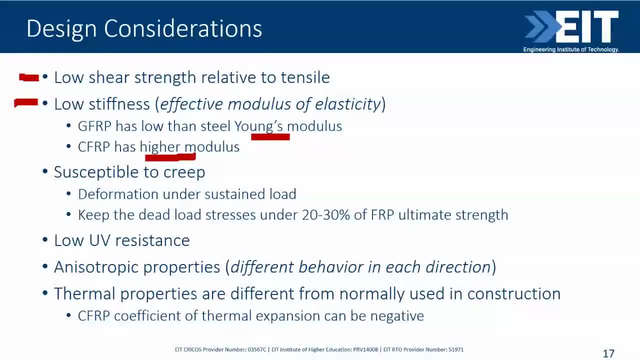 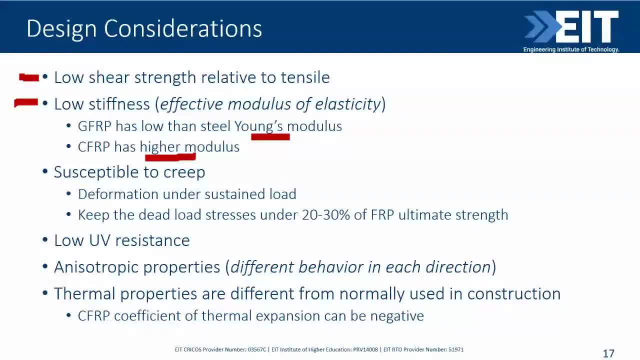 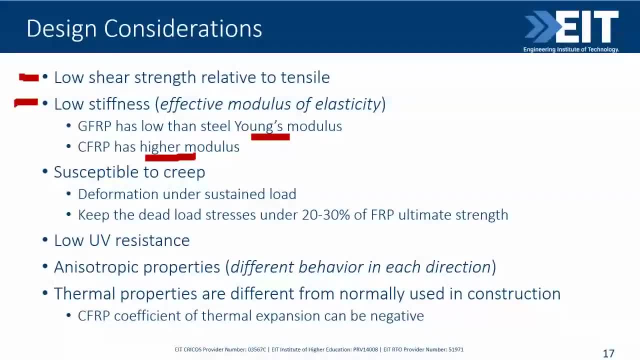 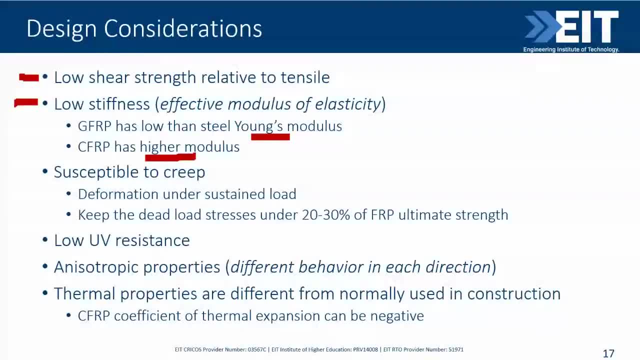 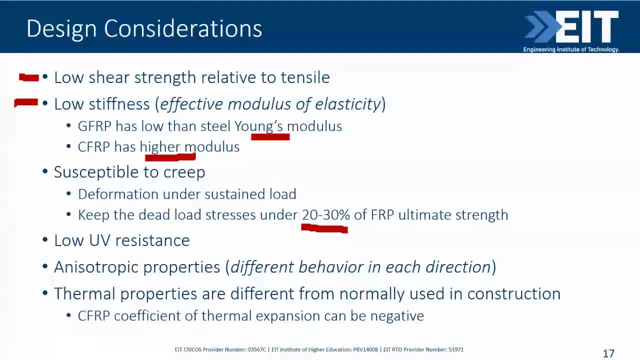 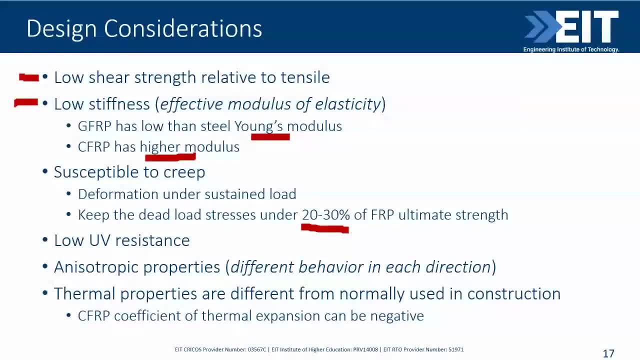 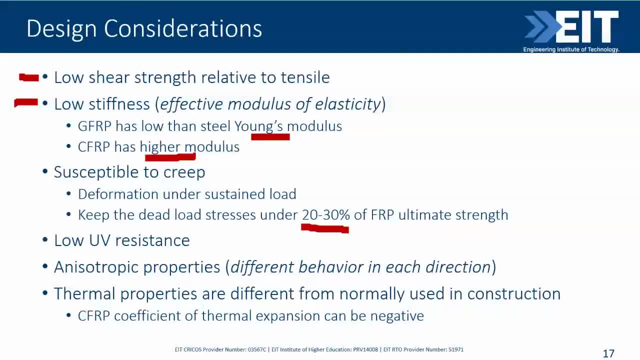 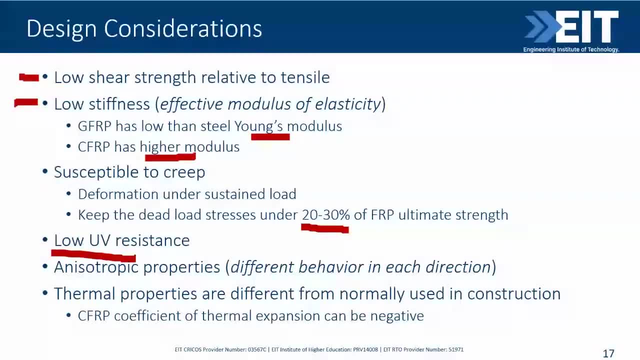 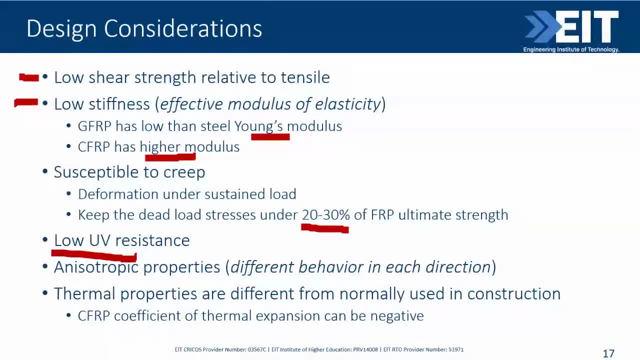 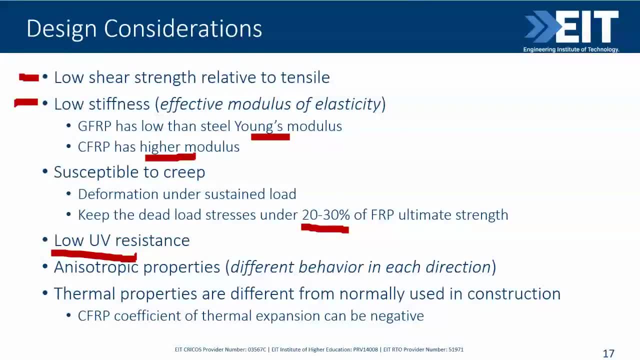 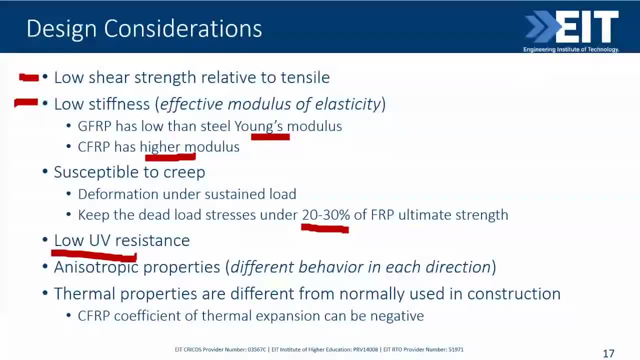 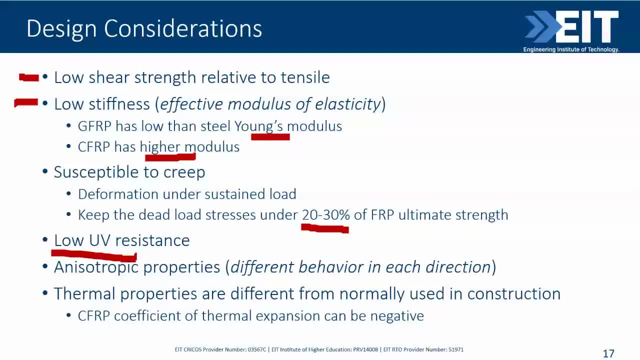 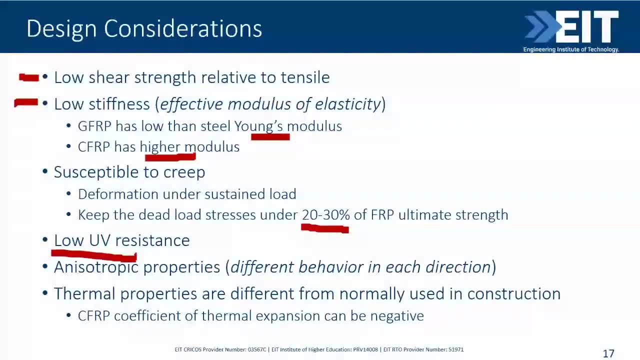 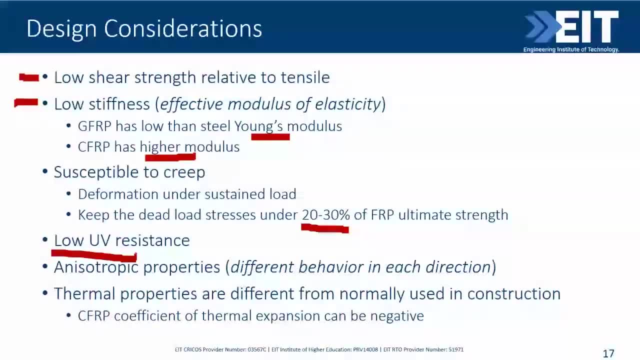 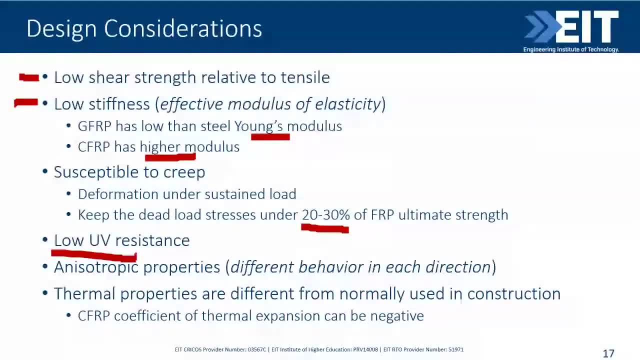 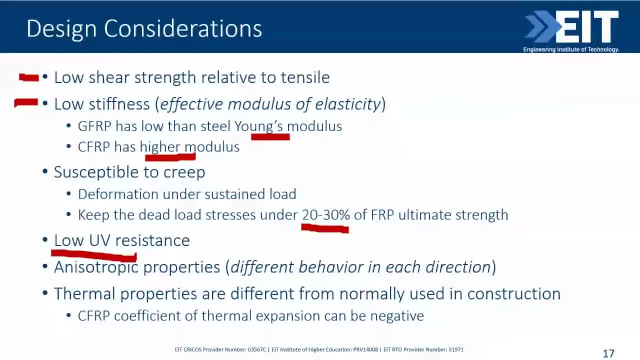 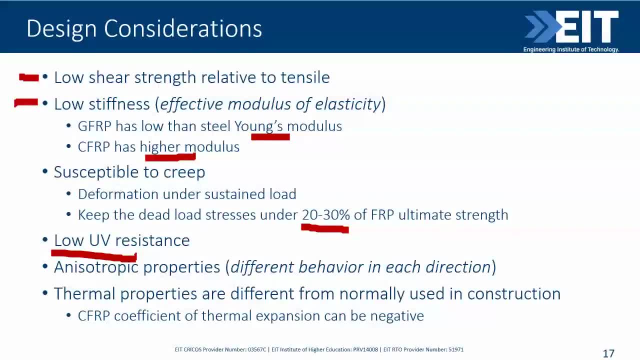 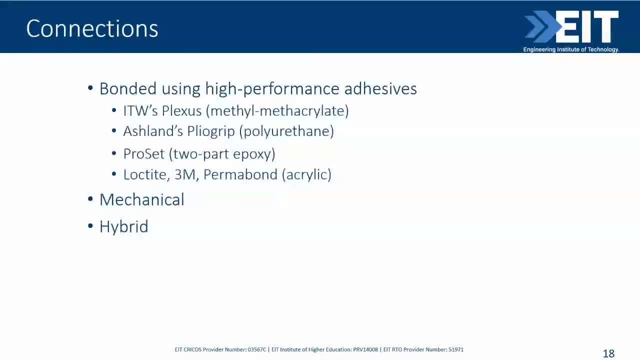 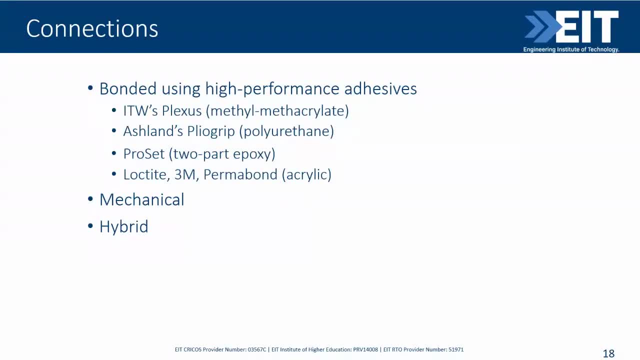 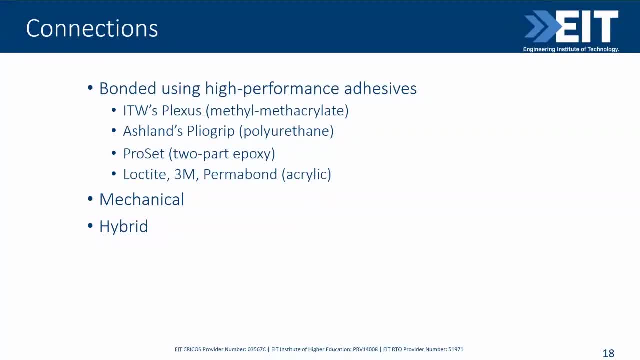 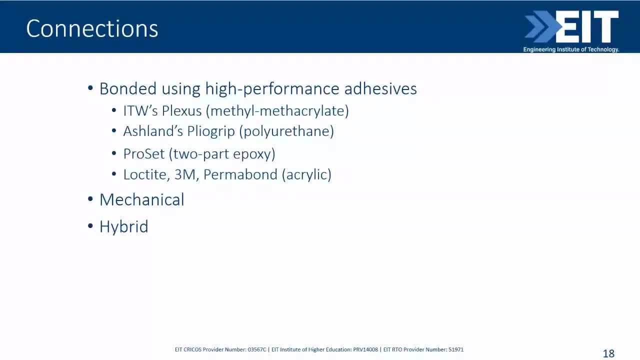 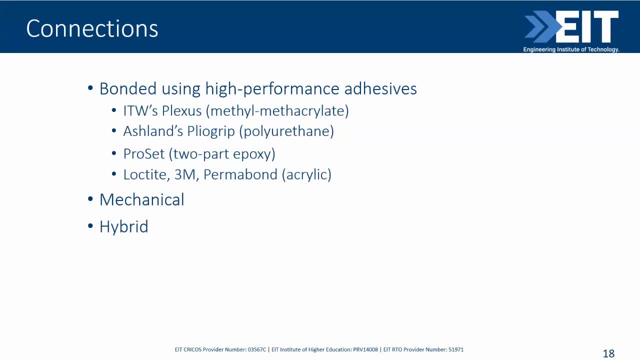 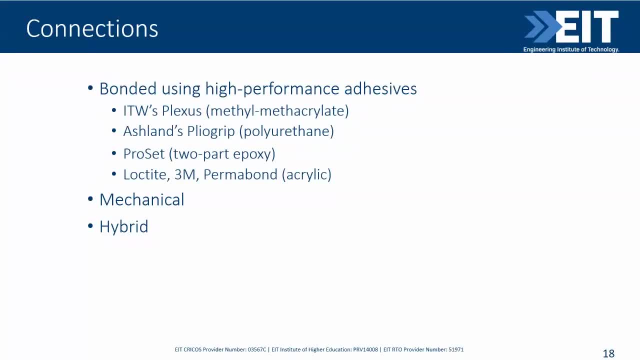 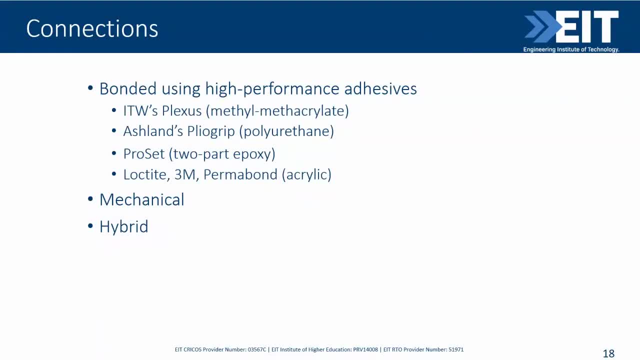 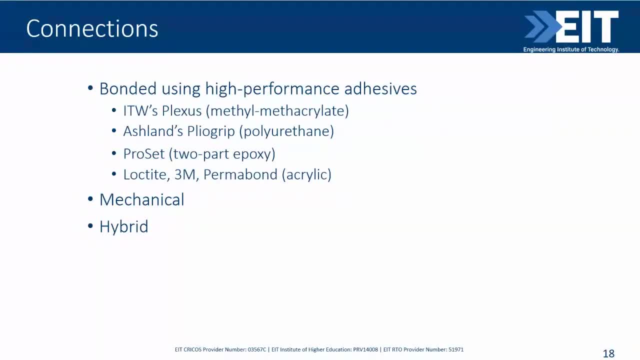 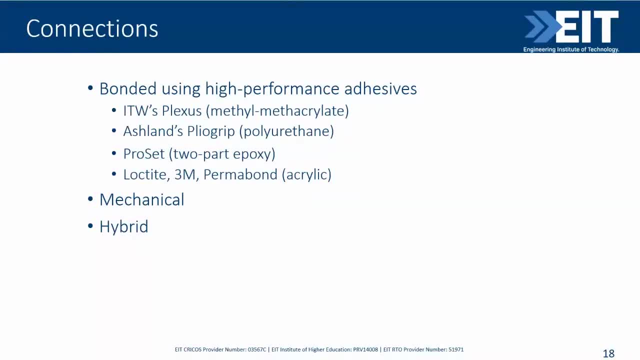 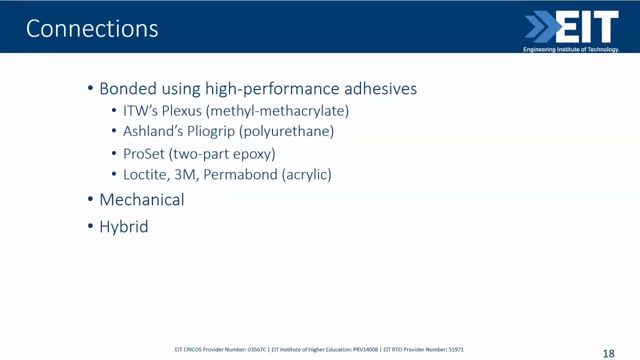 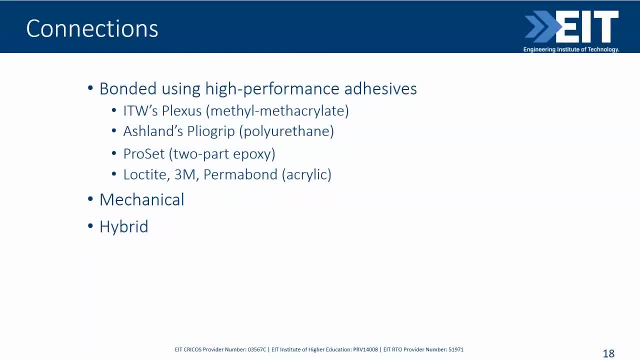 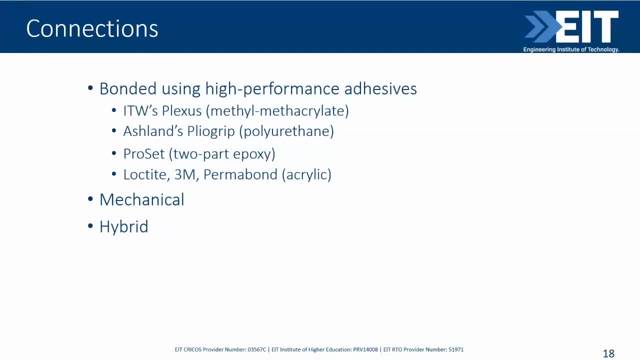 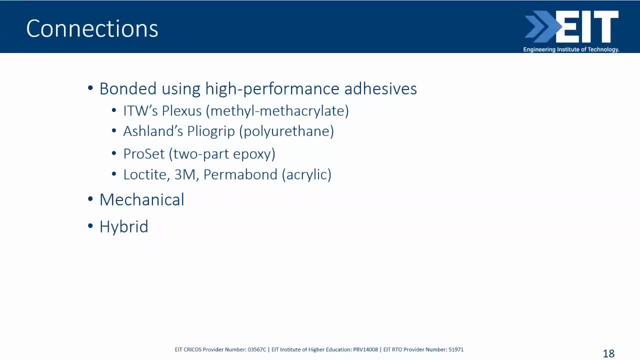 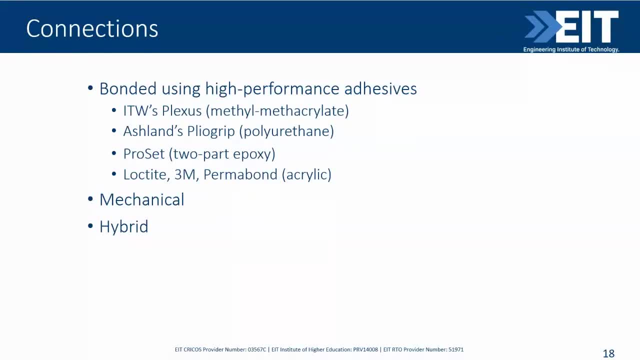 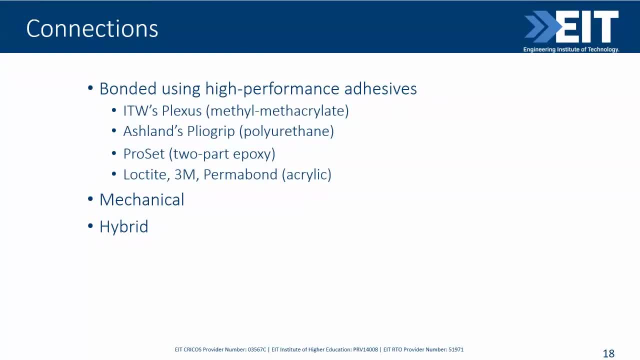 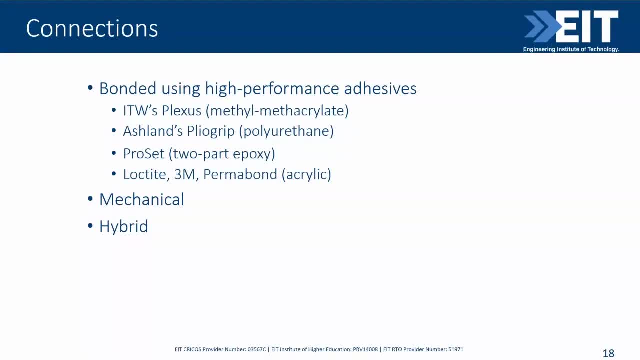 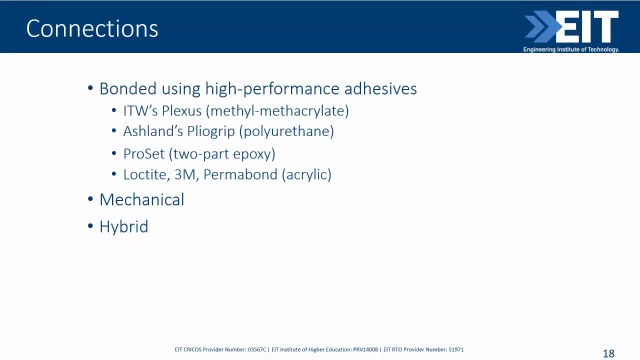 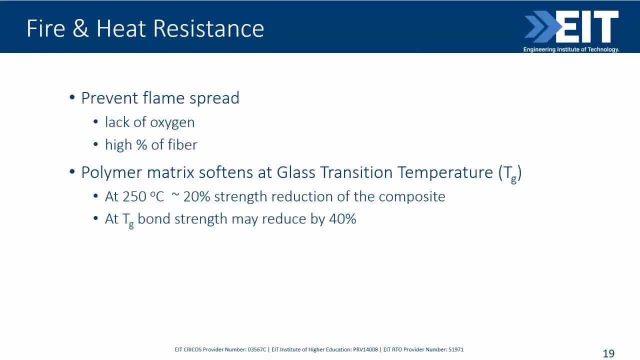 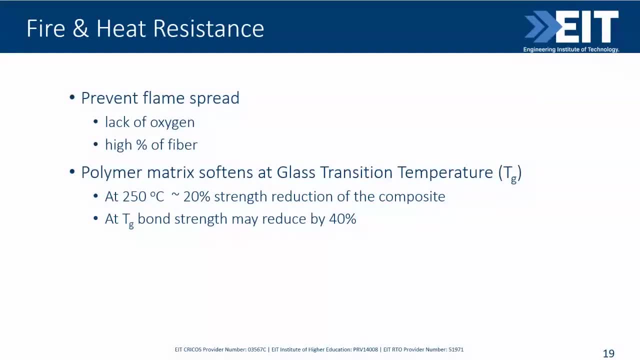 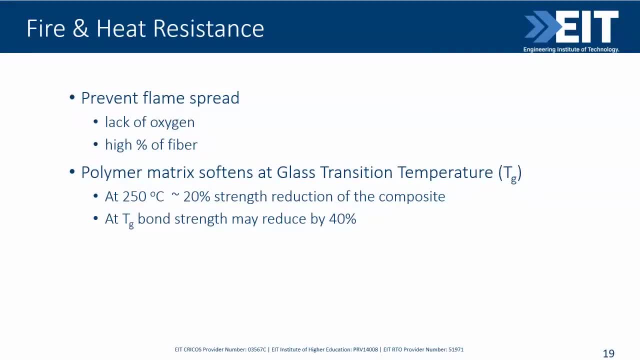 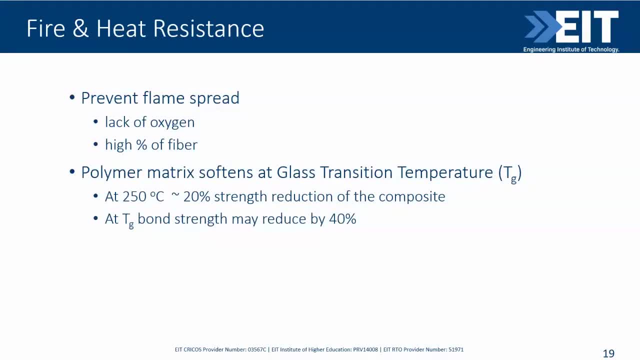 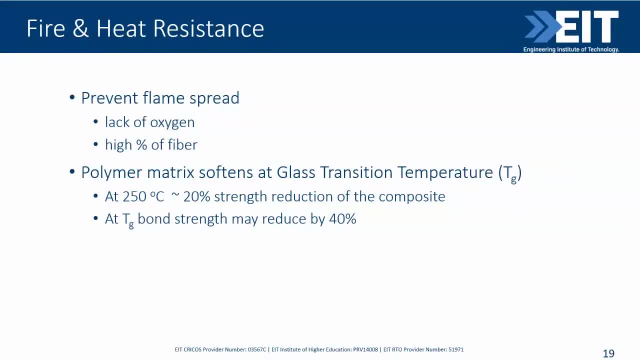 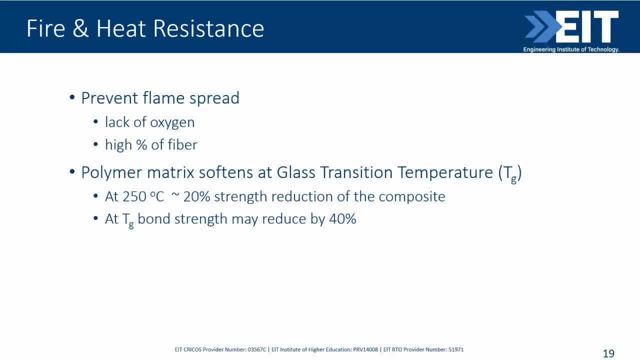 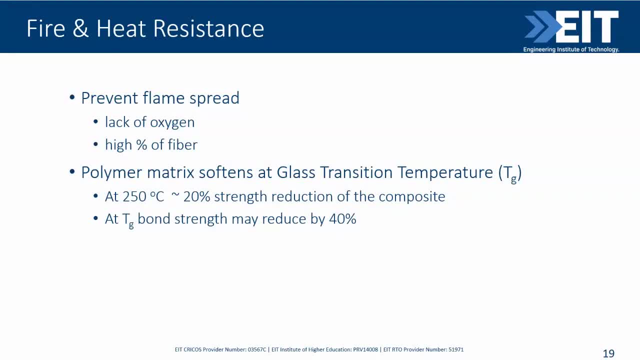 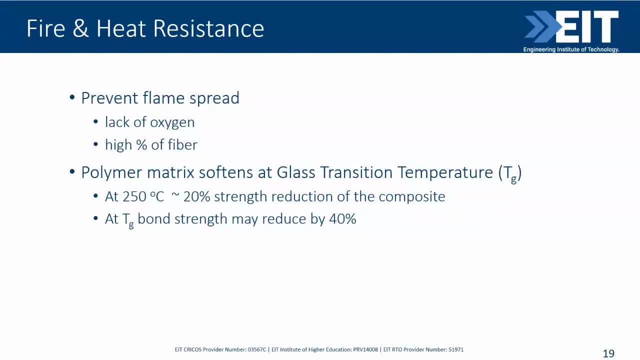 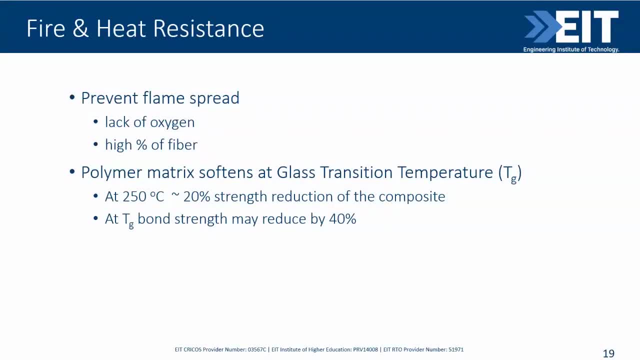 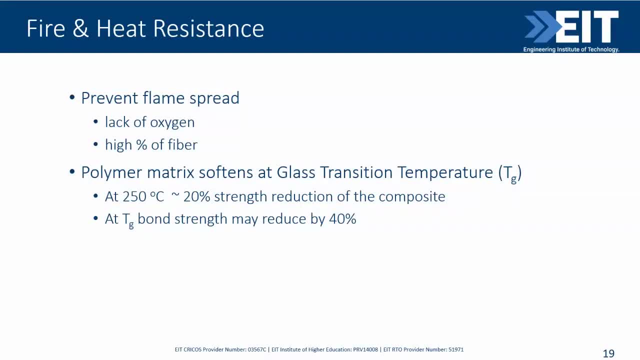 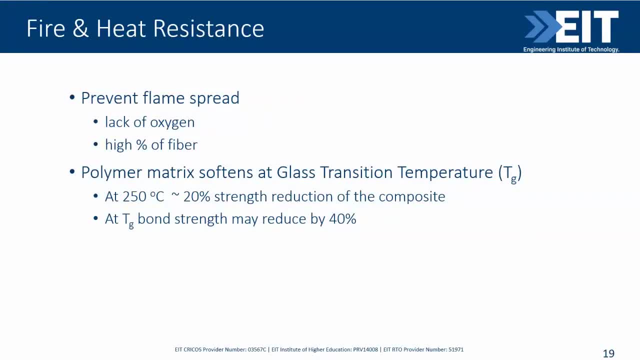 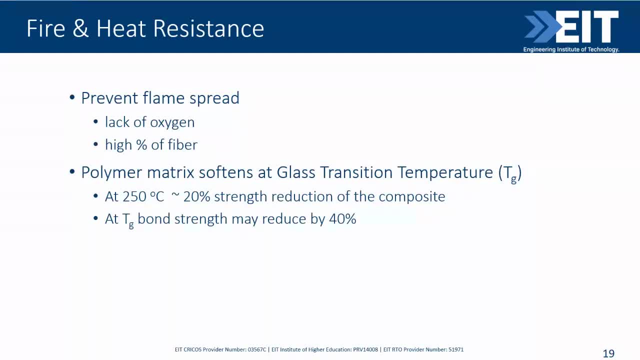 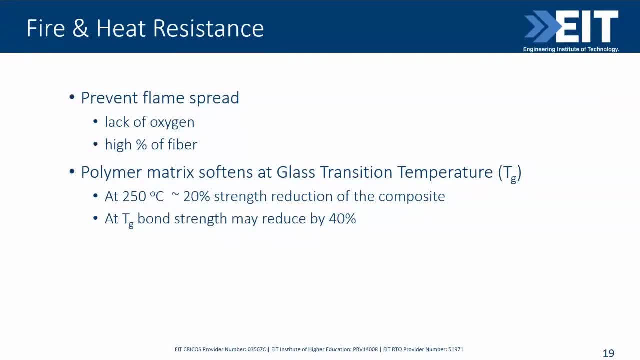 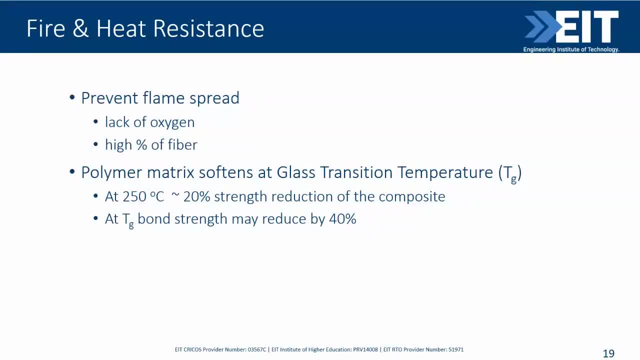 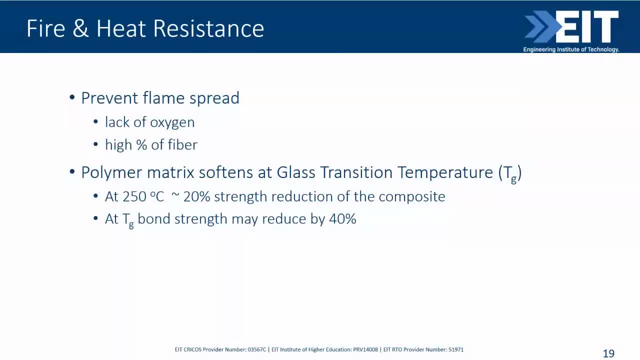 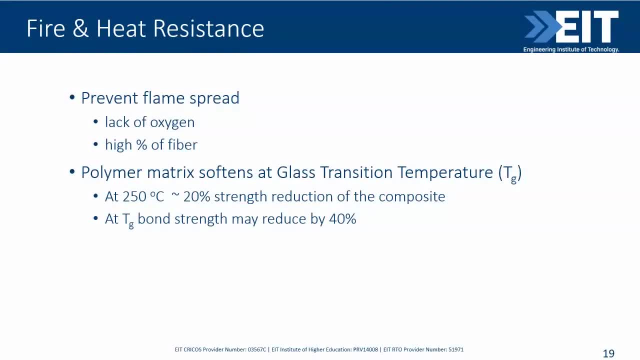 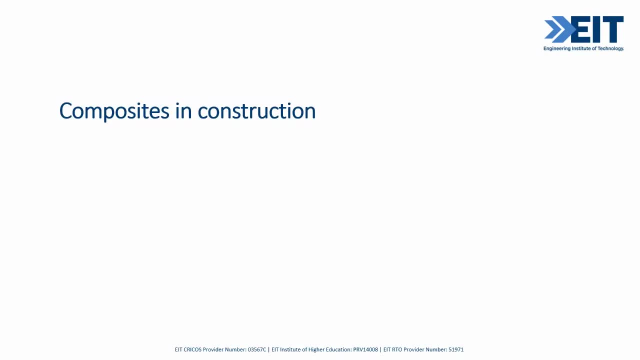 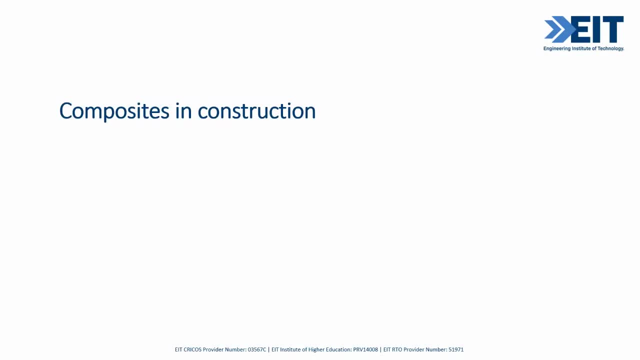 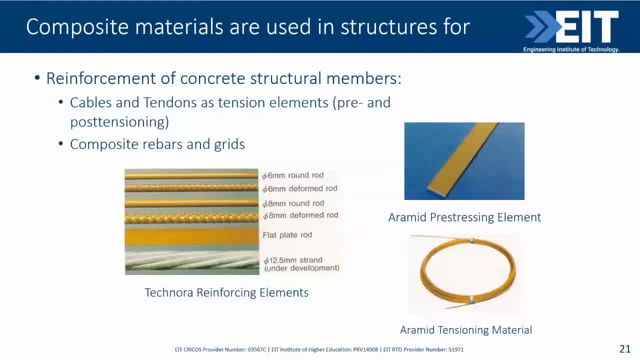 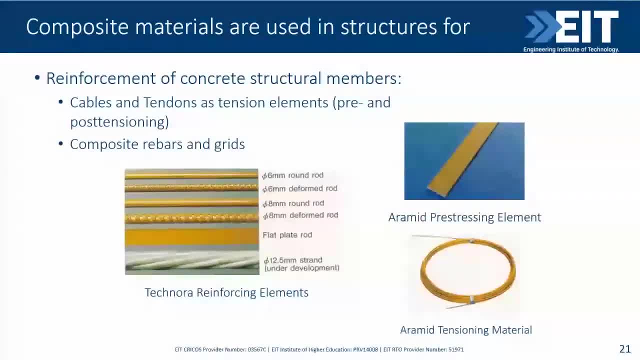 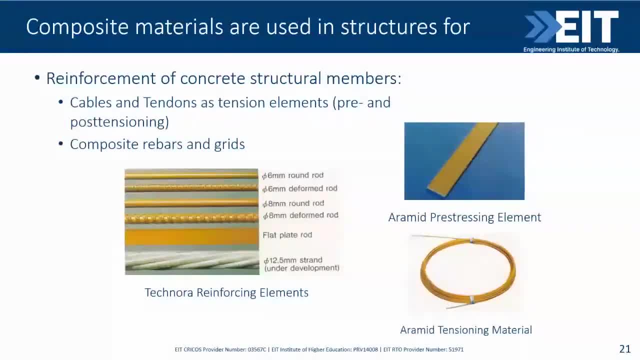 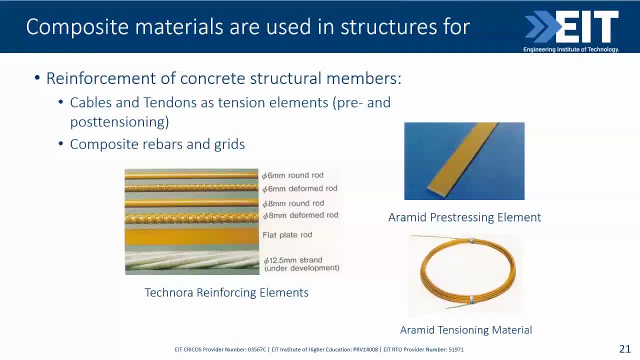 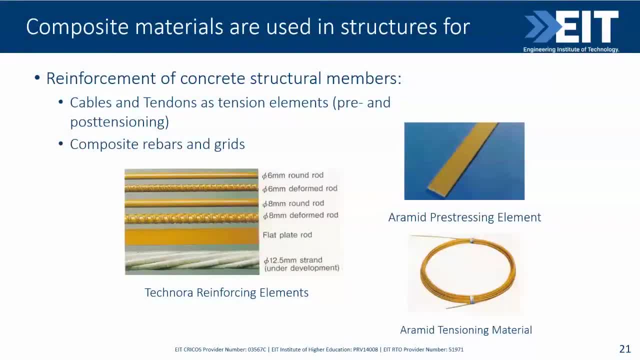 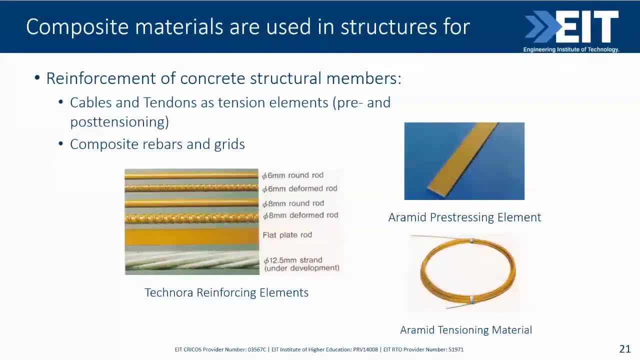 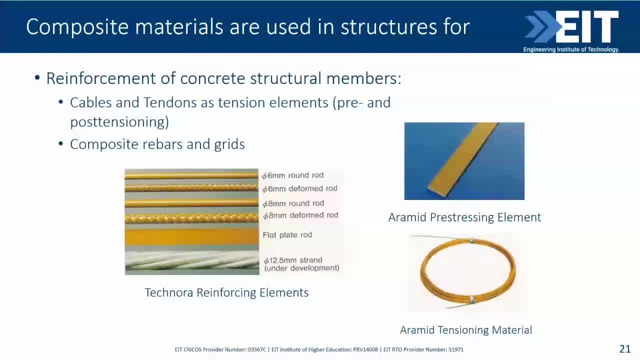 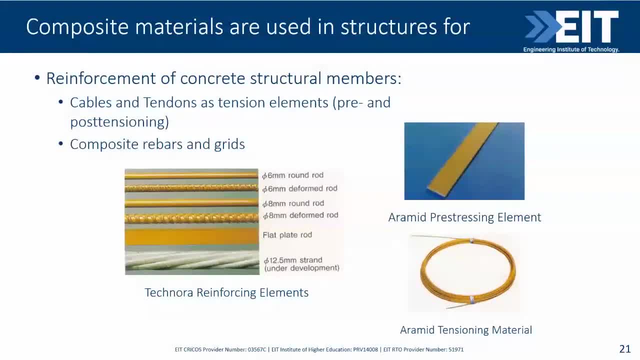 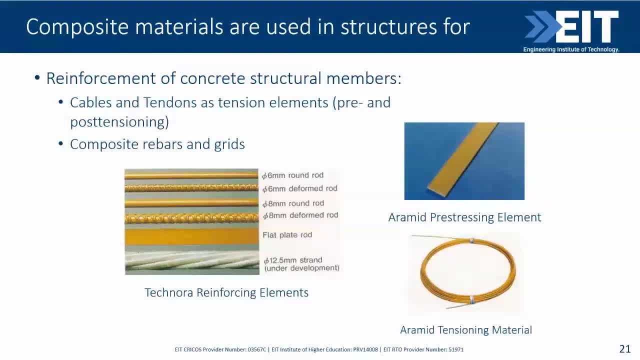 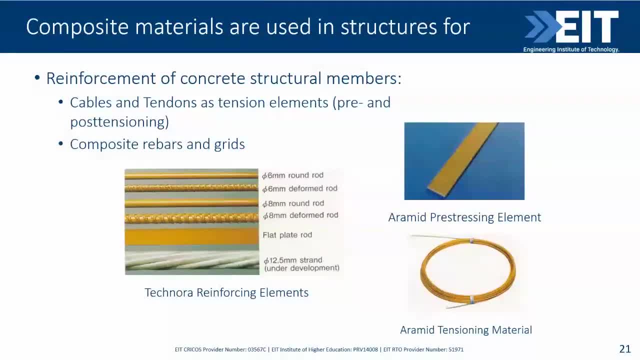 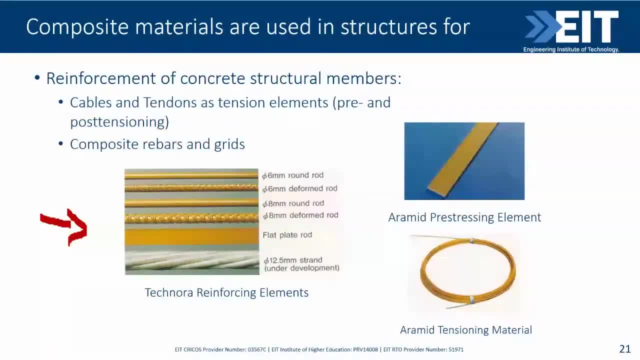 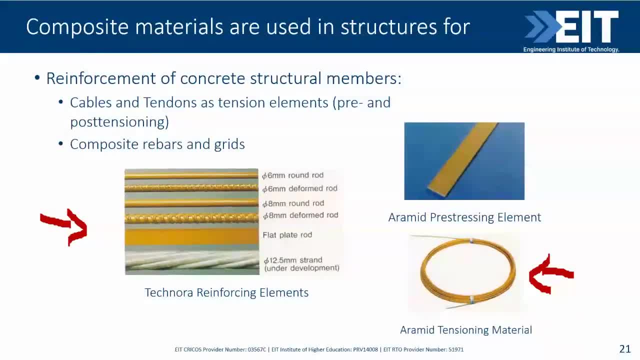 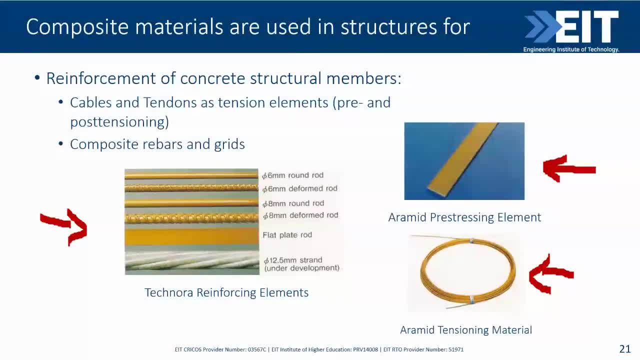 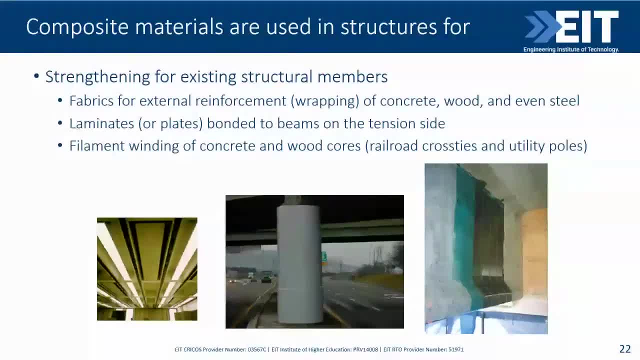 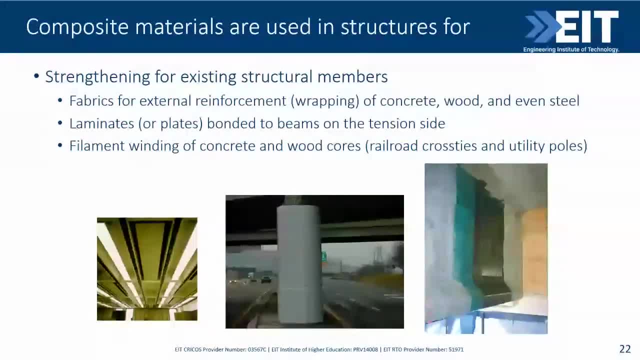 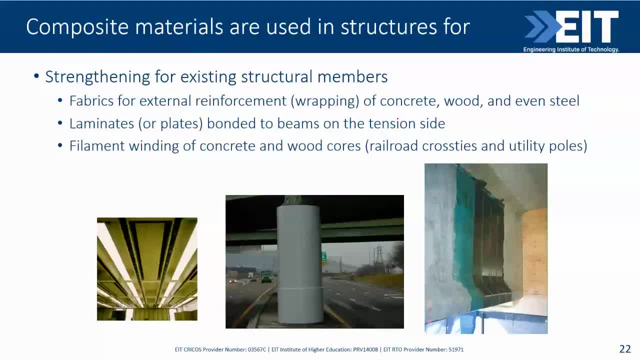 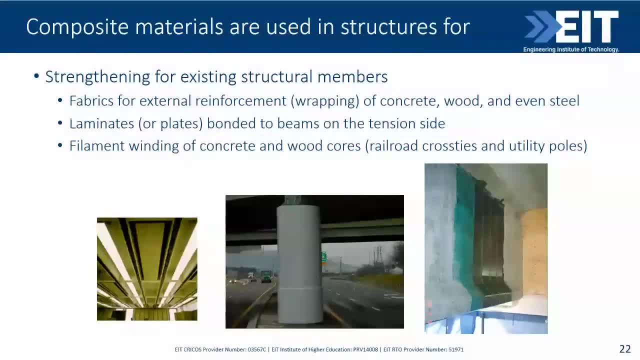 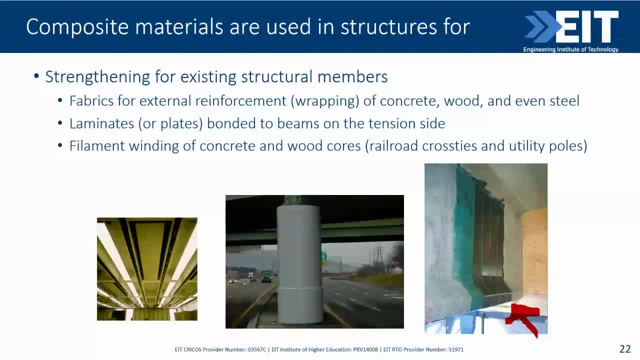 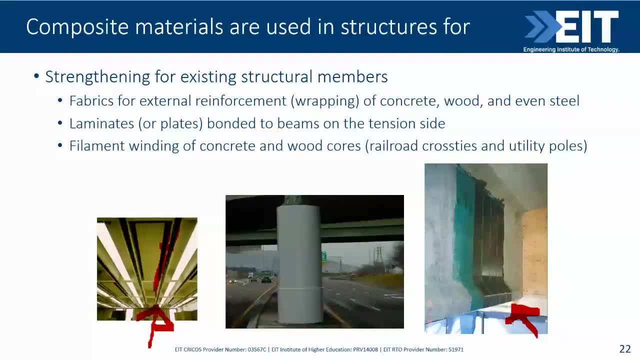 You can see the stretch side of pin or a ceiling Filament winding of concrete and wood cross some posts, like you see here. this example for electric poles is also used for railway sleepers to wrap them and provide additional strength and stiffness. 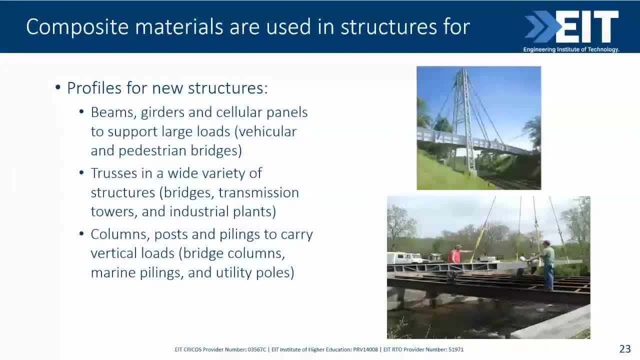 That's the second. The third application which is gaining popularity as well: the production of profiles of composite materials. So the entire profile beam can be made of composite materials, which makes it 10 times lighter. Well, I remember many years ago when some project 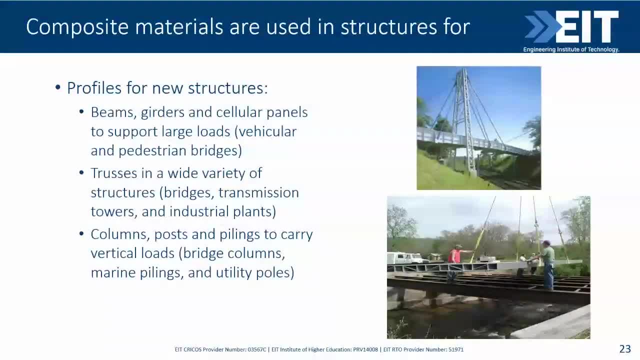 on drilling engineering when they were introducing drilling pipes of composite materials. when one of the participants was brought them to the meeting just carrying on his shoulder about three or four pipes of 10 inch diameter and three meters long, and they were made of composite materials. 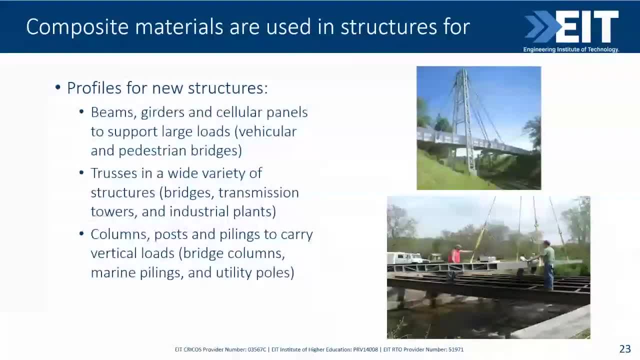 And he burned a bunch. to lift one of them made of steel, you would need a crane And it was quite impressive. So this application is becoming very popular. So production of profiles of composite materials, So some beam girders and tunnels to support lateral 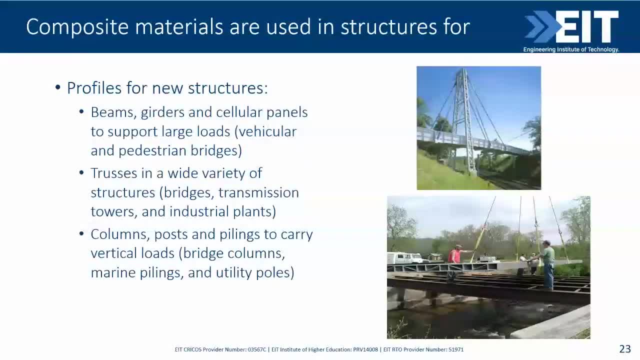 of large roads loads. It comes to bridges. There are a couple of examples- this particular one here- of the fully composite bridge made of compost materials. It is also a good option for trusses because they can provide can be. the elements will be slender, which is you know. 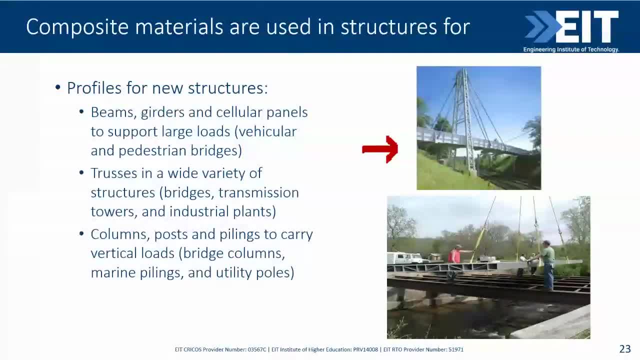 it's a good option for trusses because they can provide can be. the elements will be slender, which is you know the well which is our idea of a truss. They can be also used for corals, posts and files. 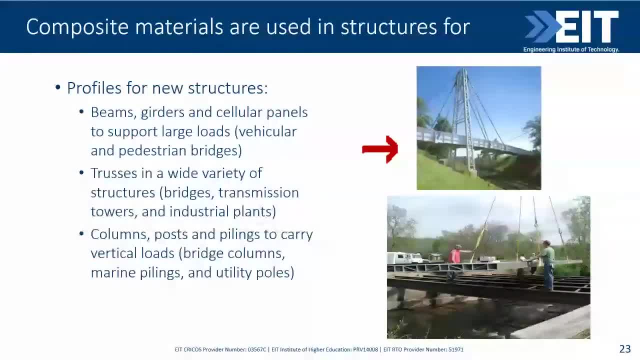 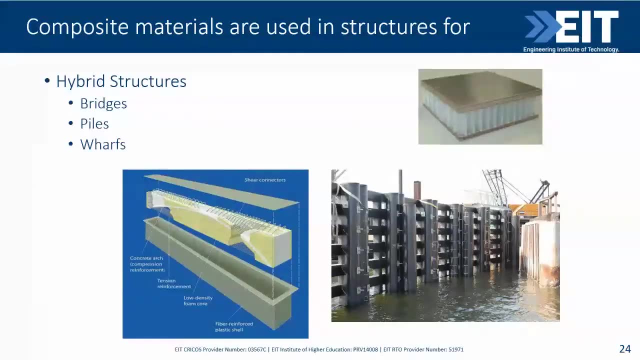 to carry vertical loads in corrosive environment, Marine structures, all different, instantiale as jetty's, and so on. So the last case- Yes, so that's the last one- is the composites were used for the hybrid structure. so what then? we're. 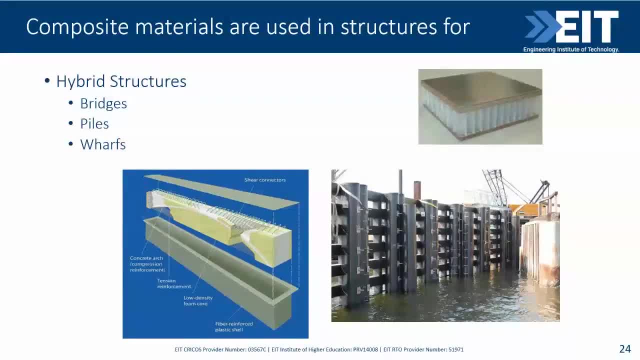 expanding this definition even further. so what's the hybrid structure? so the hybrid structure is the structure which, using many different materials- right, not only is the composite as a material, but, uh, combined already on the on the structural level, like, for example, this, uh, this beam here what you see- i'm not gonna get much details for this- but this shell which forms. 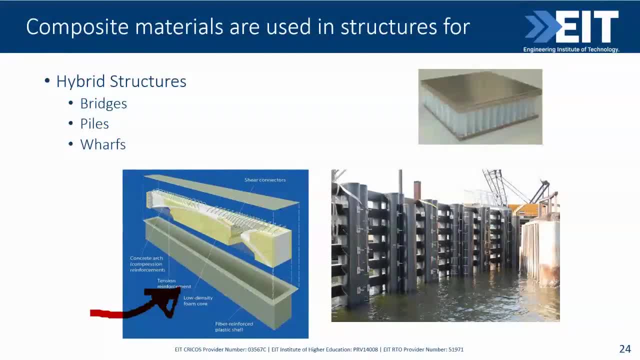 stay in place permanent formwork. i'm talking about 20 meters span made of composite material. then this formwork is brought on site. it's some american company, if you probably, if you have occurred or not, it doesn't they? they actually selling these beams, so they brought this. the very 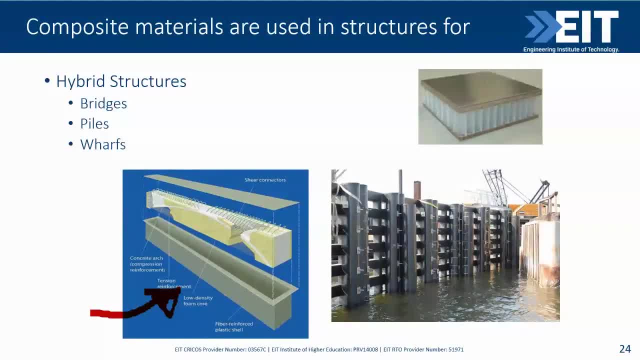 wide formwork and strong at the same time. they have some special arrangements for enforcement. you can see it here: some another structural, another structural idea of arc here inside this, this line, and then they actually cast concrete in place. but the assembly is way too easy because every 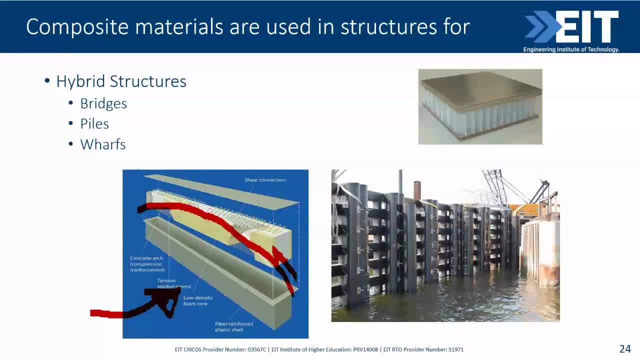 assembly- 25 meter span- is so easy that when you carry machinery pumping concrete doesn't require after at the end. that's one example and hybrid structures like we mentioned. this uh works here with the some corrosion resistant composite composites for the columns and a very simple sandwich panel with composite faces and some solar core. so 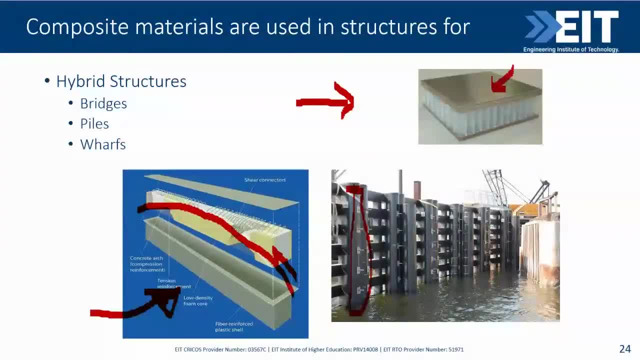 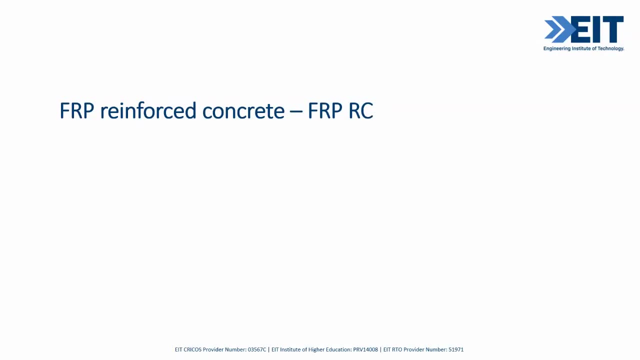 combination again. so we're expanding this definition of composite material into the hybrid structures. so they're getting to the next level of creativity, i believe. so all right next. so let's have a look. we have a bit closer look. i don't think we have that many. 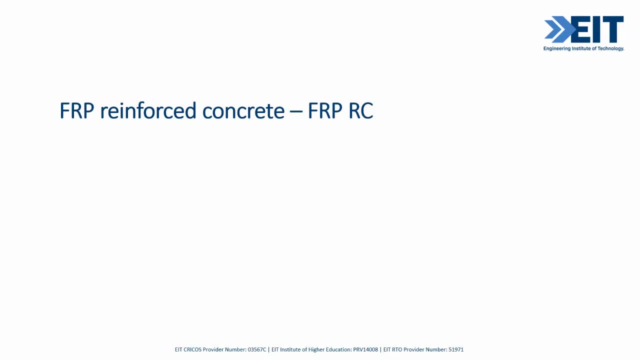 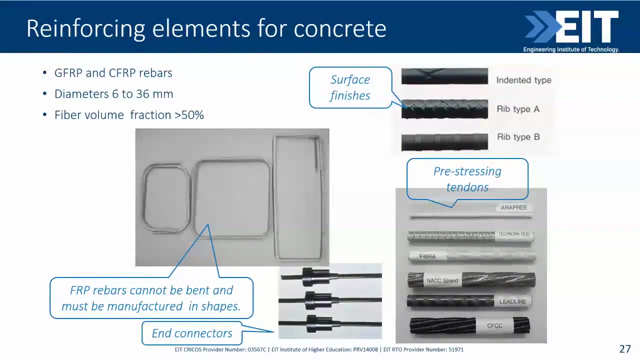 much time i will have. closer look at frp reinforced concrete. we will touch base with the strengthening much shorter and then we'll look at the summary quickly. closer look at the examples of one of the examples, in case that this bridge. more pictures right: frp reinforced concrete. 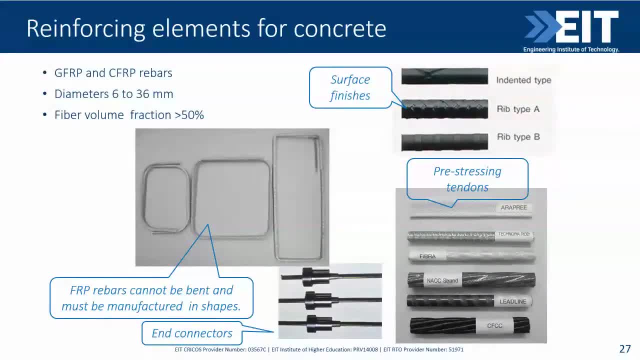 the structural idea of frp, rc, frp, reinforced concrete does not change. the idea is to provide the concrete with tensile strength. that's what steel does in steel reinforced concrete bars and the shapes of the rebars and the stirrups also the same. it's similar to 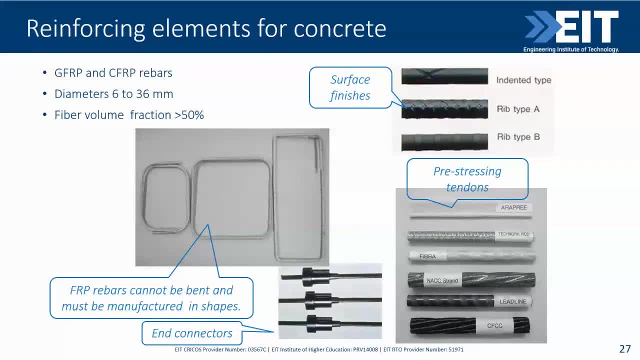 steel, reinforced concrete, the materials used- cfrp and gfrp- the diameters ranging from 6 to 36 millimeters, and that's already in the production line. the fiber volume is higher and it should be higher than 50 or 50 percent into this rebars right. 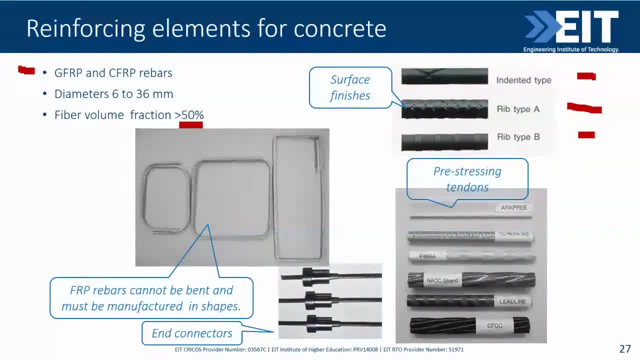 into this rebars, on this, this kind of rebars. what is different? i'm saying the same, but different. what is different? well, uh, this rebars made of frp cannot be bent on site like we can do with steel, so they must be the whole arrangement, prepared off-site to the final specification. so all these, 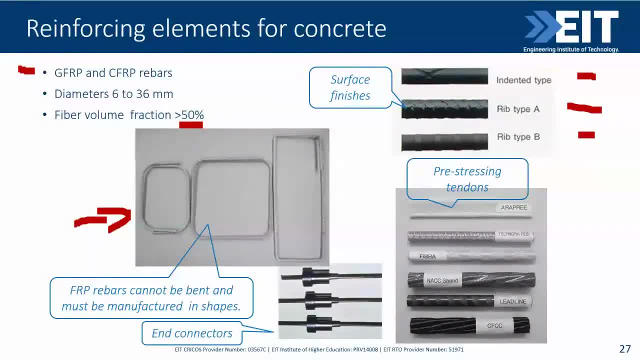 shapes must be done proper, the proper sizing off-site and brought to sign for casting or pouring concrete. another difference is the end fittings, especially for cables. they be different, different and the adhesion strength is low between the concrete and frp is lower than the steel but that's a minor problem because we're using the all different rib profiles. 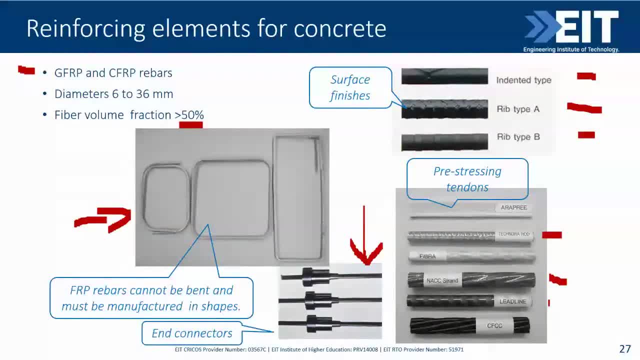 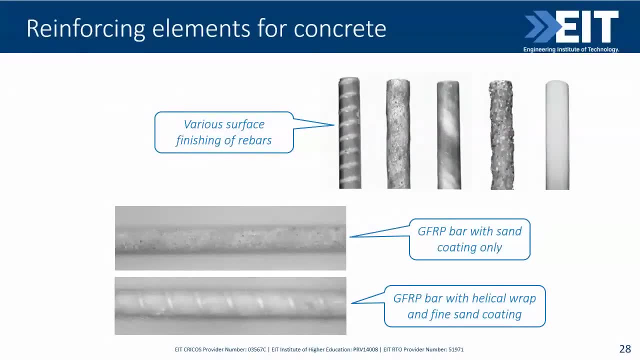 all these profiles. also, there are some methods which are improving this pull out resistance. so the next connection: so increasing this adhesion or improving the pull out resistance. so if we compare this to steel, the methods are different: coating, so we see a very surface finishing, so it's different coating. 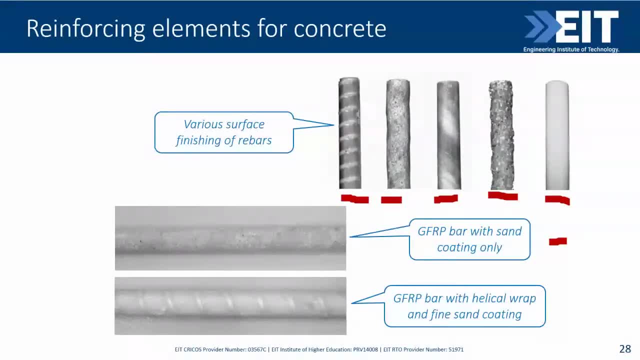 ranging from coarse sand or somewhere. that's the sand, fine sand glass. so to improve the, the adhesion, like in the steel glass as well. so it's a little bit harder to make here the, this ribs. so can be done by some helical rock, for example here. 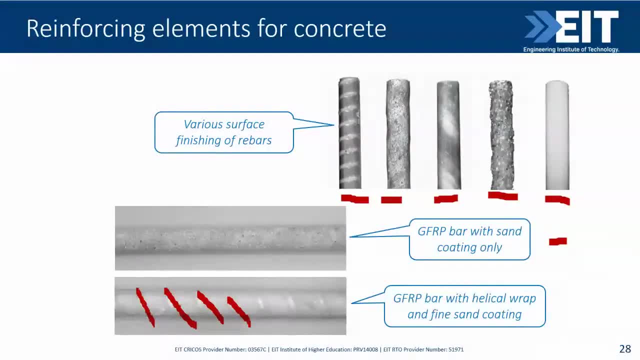 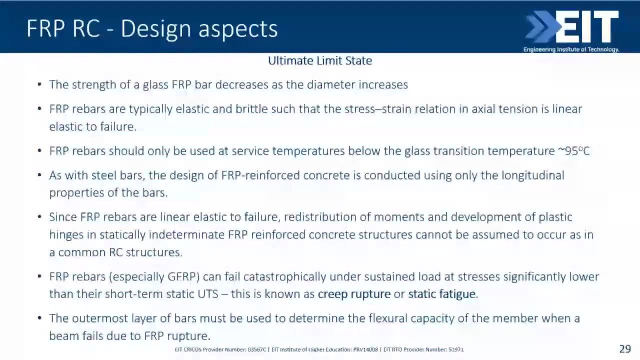 but in general wall width brings that's the pull out resistance. so the resistance of the frp bar is higher than steel bars can be. right design. so we're looking at the ultimate limit state. i believe many of you are familiar with the idea of limit state design. so we've got ultimate limit. 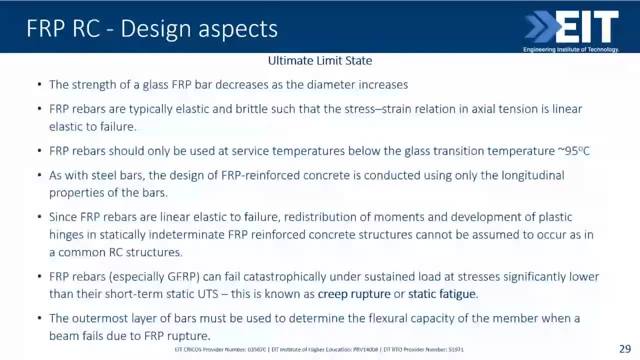 strength, sometimes called strength limit state. but this includes more than strength, including stability, includes the fatigue as well, and serviceability state. so we will, we will address here to them: so uls and sos. so in ultimate limit state, design of the concrete. so in ultimate limit state, design of the concrete. 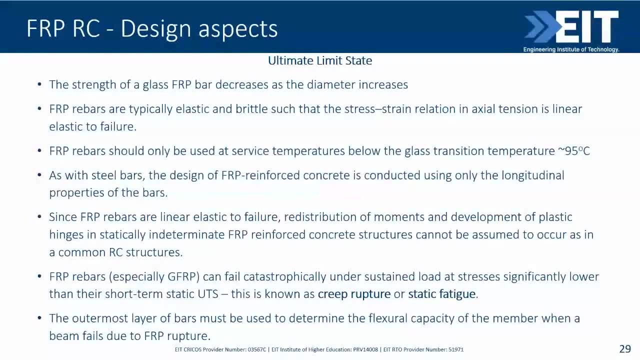 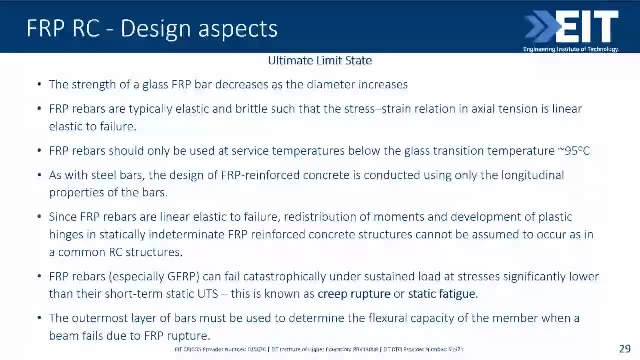 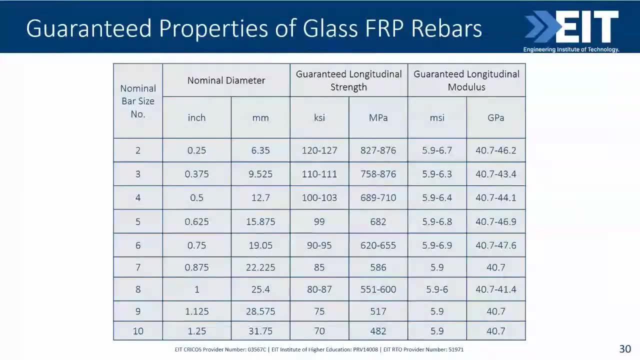 or frp bars decreases when the rod diameter is small. right, we've got this picture here: the smell, this, the strength when we are using small diameters roles. they only have this range of strength when we're using it. see, on the other end of this range. 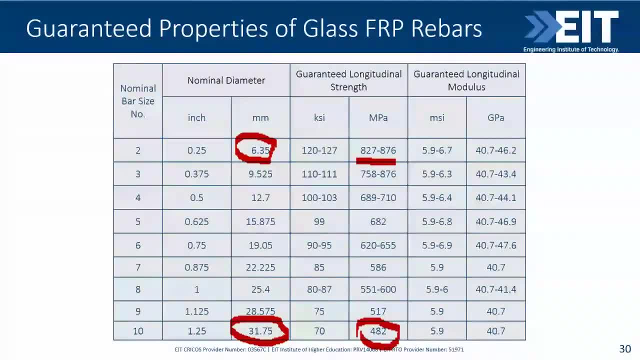 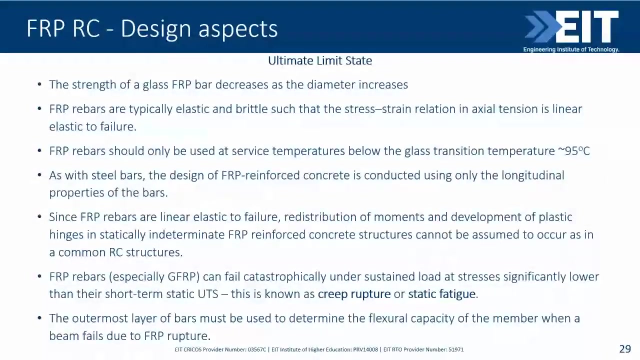 it is decreased by about 50%, from almost 900 to 480. the model is, though, doesn't change much. you see what stays in the same French, so this. this can be explained by the fact that the stress developed at the fiber located near the outer 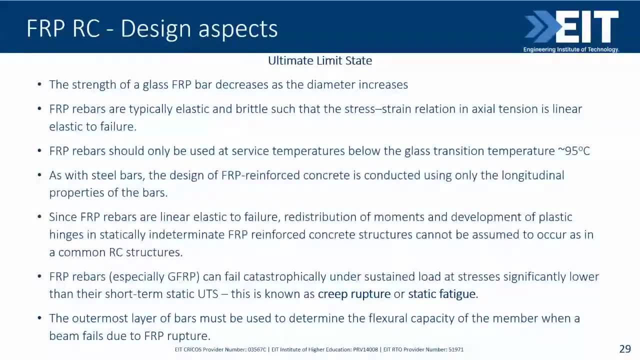 surface of the river is not fully transferred to the fibers located in the center, actually part of the fibers failing, while we have still in the most of the of the section is intact. what else? frp reverse? usually elastic and brittle. so so the stress-strain curve is the is linear. until failure, the frp. 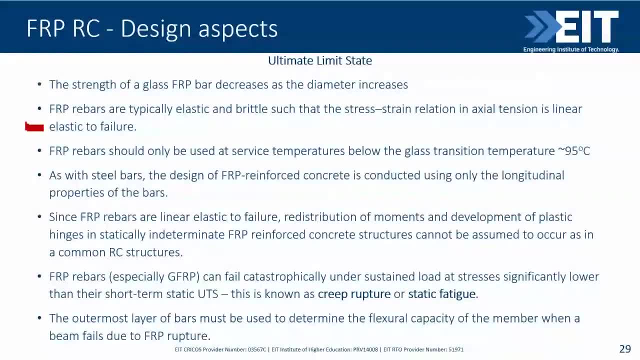 roads should only be used at service temperatures below last transition temperature. so we have this limitation of the temperature, as we're still barred if appearing force concrete design is carried on using only a longitudinal properties of the process, it's the same actually so, since the therapy bars are. 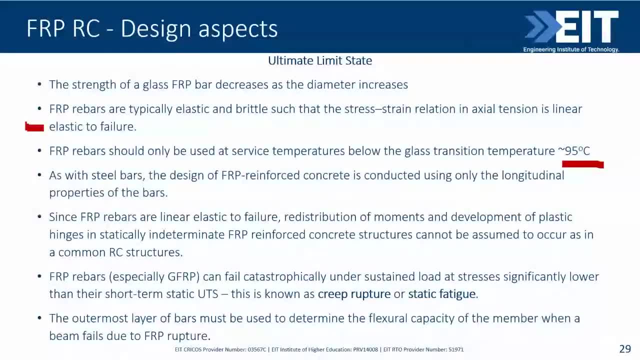 linear, elastic until failure. the formation of plastic joints and redistribution of moments is statically indeterminate, which makes it harder. reason and due to the creep and fatigue problems, a frp bars, especially gfrp, may fail catastrophically, and the continuous load at stress levels which are much higher than the ultimate tensile strength. 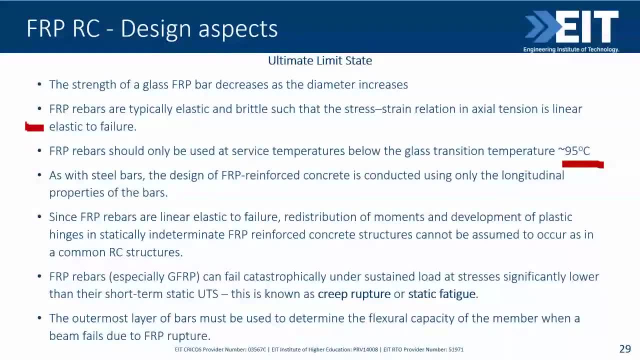 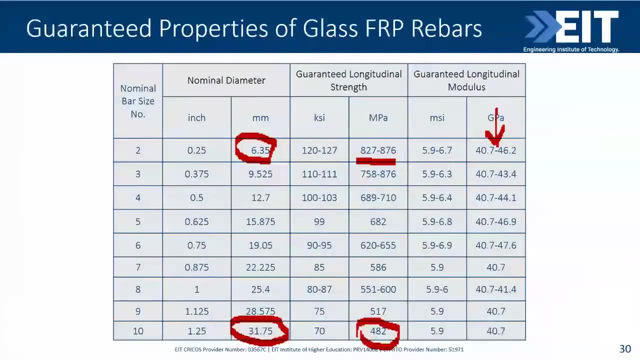 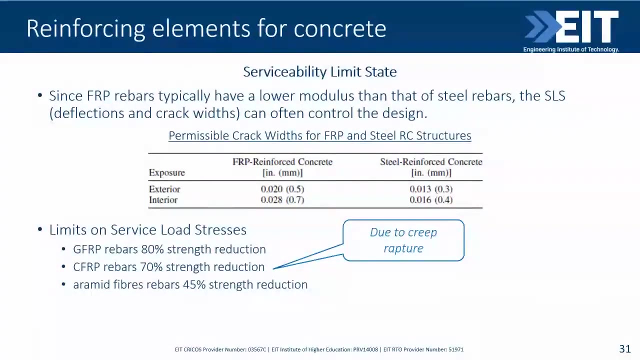 the brittle failure of frp. the, the outmost layer of the bar, must be used in bending tutorials calculation, so it's a bit, a bit tricky. so let's have a look at the serviceability industry, which is actually, in this case, will be a more important. 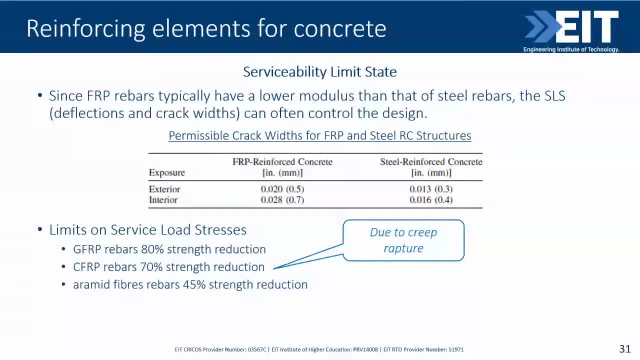 so well. frp bars typically have the lower models than the steel bars, so a serviceability limit, state deflection and crack weights can often control the design, the uh, the crack. so if we look at the it's american code, so permit permissible crack weights for frp and steel rc structures and when we compare this with steel uh, we can. 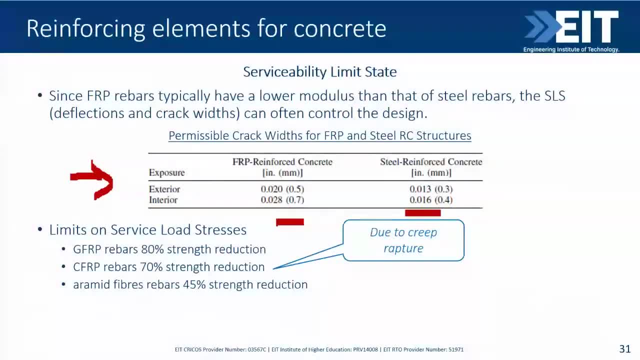 see that the permitted crack weights is in concrete structures. in the frp, reinforced concrete is greater than in steel reinforced concrete. the reason is simple: we don't have corrosion problem. we don't need to defend the steel from influence of environmental influences. so the other thing here is the limits on the service loads are much higher in this case. so the 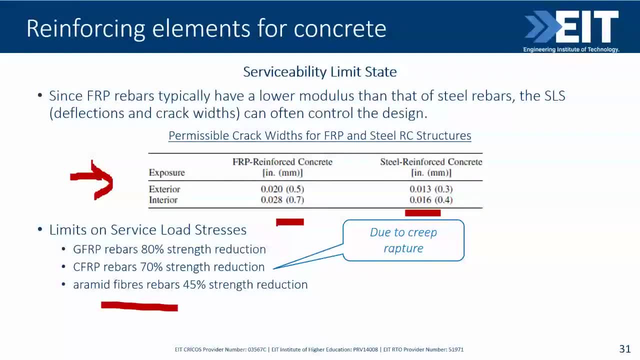 resistance factors we're using for serviceability in this thing are higher and that's the again due to the creep rupture, due to the creep problems. so they can go for the aramid fibers up to 45 strength reduction. so the design resistance, the resistance factor, will be much lower. 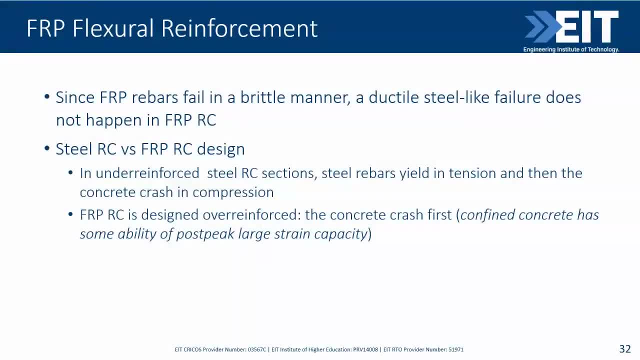 right. the main difference within design of frp and steel reinforced concrete is due to the fact that the failure of frp is brittle, so and failure of steel is ductile, so, as a result, the steel reinforced concrete is designed is under reinforced, which means the area bars yield. 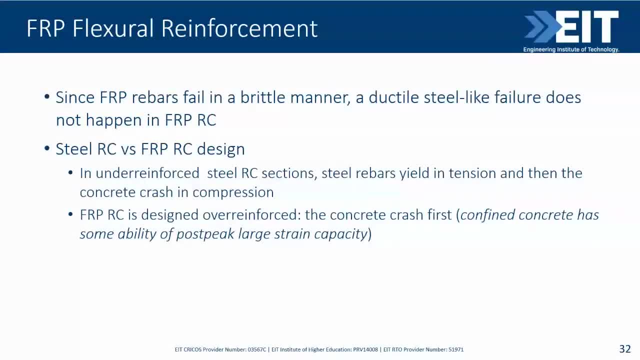 intention and then concrete crushing, compression. that's what we do in conventional concretes. uh, happens with frp- is essentially over reinforced because the concrete will crash under compression first. uh, and it is. it is before. there is strong fibers, very strong rebars will yield, they will. 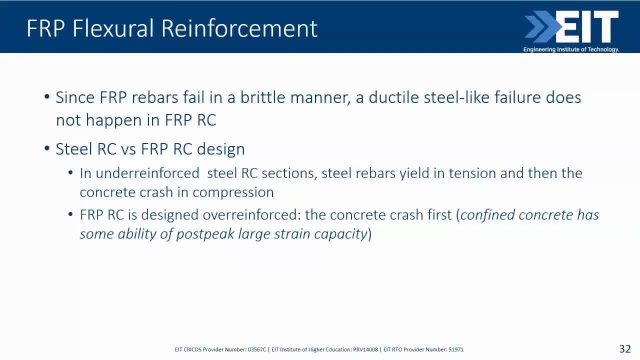 they do not yield but they fail. well, it is actually possible, because concrete does have some post fixed strength capacity. it is possible because concrete does have some post fixed strength capacity. it is possible because concrete does have some post fixed strength capacity. it is possible because concrete does have some post fixed strength capacity. 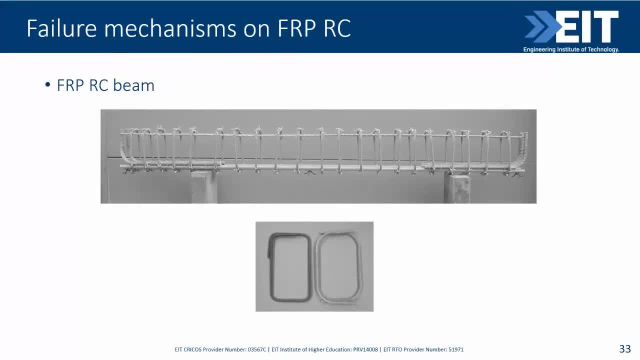 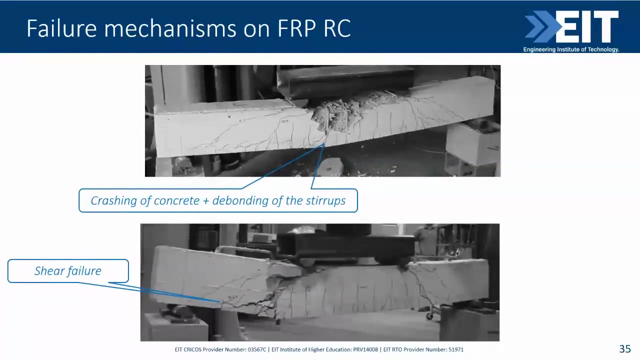 everyone. let's have a look at this. they got an example of some typical frp reinforcement cage and which needs to be pre-manufactured. offside the failure of uh, if appearing force concrete. here- that's the example that's i just mentioned- we can see a beams are failed due to crushing and concrete. 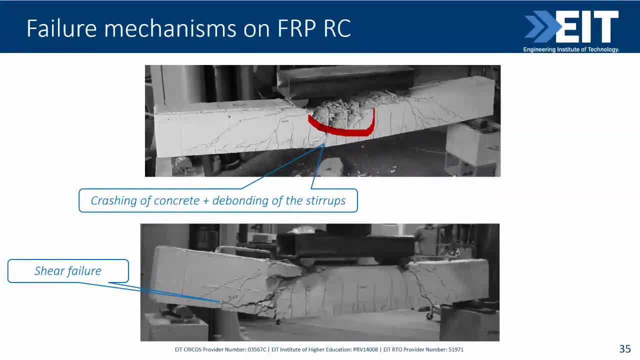 and the compression zone, uh, or the bonding of stereos over the tension zone. so it's not really a kind of really see here on this small picture, but it's there well. also we can notice the large diagonal shear crack here due to the lower shear resistance. 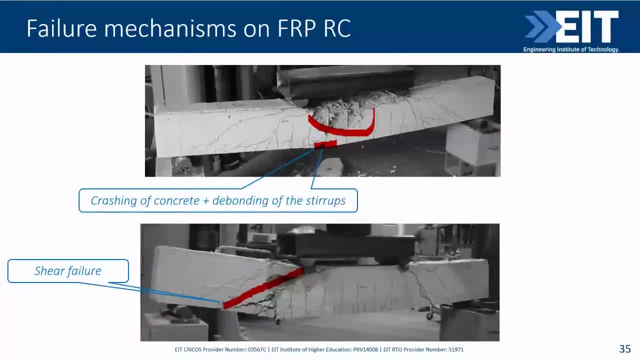 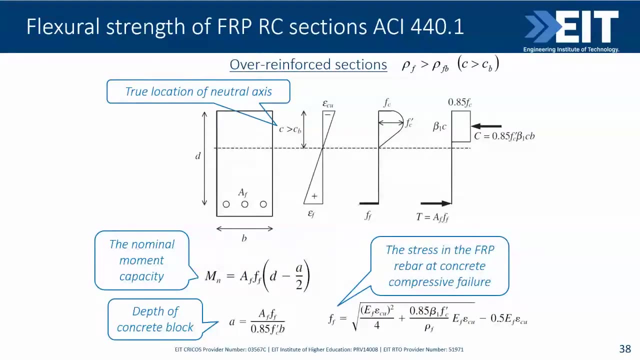 or the shear failure as well. that's the main uh failure mechanism in frp range force. concrete elements: all right. so when we look at the computation of flexural strength of fiber, reinforced effort here reinforced concrete. excuse me, we use the this common reinforced concrete model, all right, reinforcement concrete part. anyone who does structural engineering a very familiar with. 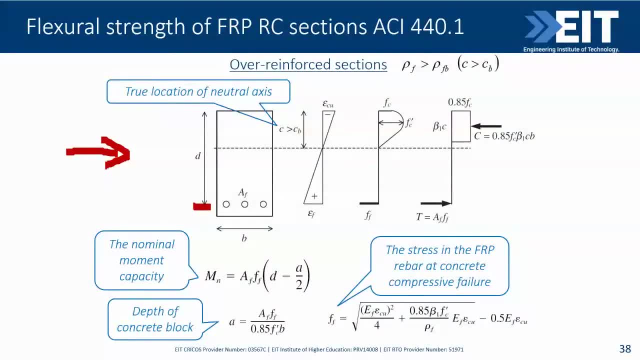 this and even then solid mechanics is discussed. so have some kind of a hybrid structure. uh, do you do? is the a f of p? reverse is very high. stiffness: the neutral axis- here is neutral axis- can be very high. that means this compressed concrete zone will be small when we calculate the 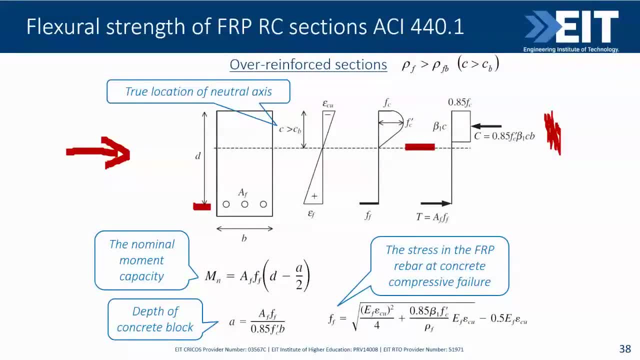 c. i just shortened a couple of slides. i believe if you and download the, you the the slides, you will be provided. there will be a couple of extra slides there with more details there. we don't have much time to go through them. so when you calculate this c, it will become, and i will find out that it's quite low because the stiffness of the fiber 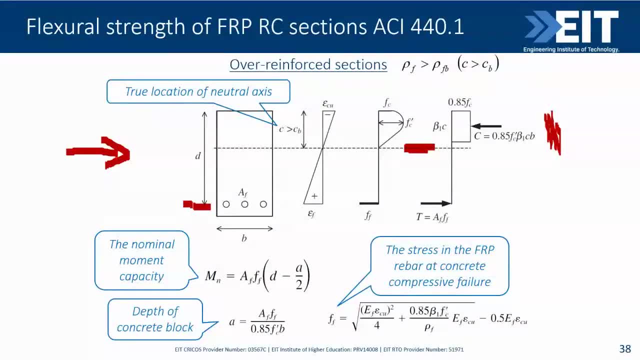 here is high, and other problem is- this is a well well known for structural genius. flexural resistance factor 0.9 is used for tactile failure of steel reinforced concrete and then in this case it cannot be used at all. so the resistance factor is low to 0.65. 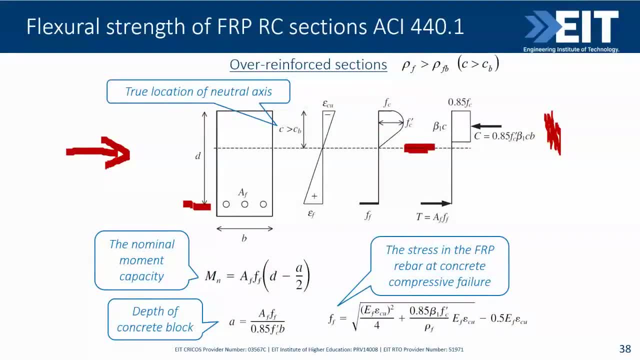 now all standards technically allow the use over or under enforced design. for this, however, the series serviceability limit state, the deflection and crack weights will impose higher reinforcement ratio. i didn't bring the expression here again generally, given the general picture, and so the if, if, the and the higher reinforcement ratio. 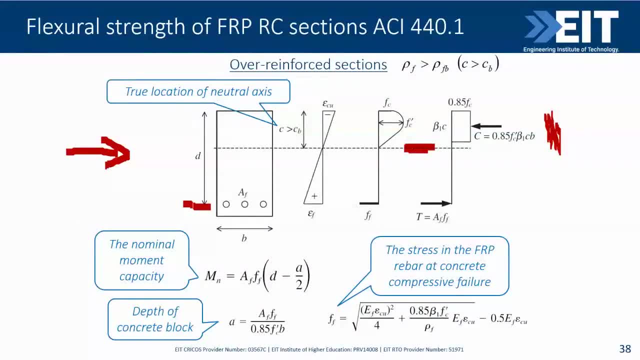 means over reinforced conditions. so, as usual, in this case, the nominal moment capacity. this one is defined as a couple, so there's two forces. with this, it's never calculate this couple. we have this, uh, reinforcement force and compression. so that's how we calculate the normal capacity here. 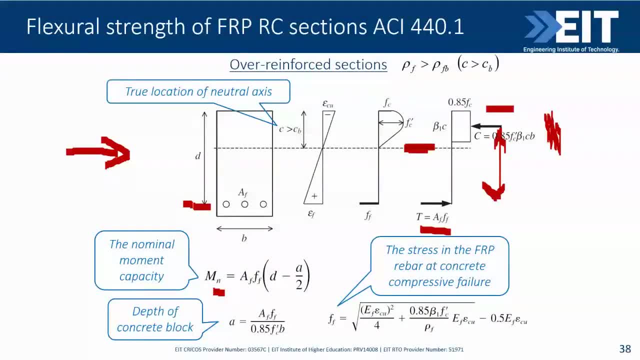 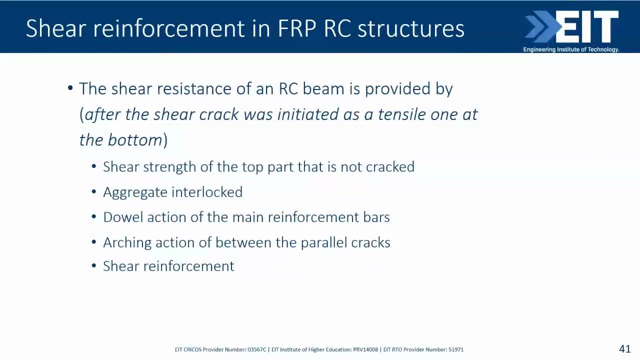 however, when we use the this case, we cannot use the yield in steel reinforced concrete. we use yield strength of steel to calculate these forms. we cannot use it here because there is no outcome right. the shear resistance: let's say a quick note into the shear resistance. so the shear resistance of steel reinforced beam is provided by shear strength at the top part. 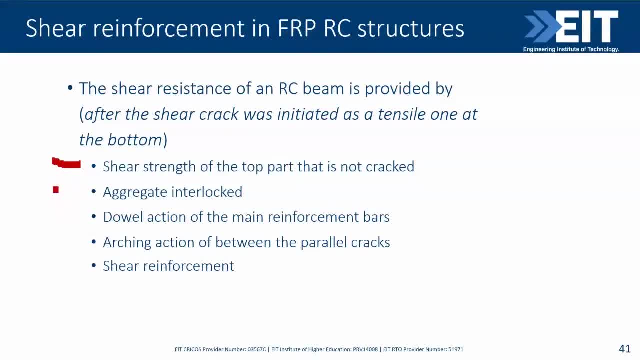 when it's not cut, cracked by so-called aggregate interval, which is the friction between two sides of the craft beam or two sides of the crack, and then double action of the main reinforcement inside of reinforcement bars, or double action arcing or elbowing action between the parallel tracks, right when they want. 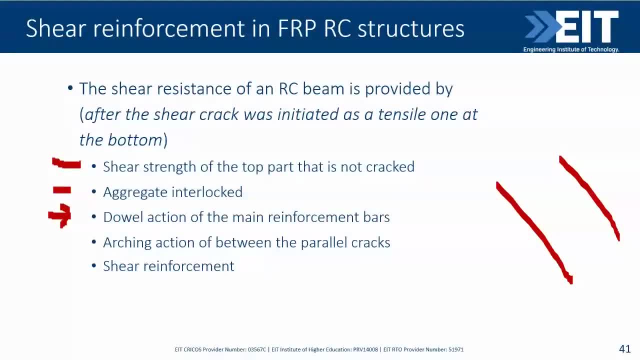 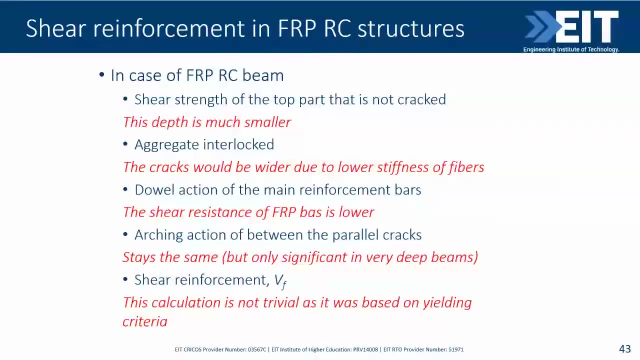 to rotate, they actually elbow each other and they cannot move, so which provides additional shear strength and the shear reinforcement which we add there. however, what's the difference is when we look at the frp rcb, the shear strength of the top part is not the first one. this 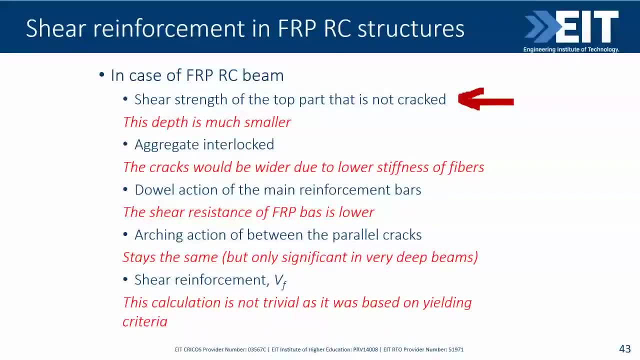 in practice the difference is again the depth, like we said, of the neutral axis, that the compressive part of the concrete is quite low, so much less. so the contribution of this will be insignificant. aggregate internal work. what happens with this? aggregated to work, the weights of the critical diagonal crack? 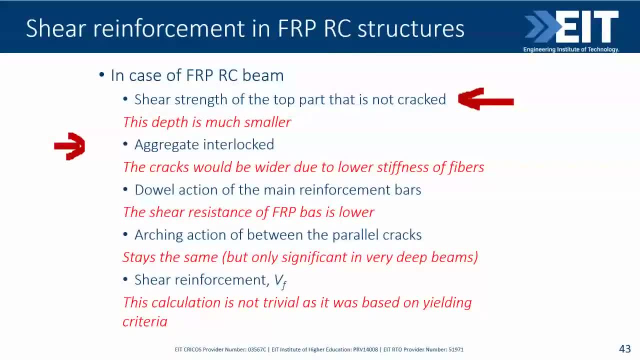 in the in frp reinforced beam is likely to be wider because the flexural stiffness of frp- actually over rebars- is lower. the strength is higher but the stiffness as well. so it's likely to be wider, which means we'll be reducing the, reducing the. 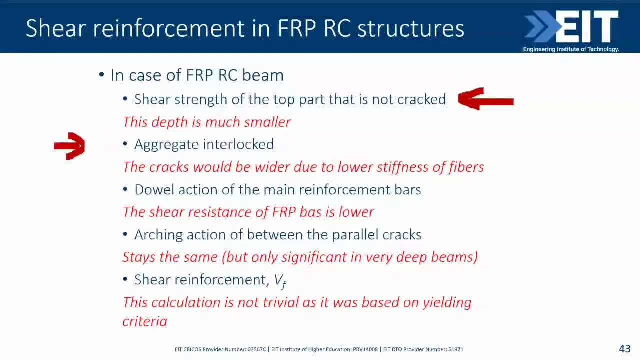 this contribution as well. dowel action, the third one. the problem is that the shear resistance is not the same as the shear resistance of the third one. resistance of frp bars is lower. we're also losing from this, but it's about the elbowing. elbowing, it actually stays about the 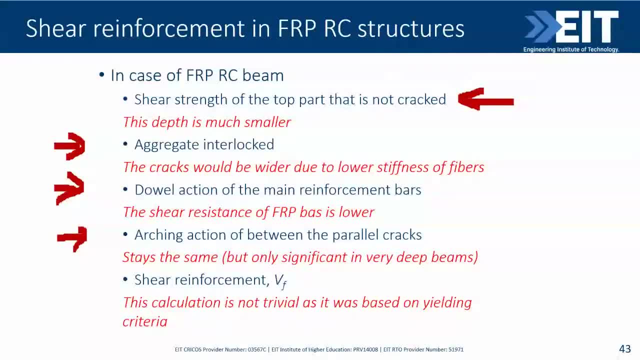 same. but this becomes only significant if we have deep beams, otherwise this effect overall for very shallow beams is already insignificant. the shear reinforcement, uh well, this calculation, i say, put here not trivial. the stirrups do not yield so the stress, and if a fist here cannot be calculated in a simpler, 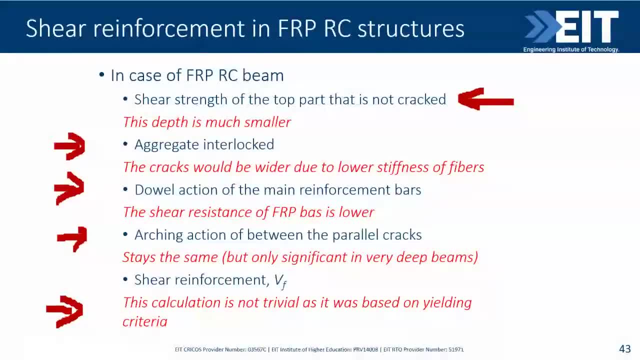 manner which is not forced and it still stir up as we do there, which way actually use the use as a displacement in the bar. so this calculation is not trivial. however, the we still need some codes for this, but there are some already provisions. but overall, the conclusion for all this is: 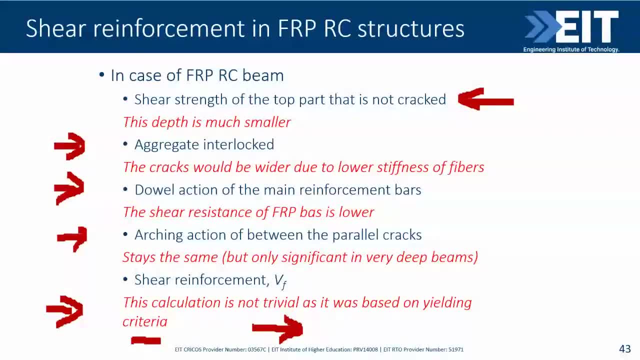 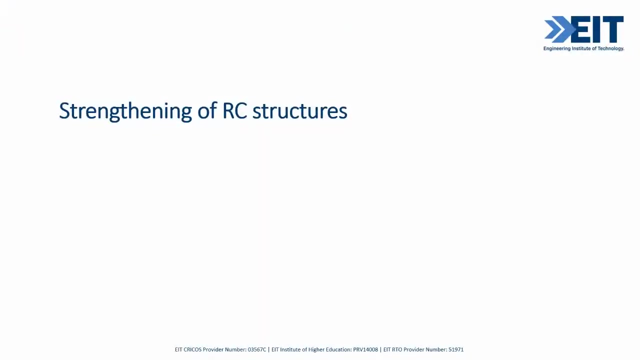 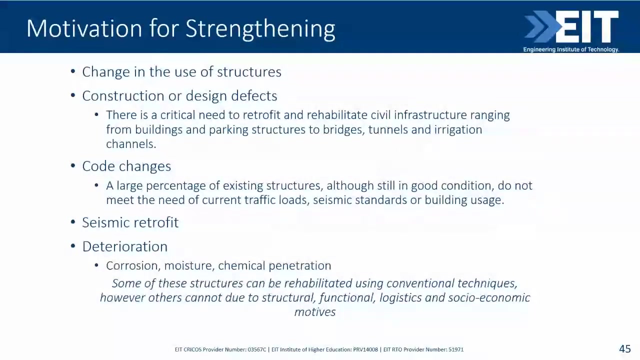 that's the shear strength of. well, the shear strength of the fiber reinforced beam will concrete beam will be lower, so needs some additional attention. all right, okay, so the next part. well, probably we'll do briefly. a strengthening of rc structures, is it? uh, uh, um, um. And the replacement? what's the catch? The replacement of the functionally deficient civil infrastructure is not a feasible option In most cases. there are several reasons. 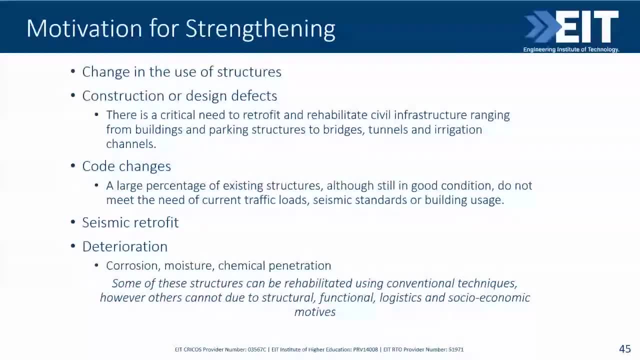 In most cases they range. It is not optional in most cases because the reasons range from economics, simple costs, to logistics and some social economic impacts. So it's to remove the inhabitants there for a considerably long period of time. Would it be just tenants or industry or something? 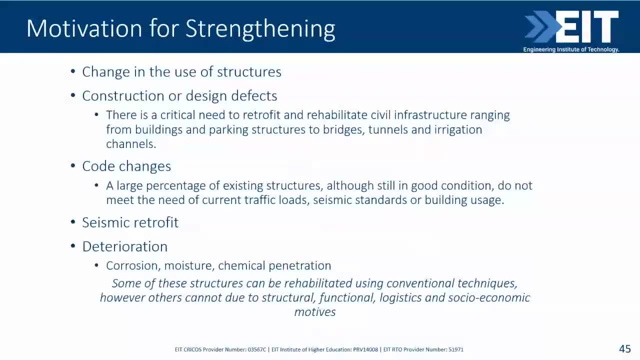 Companies, it can be quite cumbersome. so a large percentage of concrete structures that were built in the 50s and 60s are almost still in good condition. They do not meet the current requirements, current standard requirements, especially bridges or current traffic roads. 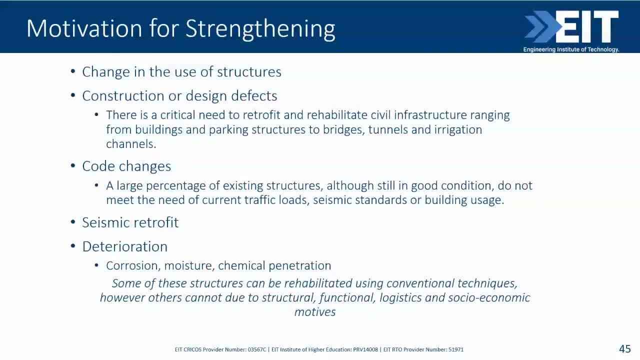 but the seismic standards have changed, So another thing which can affect this is the change of the building purpose, so different usage for a building or structure. So all these leads that we need these structures needs to be improved, needs to be straightened. 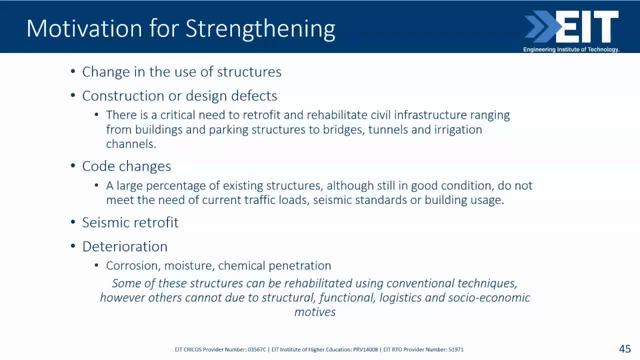 Some of these structures have deficiencies in the design, materials and so on. So deterioration of materials is also a problem, And if we want to retrofit these structures using conventional techniques, well, it is obviously possible, But involving some problems or removing people around. 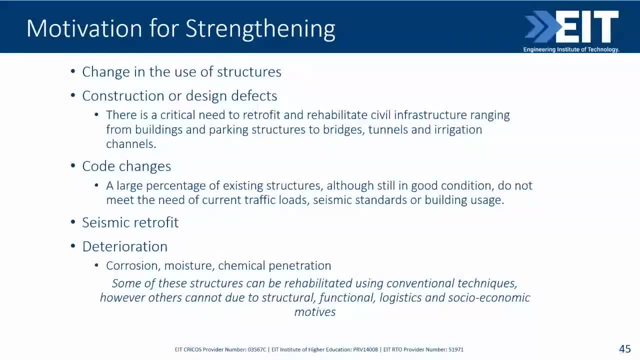 But in many cases it cannot be done due to some structural reasons or function increases. So we cannot add more steel. Simply speaking, we cannot add another steel beam into the car park, right? Because then we will lower the clearance and it cannot be used for the some. 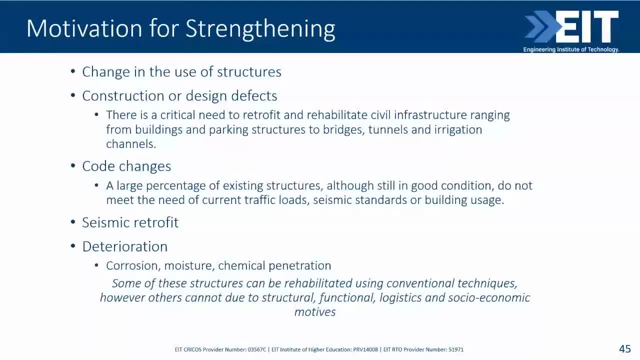 So we will reduce the clearance in the car park, So we are reducing the use of it. So all different reasons for this And the use of fiber FRP composites presented itself And, like I said, 20 years ago, it was an attractive option in all these cases. 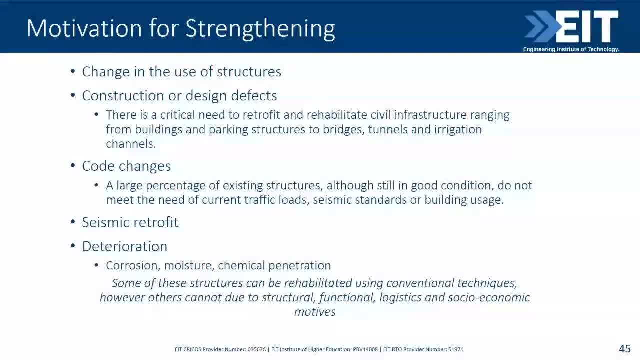 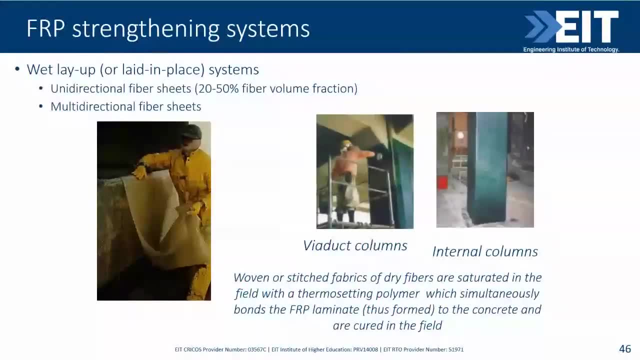 And it has become very popular since then. So let's have a quick look at this. This strengthening system includes mainly- we can distinguish two, So one is latent place, FRP sheets. So the latent place meaning that's the, actually the fibers coming inside. 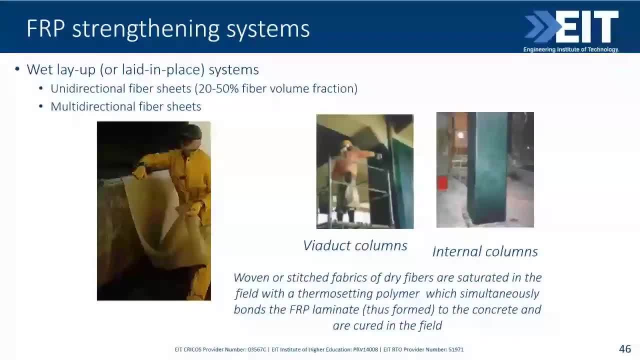 In the form of fibers or some mats, woven fabrics, And they're saturated with polymers on the side. That's what you see in this picture, actually This one- And they're on the side And they're cured in the field. 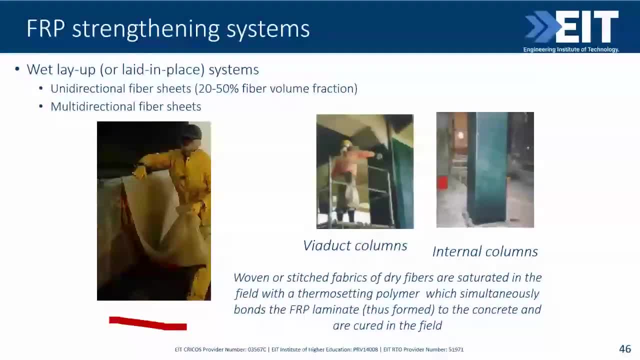 And they simultaneously, at the same time, create a bond between FRP and concrete. So when you actually do this latent place cases- that's the resulting wool- One actually apply the sheets of the FRP sheets- only the woven fabrics- And then they apply the polymer. 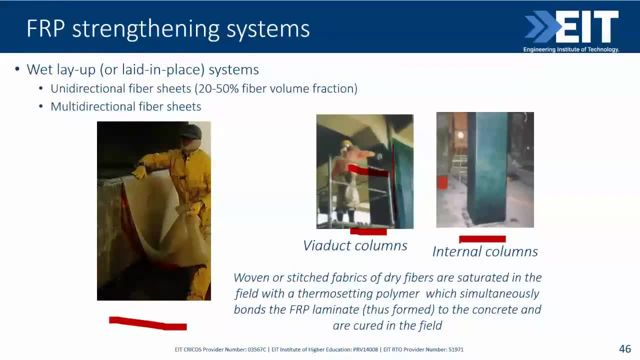 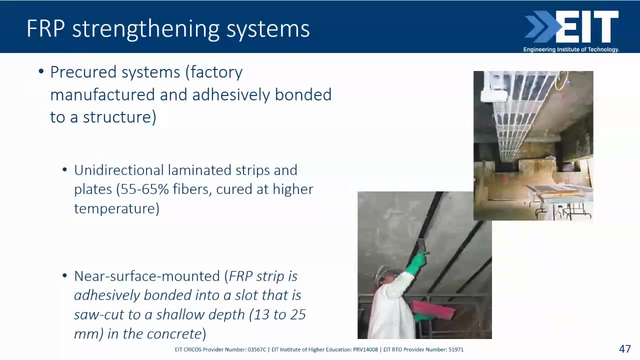 Applying the polymer, So you see some kind of FRP on place on side. Well, it is definitely will be The lower volume of fibers, Because we cannot do this manually. The other way is: some use some procured systems, So ready, off-site manufactured composites. 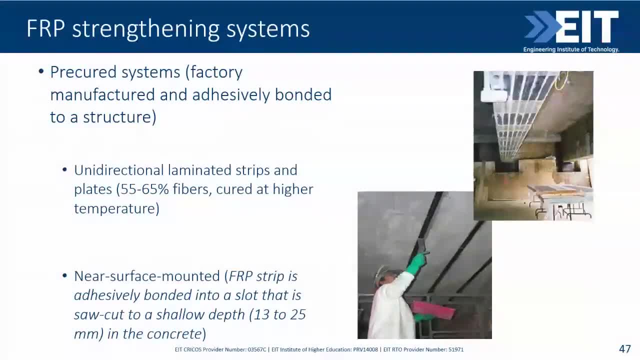 And they will be bonded to the structure on side. So in this case, mostly unidirectional laminate strips. So it's in this picture. So not enough of this picture And this one. Strips and plates with high fiber volume content. 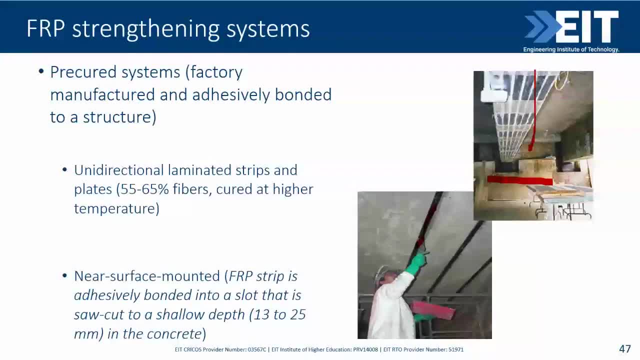 And the other option is actually so-called near surface mounted strips. So for this case, the cuts, the slots, are so cut here Relatively low depth, About 20 up to 25 millimeters, And then into these slots FRP strips are easily bonded. 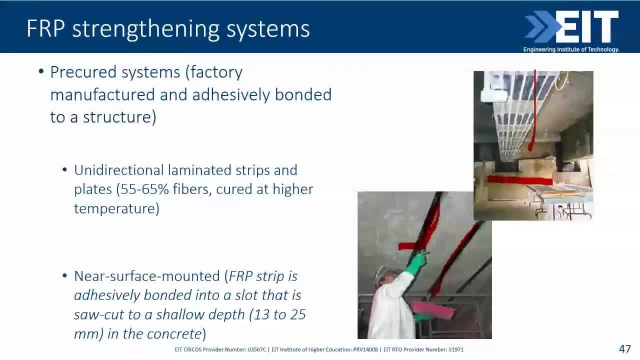 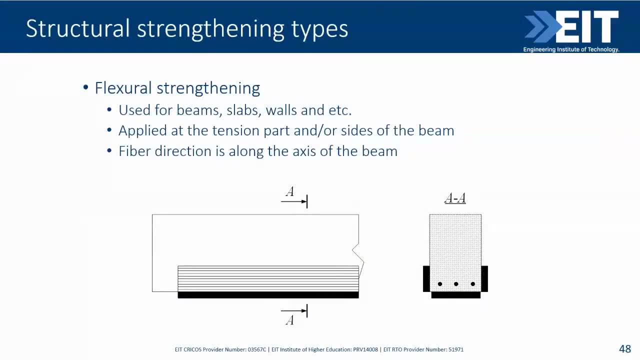 So providing the additional strength, That's the procedures, That's the systems. In terms of the structural terms, The types of strengthening should be selected by the type of resistance to be improved. So, if you want to improve flexural resistance, shear or axial strength, axial resistance. 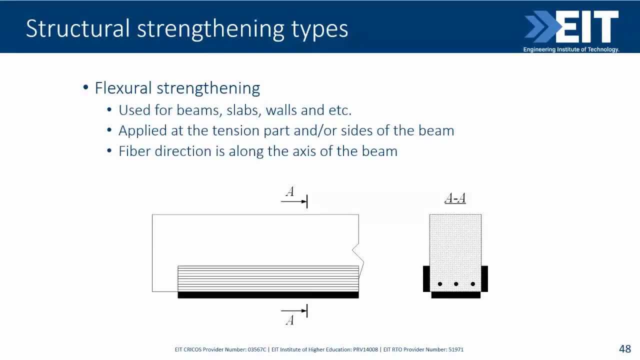 So we will call it flexural shear or axial strengthening. So the flexural strengthening is used for beams, slabs and walls. It applied at the tension side of the beam, The tension side, And go aside. But there's no point to apply it higher than the neutral. 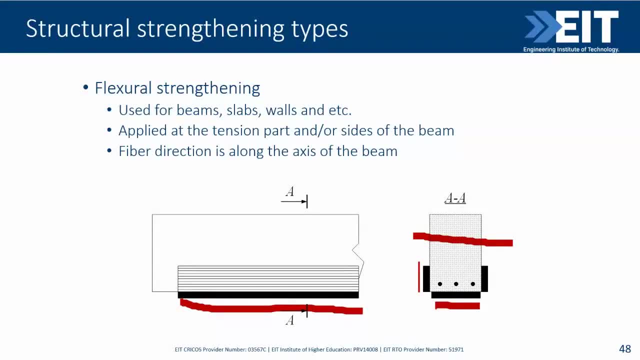 And there's no point to apply it at any compression Because it's not going to work there. So the fibers- actually the fibers- will be oriented in the long the axis of the beam for this case. The other one is shear strengthening. 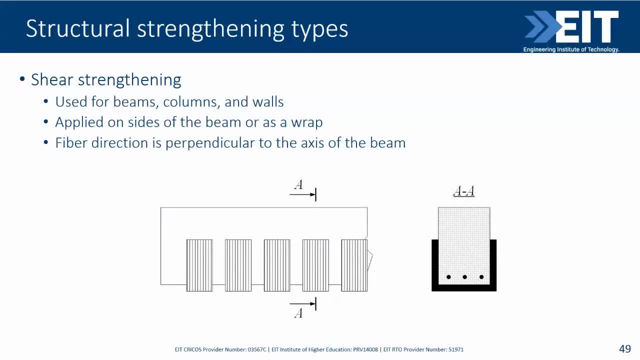 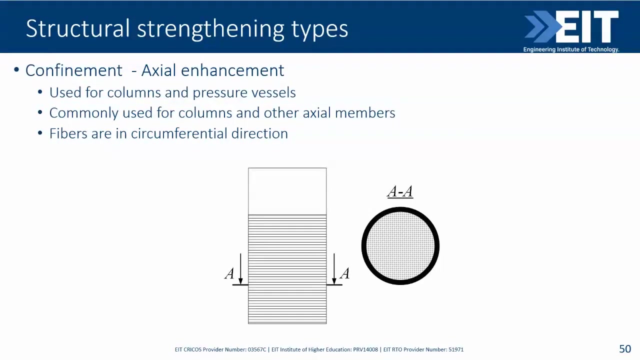 Which is used for beams, columns and walls, And it applied on the side, Which can be even go all the way around Wrapping the whole web, And the fibers in this case are oriented perpendicular to the axis. The axial enhancement is done by providing a confinement. 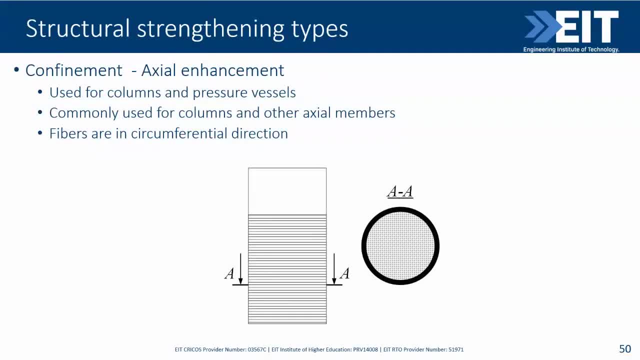 Around the compressed member- If this is my compressed member column- Axially compressed, So we provide the confinement Which will restrict the expansion and the axial compression And will improve the resistance. So the fibers in this case are oriented in circumferential directions. 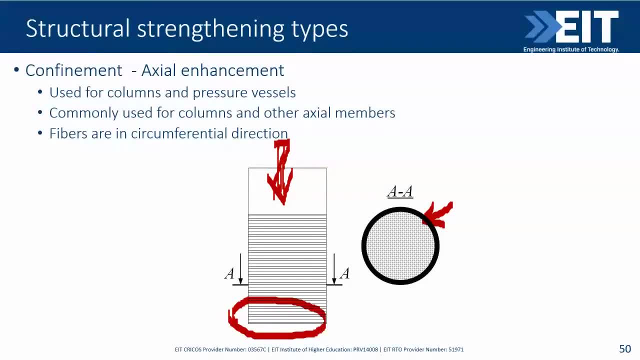 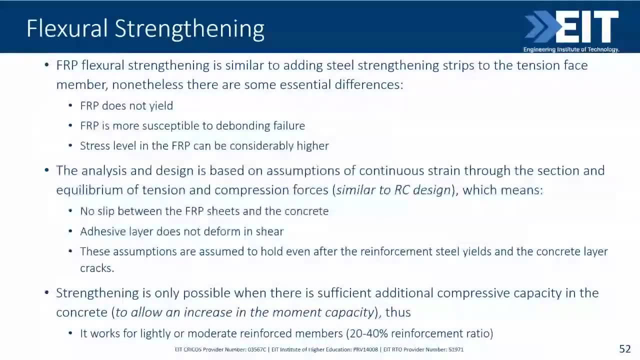 So around Winding filaments around the column Right. So flexural strengthening, Let's just highlight a couple of things. Flexural strengthening by FRP is similar to strengthening by adding steel plates. So we would add them in the tension side of the column. 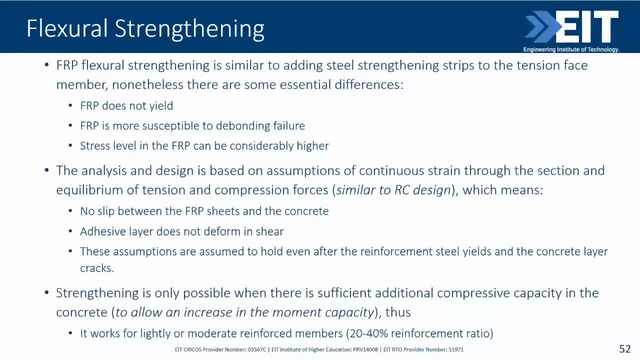 But there are obviously some differences here, Besides the difference that the steel we need to add massive amount of material And FRP will add very thin plies, Which will be easier and will not require stop functioning the building, But structural differences. That's what I want to highlight here. 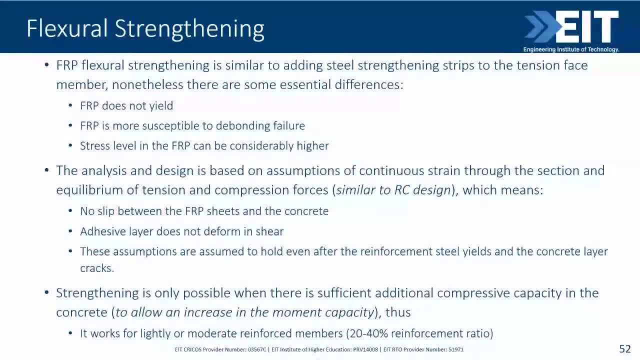 What's the difference? The number one, We've mentioned it many times today already: FRP does not yield Brickle. FRP is more susceptible to delamination failure. It can be. The stress level in FRP can be much higher. 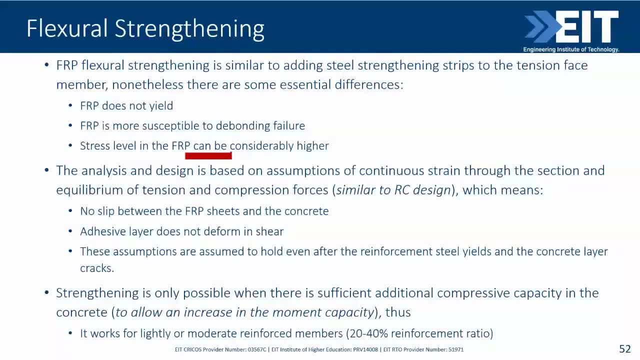 Which needs to take into account, And the analysis and design Based on assumption of continuous transition and equilibrium Of tensile and compressive forces, Which is similar to the design of steel reinforced concrete. That actually means a couple of things: No slip between FRP sheets and concrete. 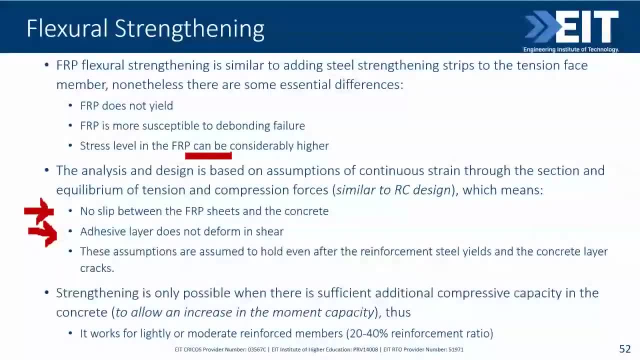 The easiest way- does not deform in shear, And this assumption is actually Will hold to even after the reinforcement steel yields. So in this case- I have to highlight this- We actually We have three materials here: We have FRP, We have concrete. 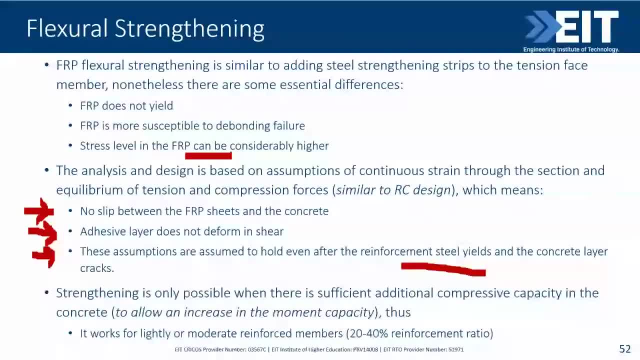 And steel Right And all together. This strengthening is only possible When there is a sufficient Additional compressive capacity in concrete. Because we have, The concrete must allow The increase in the moment capacity, Otherwise we wouldn't Do anything in this. 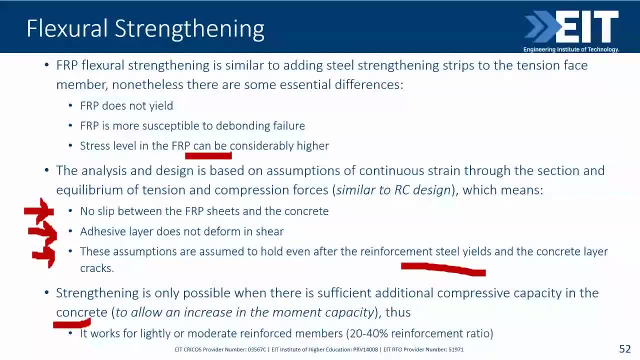 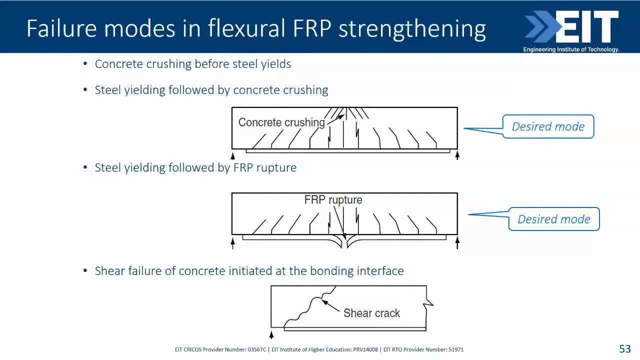 And this is possible With relatively low Reinforcement ratio. The failure modes: I will probably skip the We'll see. So the failure modes. The failure modes: We're looking at the flexural, Which is our most popular, The failure modes. 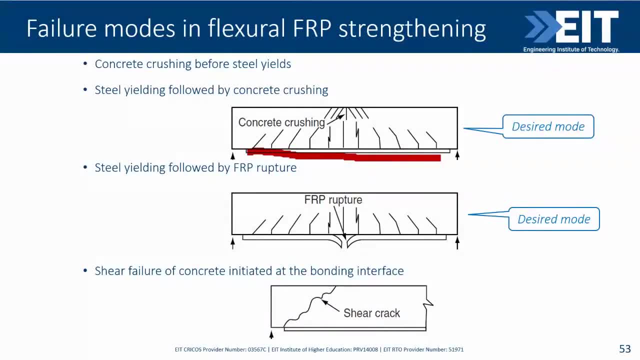 There's attached layer of FRP on the Concrete Steel, reinforced concrete, P Loaded and bending. So the modes are concrete crushing before steel yields. There's nothing to do With the Frp sheets- Steel yielding, But Frp sheets. 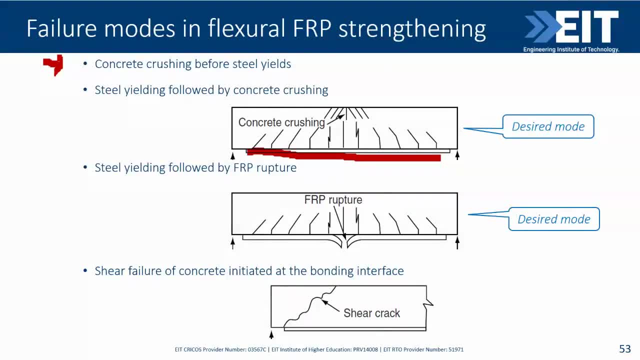 Changing The equilibrium In the procession. So the steel Yields, Followed by concrete crushing. That's what we're actually One of the preferred modes: A steel Yields Followed by Frp, Which Was actually 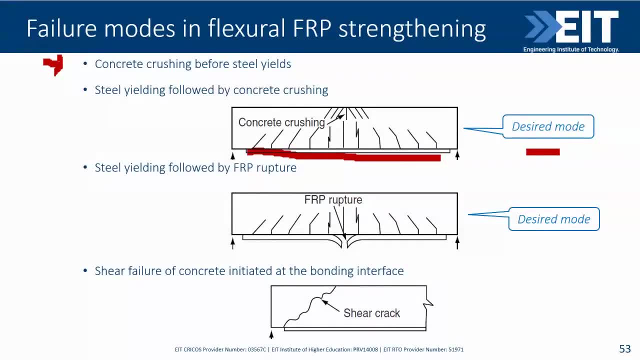 Preferred In the procession. So The steel Yields, Followed By Concrete Crushing. That's what we actually Considered. The third Mode, The shear failure Of Concrete Initiated At the 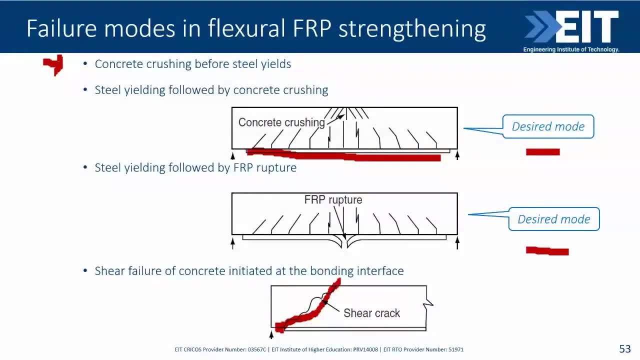 Bonding Surface. So It's a shape- Initiates Here And propagates Towards The Top- Another Failure Mode. Well, This Mode Become Important When We Design It. 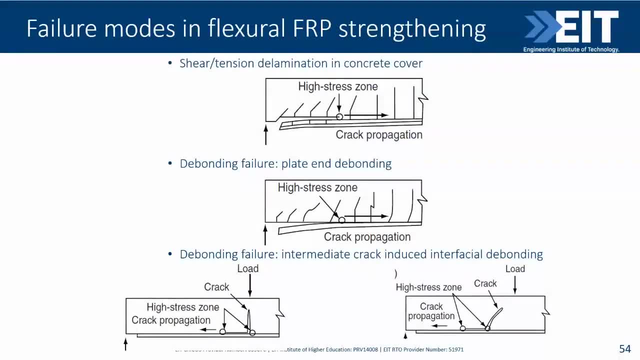 Starts At The Top And Propagates Towards The, Towards The Middle, The Bonding Failure. So It's Actually Again, It Starts In The Middle And 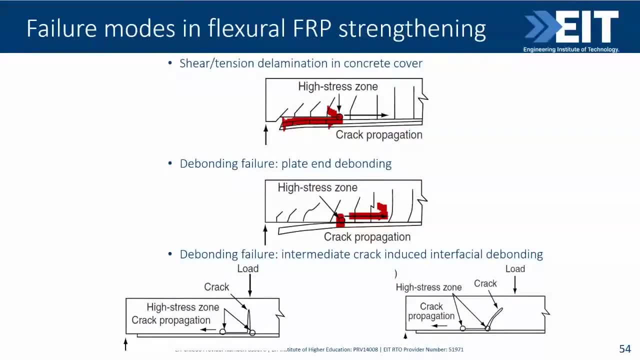 Then Propagates In This Point: So We Have The Crack Induced: Interfacial Bonding. So We Have The Crack Here, Starting At This Point. 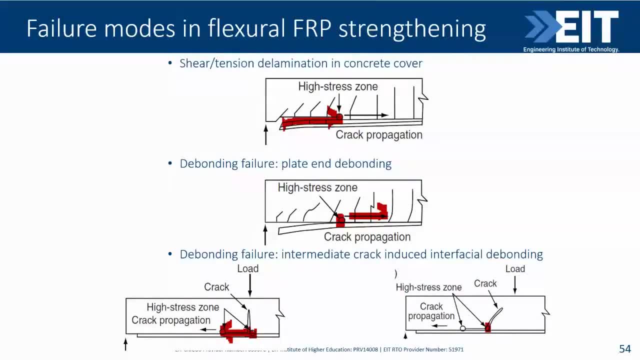 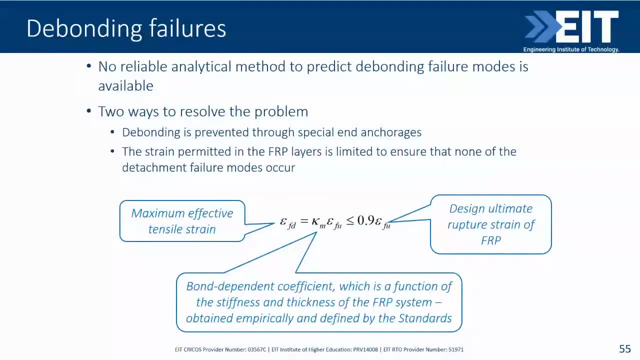 Which Actually Initiate The Crack, And It Will Propagate In The Middle And The Middle- And This Is A Very Important- To The End Of 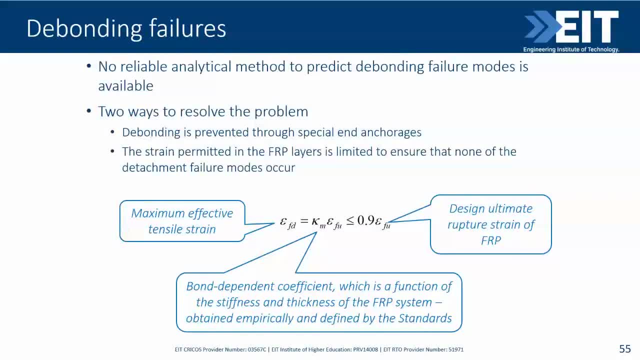 The Bonding. So We Have The End Of Bonding And The End Of The Bonding. So What Instead, Instead? The American Concrete Institution Guide. 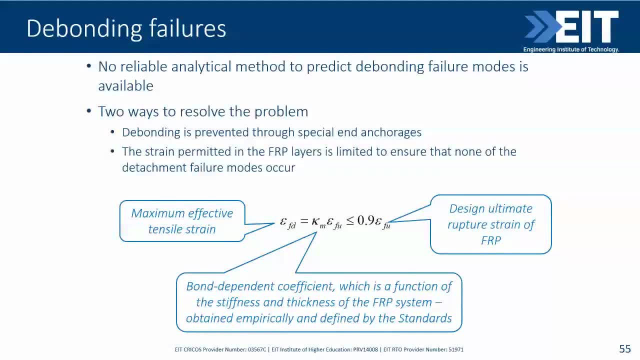 American Standard And Proposes Two Ways. So The Bonding Can Be Prevented Through Some Special End, Some Kind Of High Strength Bolts There I've. 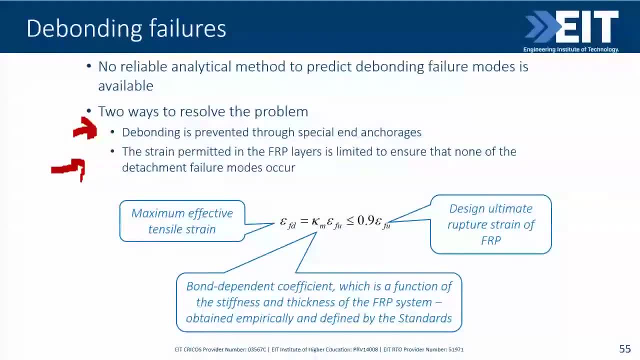 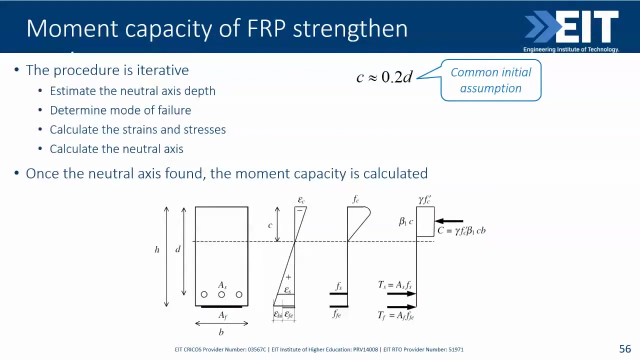 Seen These Designs Is Going Through To Prevent This. The Bonding And The Other Way Is In Design. So To Limit The Moment Capacity. So 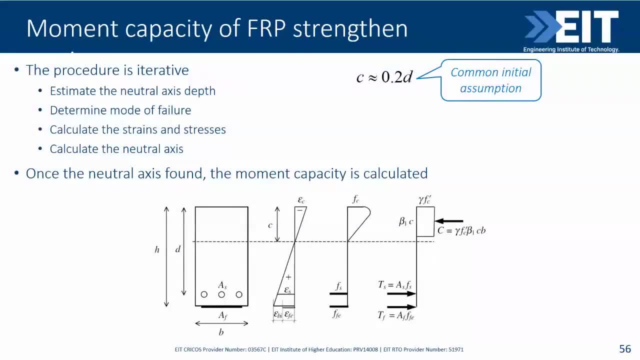 The Moment Capacity, The Nominal Moment Capacity Of For P, Strength And Cross Section. Yes, You Can Know The Similar Picture. Now We Have The. 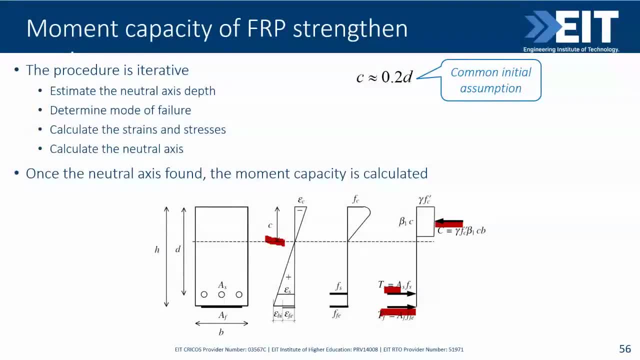 Compression. In This Pair, Which Are Two, Prefer One. I Mentioned Compressive Failure Of The Concrete. That's The More One, More Two: The Failure. 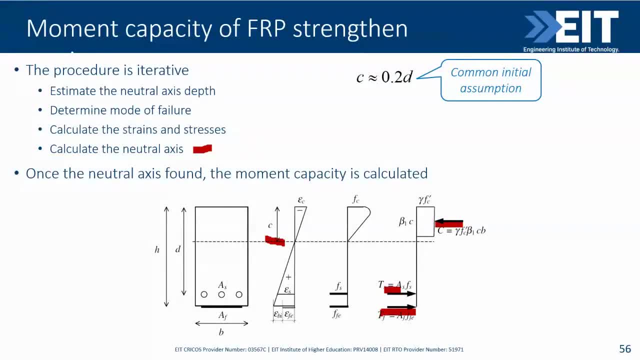 Of Frp Statling System, So Frp Layer Breaks. We Can Calculate The Moment Capacity Once We Found The Access, Avoid Showing You Any Expressions. 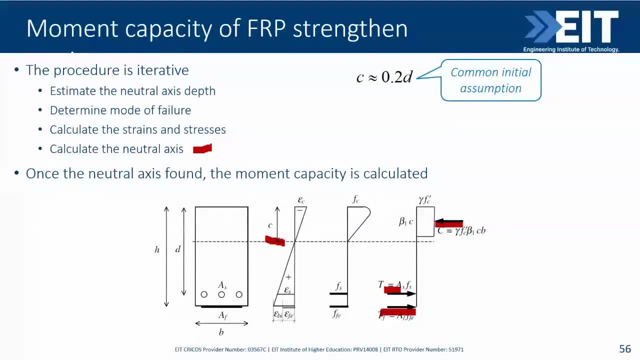 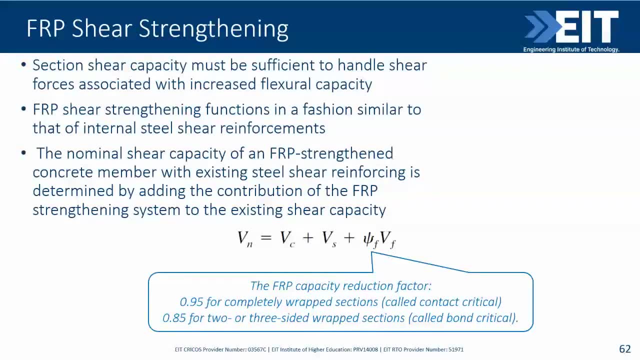 For This. It's Probably More Interesting For Practical Engineers. Who Wants To Do The Concrete, Steel And Strengthening Shades? Let's Go Faster From Here. 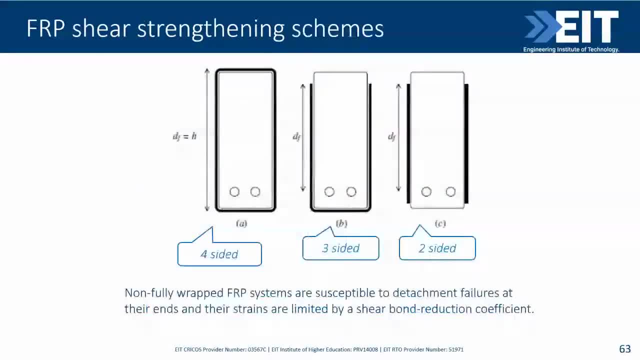 They All Have Different Design Factors And, Like We Said, It Can Be Done Two-sided, Three-sided Or Four-sided. The All Right. So In This, 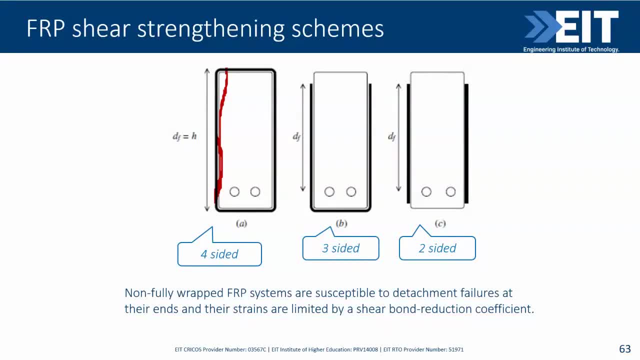 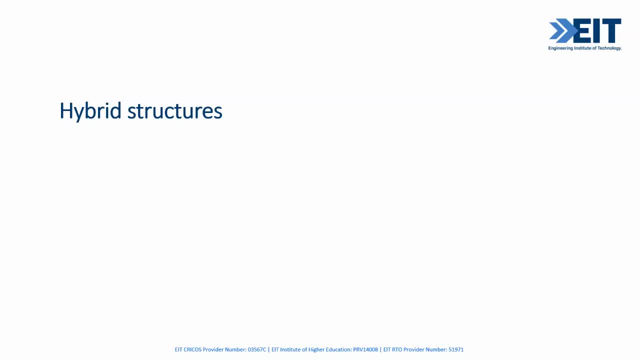 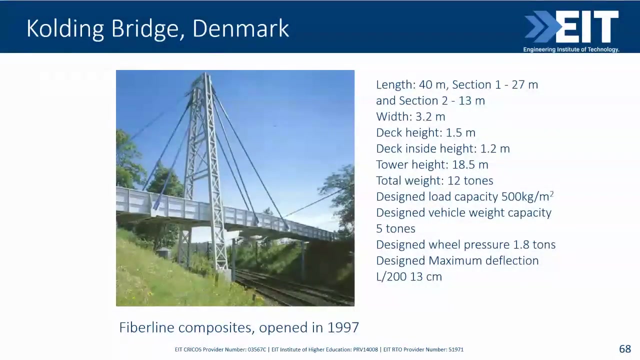 Case The, This Splice Will Provide Some Additional Shares. Wow, We Probably Running Definitely Out Of Time, But We Will So Keep Over. There Are. 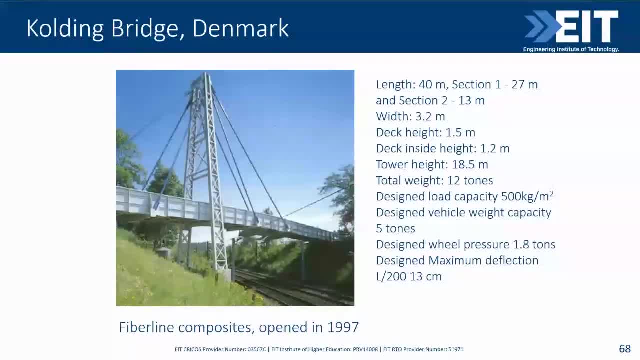 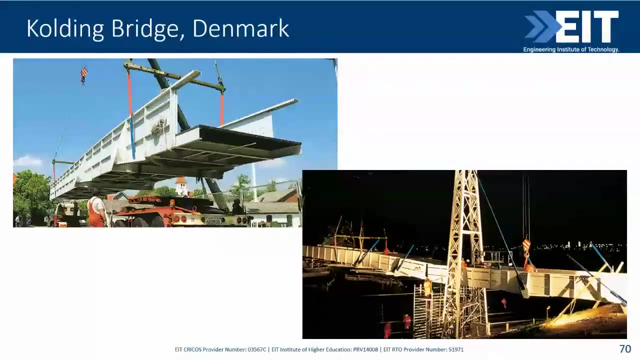 Fully. First Composite Bridge In Denmark, Built In Ninety Seven Fully Of Composites. So All Elements Are FFP. Easy Installation. Now We'll Skip Details. 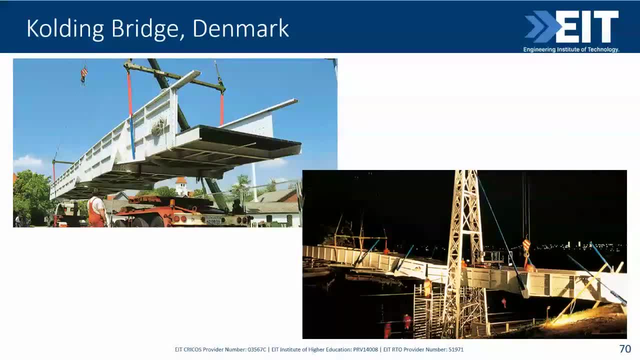 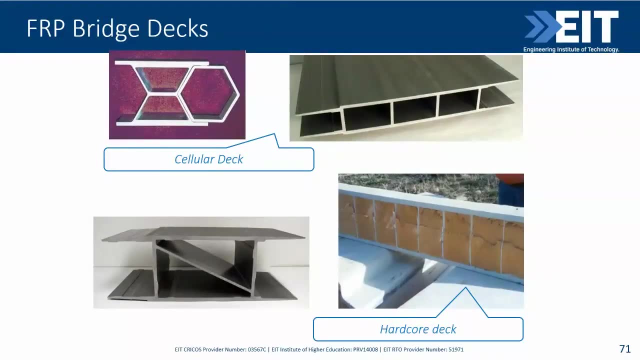 On This Way. They Have Many More Since Built Since Then. Right The FFP Bridge Decks Getting More Popular, Though It's Very Corrosion. 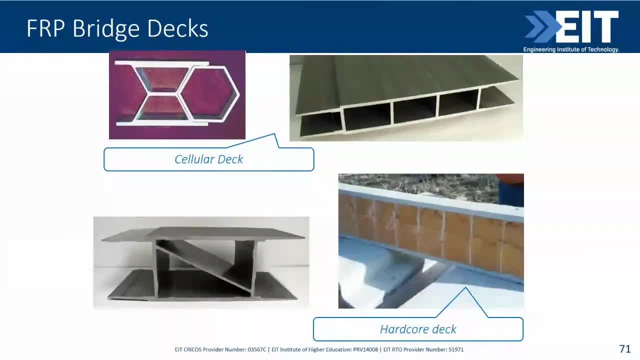 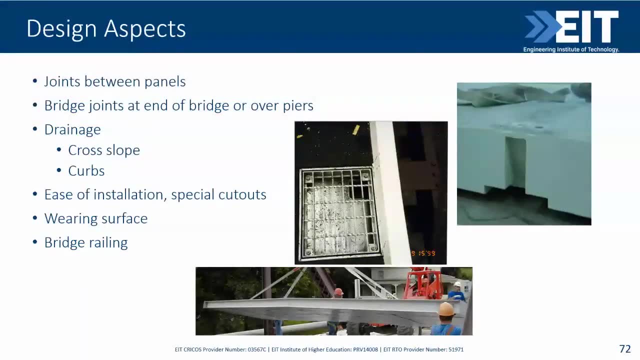 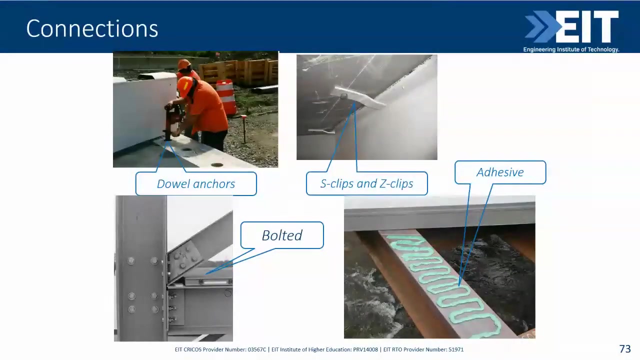 Resistance, All Different Elements Really Readily Produced In Different Countries. Today You Need To Be Consider The Connection. We Mentioned It Before And There A 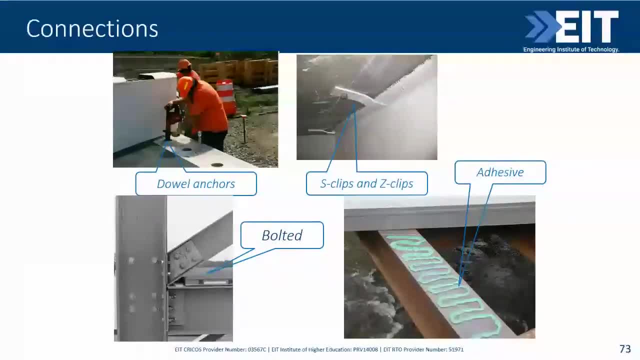 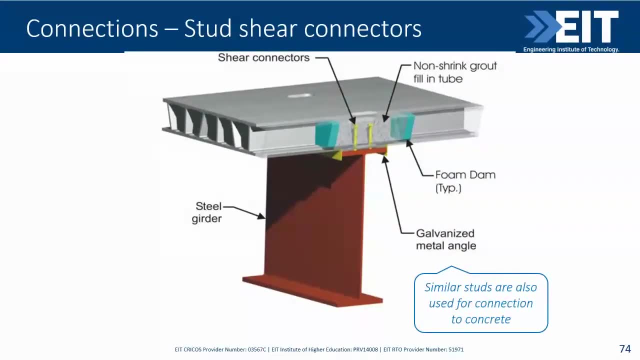 Couple Of More. The Connections Are Mostly Done Is Discussed Using Mechanical Devices And Adhesives, The FFP Deck. If Anyone Who Is Familiar. 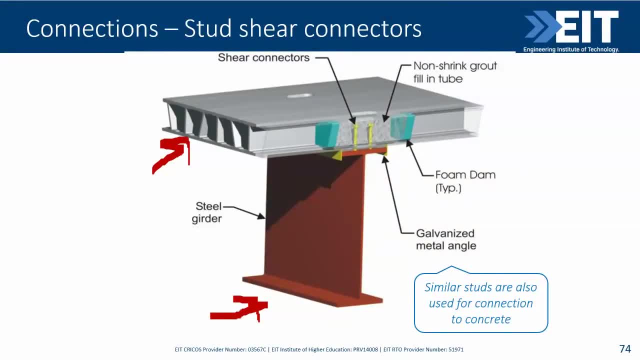 With Steel, Concrete Composite Construction, Which Is Steel And Concrete In This Arrangement They Are Actually. This Case Has A Concept. It Is Still Your. 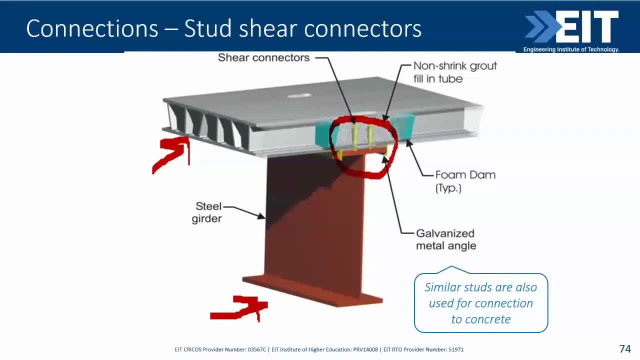 FFP Deck. But The Hybridization Of Concrete Floating And FFP Beams Is Also Becoming Popular. So Using FFP Beams On In Addition. 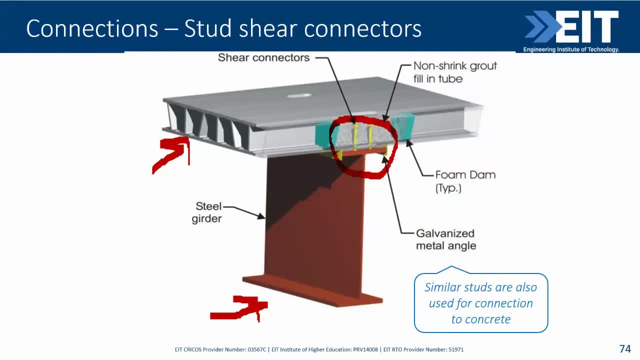 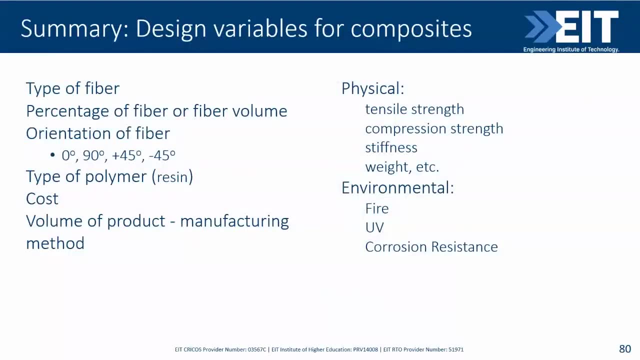 To FFP Reinforcement. So Here Already Did. Well, Let's Summarize All This. So When Designing In Composite Structure That Uses Composite Materials, You 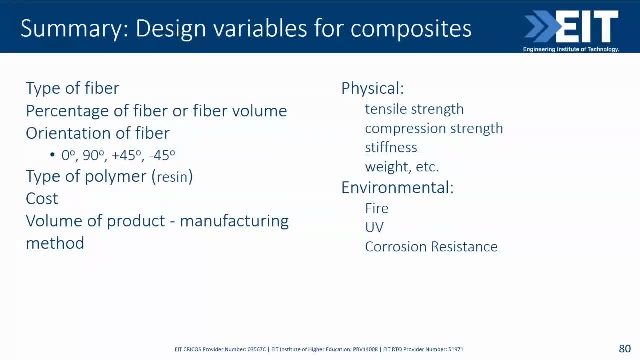 Have To Consider The Falling Parameters, So It Will Be Type, The Orientation. We Didn't Actually Look At The Different Ones, Only 0.. 90.. 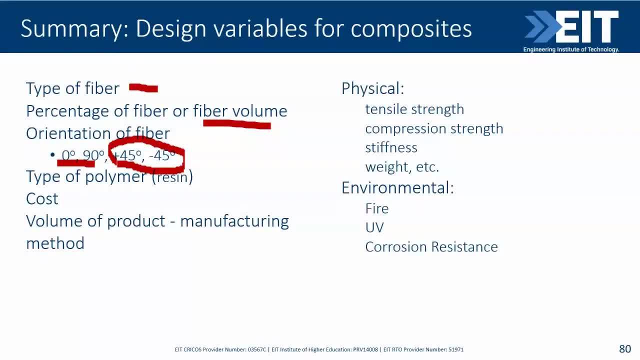 Degrees, So In Two Direction. But The Possibility Of Angle Plies Is Very Interesting Especially For Which We Said Was The Problem. So Type Of 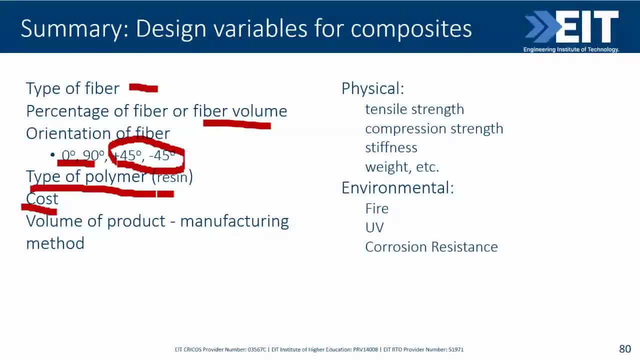 Polymers Resin, And That's The Another Consideration- The Cost Which Is Related The Resin, The Polymers Becoming Cheaper, So It Will. 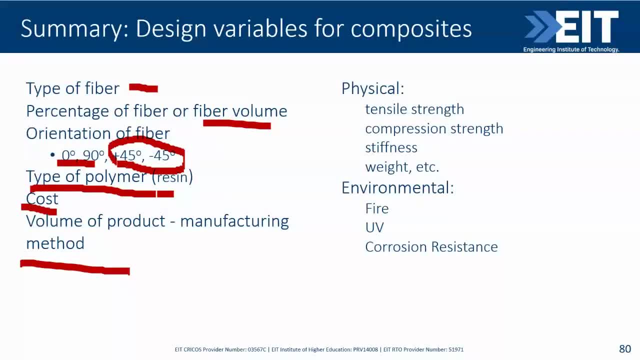 Lead To Optimization Of Required Physical Properties Such As The Silent Strength, Compressor Strength, Stiffness, Weight. So Environmental Influence Is Also Important Here. So 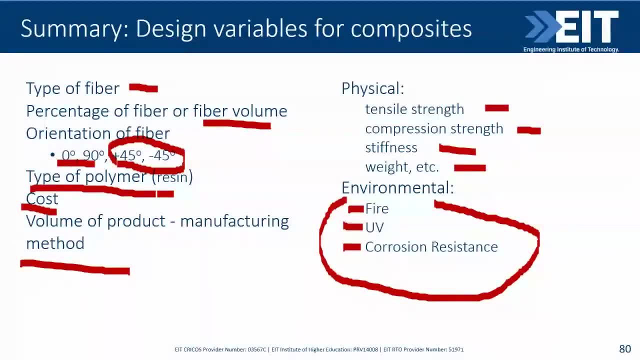 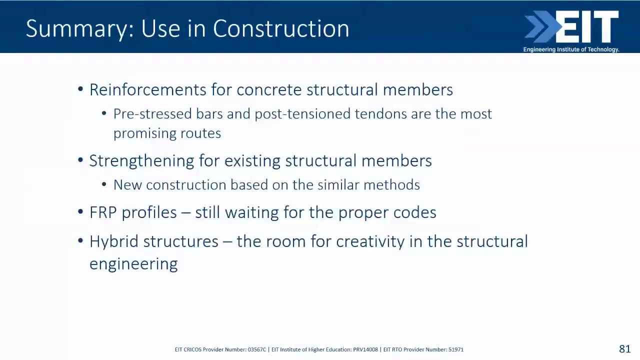 We Will Improve Mental Resistance, As We Need To Take This Into Account, Because These Are The Behavior Of Composites And This Aspect Is Different. 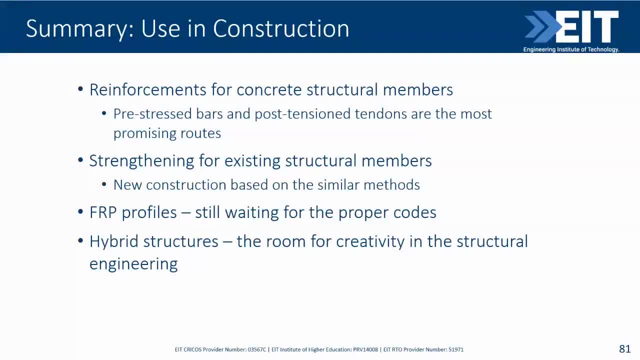 From The Conventional Structural Materials. Right- And To Sound This To Convene Here- Is That The The Fiber Enforced Composite Materials Are Gaining. 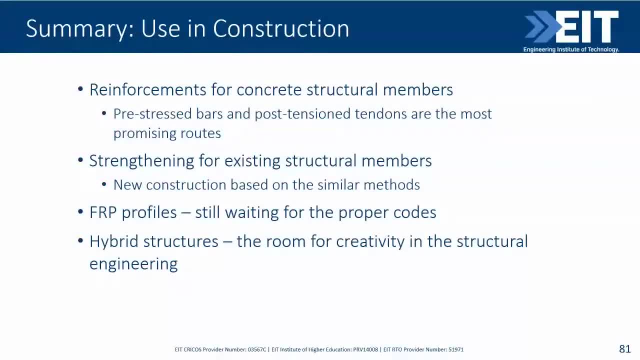 Strong Popularity In Audience Over Overall, Everywhere Now Actually Becoming A Net Of Choice In Structural. More Potential Is In The Pre-stressed And Post-tension. 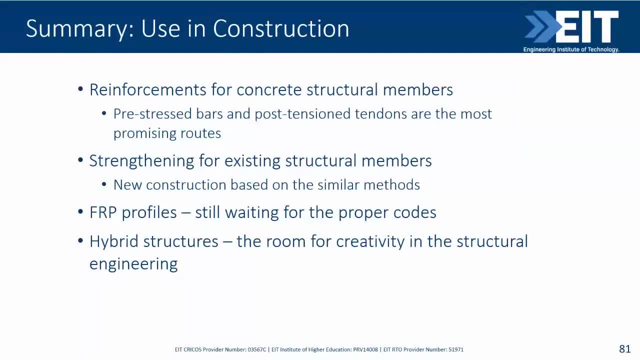 Elements Of Pre-stressed Parts And Post-tension Tendence, And The Other Aspect Is This Is Quite Well Developed. Part Of This Is The Design. 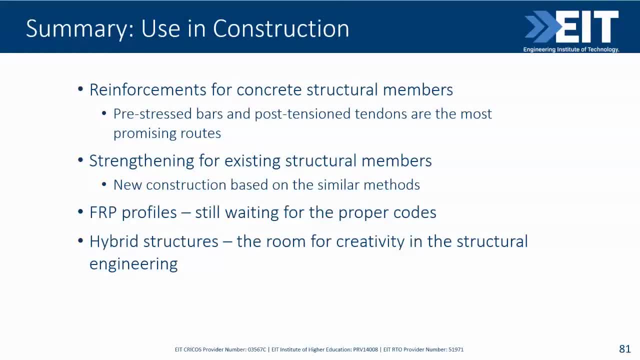 Of New Structures. Another Point I Would Like To Highlight Here, It's About FFP Profiles, The Structural Members Made Of FFP, While They Still 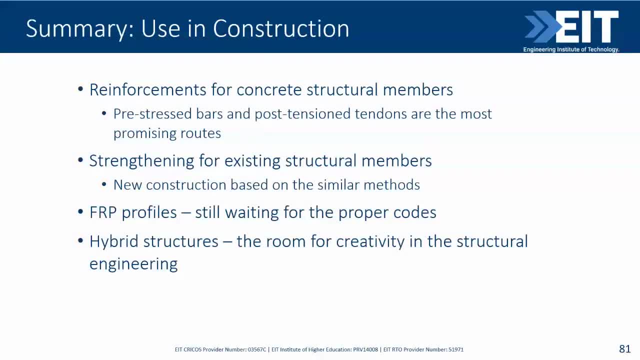 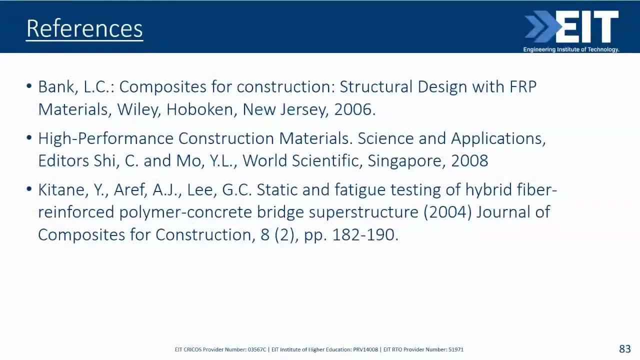 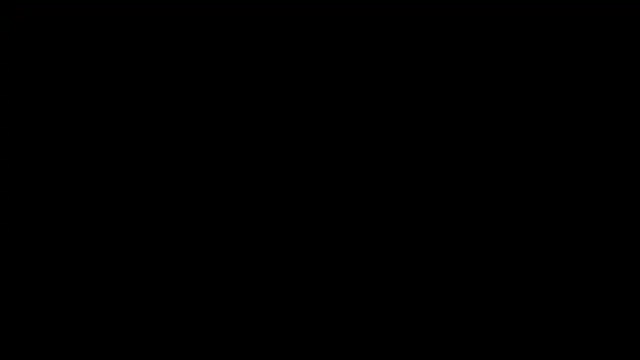 Acquire According To The Structural Right. So Well, It Is All I Have For Today. There's Some Reference List. Quite A Lot Of References Understand. 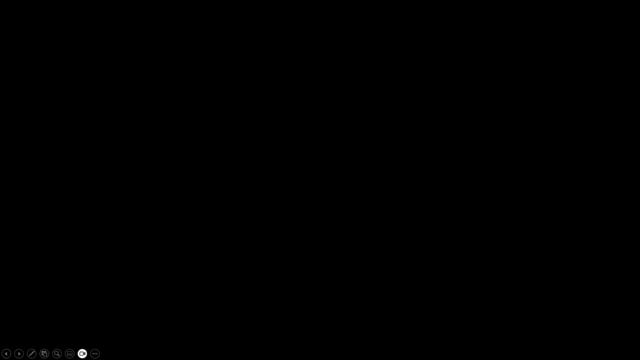 And They Didn't Bring Reference For The Profiles. So, Dr Eager, I Think We Have One Question Here In The Chat. He Is Asking If 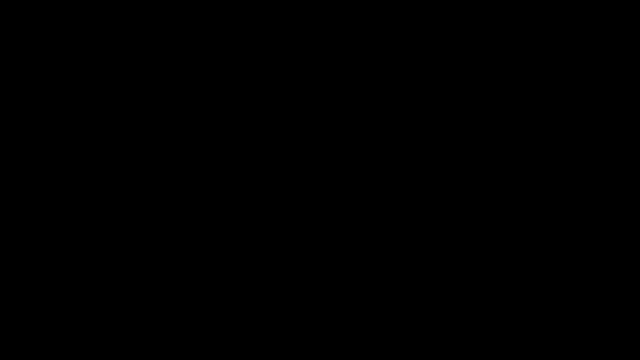 Is It Better For Fibers To Be Randomly Orientated Or Oriented, To Be Oriented In The Same Direction As The Bending Axis To 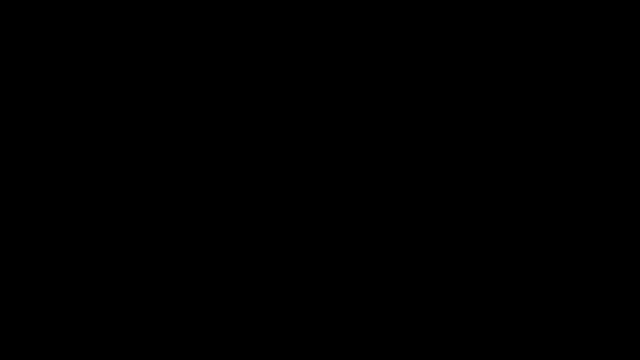 Achieve Strength, Ductility And Resistance To Crack Formation. Well, The Optimum Design Can Be Achieved When With Some Preferred, In Some, In Some. 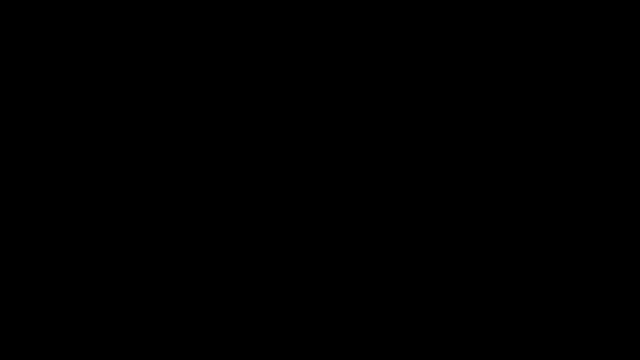 Cases. It Is Also Popular The Particle Reinforced Concrete Today Or Chop. So It's Just General Improving Of The Effective Property, That's The There. 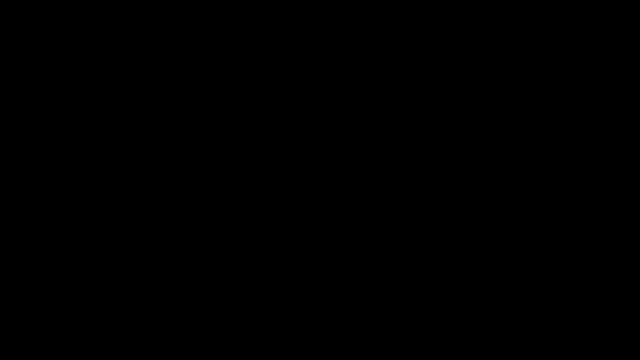 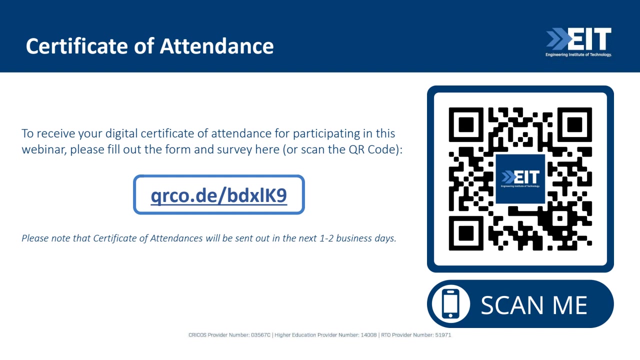 Is And Target Specific Law, So We Can Be More Specific, And When We're More Specific We Can Save. Okay, Thank You So Much For. 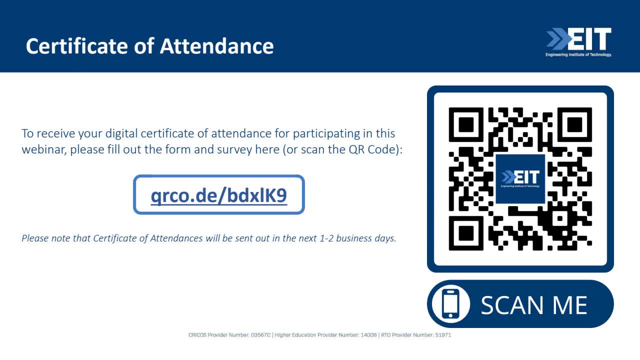 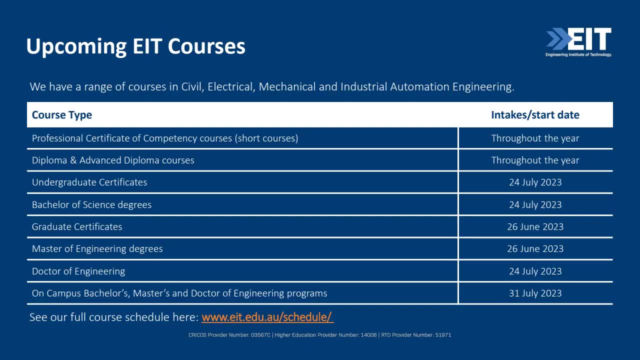 That There Is Another, One Another And Other Than Matrix Of Fiber. So It's Two Questions Or One I Missed Here. It's This, It's. 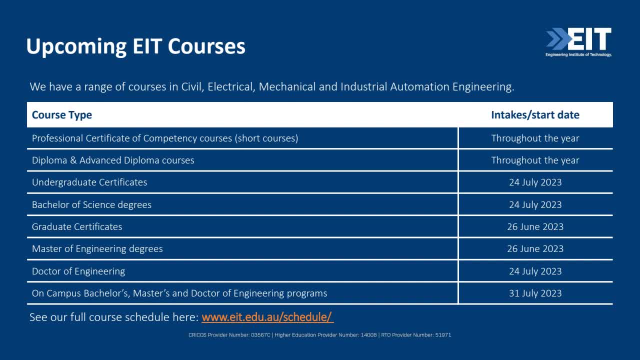 The Same. Can You Repeat, Please? Sorry, Someone Asked What Are Metrics And Fiber At That. That's Because Students Components Of A Composite Material. We 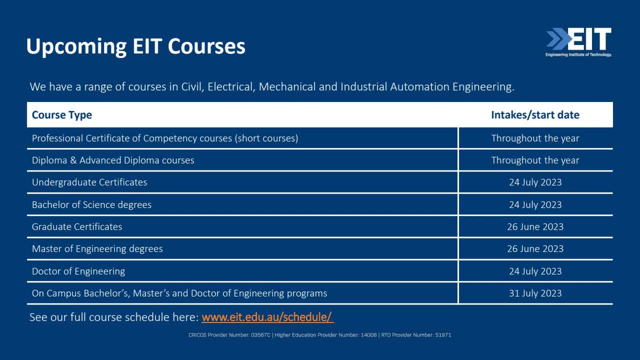 Using A Fiber Incorporated Into Metrics To Receive The Composite Right And Then This Composite Material For Creation Of Structural Components. So Bridges It Is At. 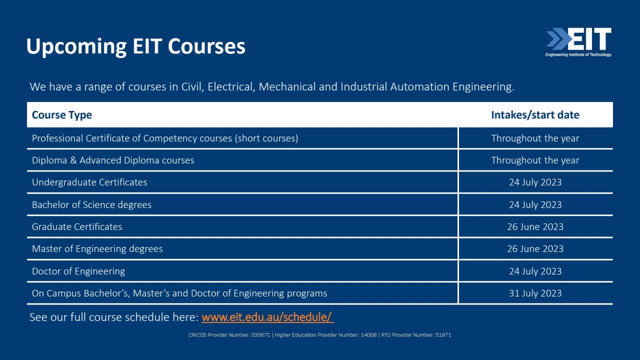 The Moment It Is Mostly Decking For Structural Beams, For Pedestrian Bridges, For Other, For Light Bridges Is The So The Beams Are. 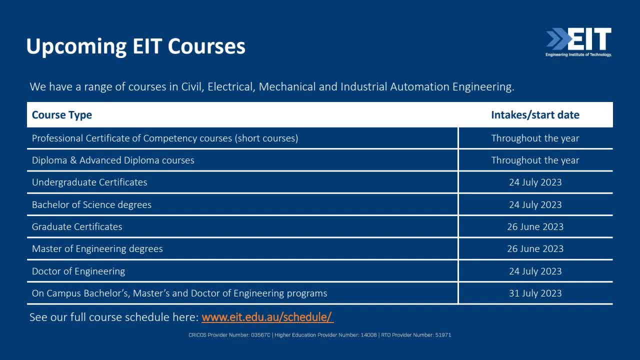 Fully Made Of Structural Composites: Frp. All Right, Thank You So Much. I'm Afraid The Question That. That's The Way I Understood This. 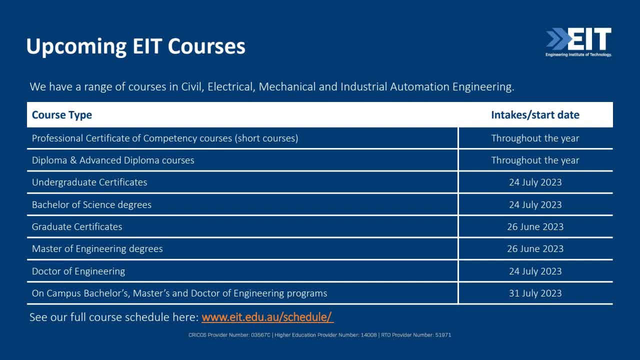 Question: Okay, So We're Going To the next Part Of Our On The Stat Of Our behave. What Do You Think That We Have? An Important 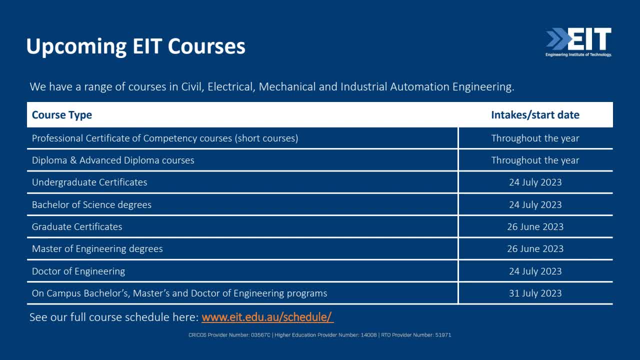 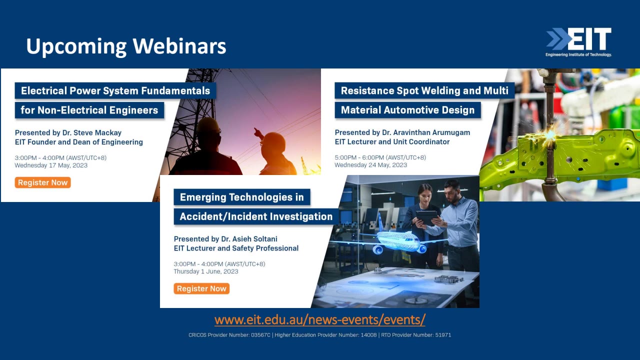 Beyond In The Future Of If A July. you can visit our website, wwweiteduau slash schedule so that you can see all the list of upcoming courses that we have, And these are also our upcoming webinars. You can visit our 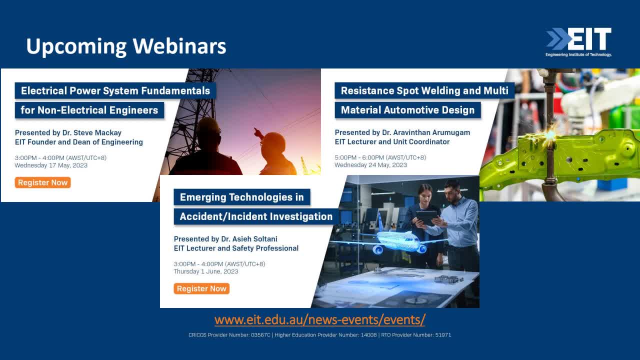 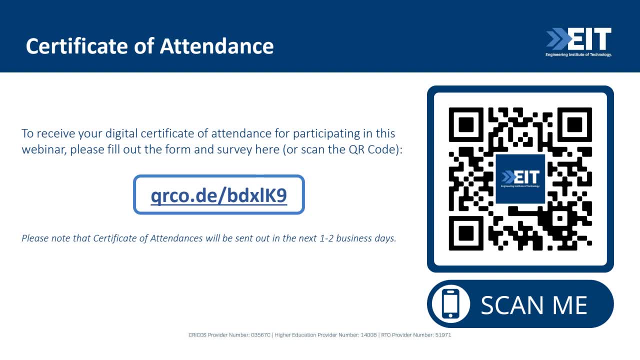 events page on our website to look at our upcoming webinars, And in two to four days we will be sending out the video recording of this particular webinar. And for those who'd like to use the QR code, kindly scan the QR code that you can see on your screen right now. 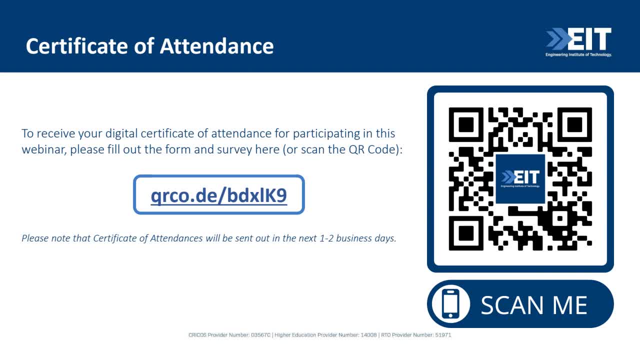 to request for your certificates And for those who'd like to use the link, copy and paste the link or click on the link that I sent on. I mean in our chat box right now And again. for further questions, inquiries and concerns, please send an email to. 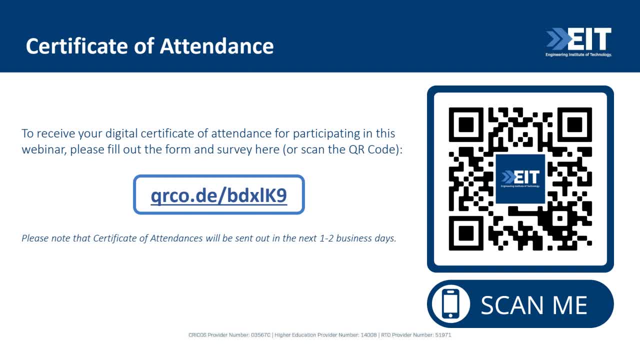 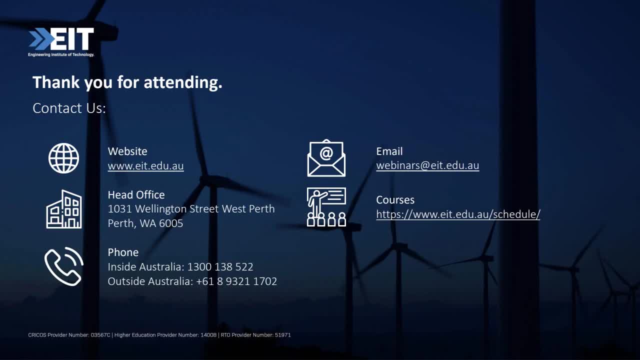 webinars at eiteduau. I know that you have a lot of questions to ask And we are very grateful for Dr Igor that he covered everything in this webinar And I do hope that everyone learned a lot and a lot of you are saying thank you, You are very much welcome. 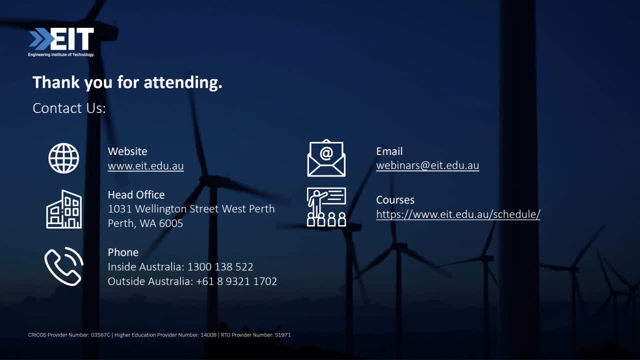 And thank you also for participating. And here are our contact information. You can see our website link on the slide And we also have our phone numbers and our email address that are direct to the webinar channels. So if you send an email to our webinars inbox, then 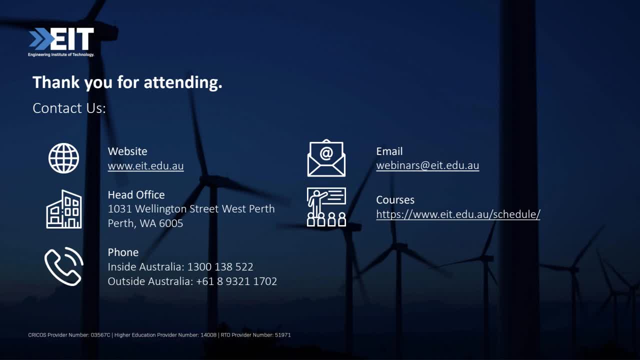 we would be more than happy to assist you as well. All right, So thank you. Thank you so much everyone. Thank you so much, Dr Igor. That was a very informative session, And I can see that every one of them also enjoyed it and find it interesting. So again we will be.